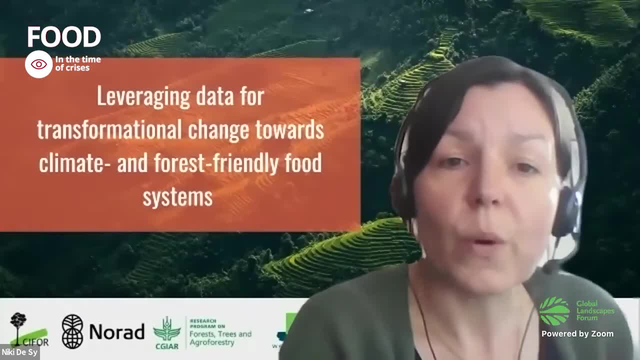 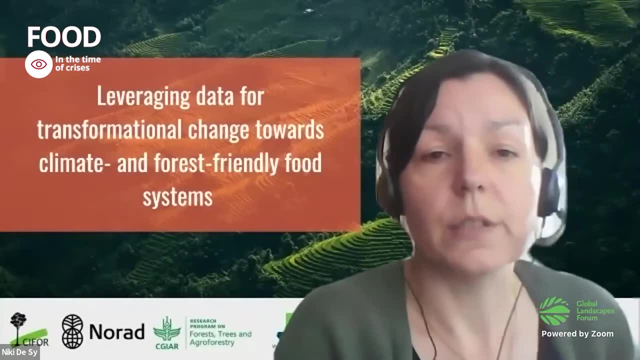 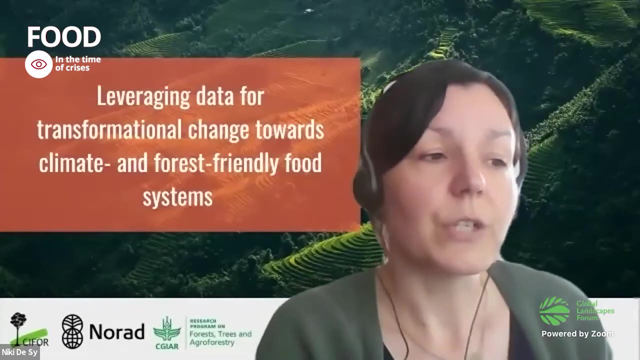 Of course we would also like to hear from you Your questions and observations. So there is. you can always post your questions to the Wolva app in the Q&A section And or my colleague Asrit Boss will be moderating those questions and we'll try to answer at least some of those. 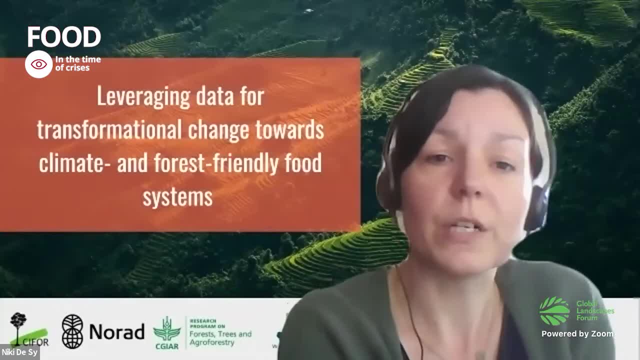 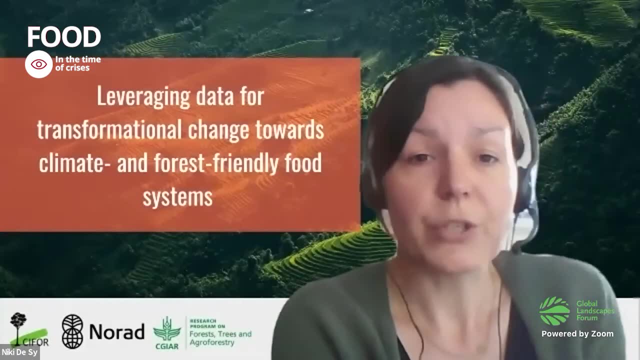 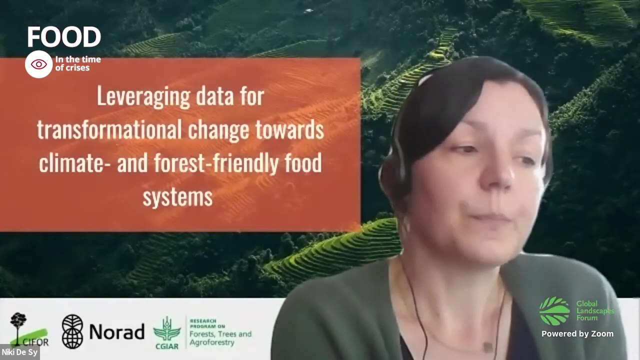 So you can post throughout the session. please post your questions there. There's also Spanish audio translation available through the Interactio app. We have shared some instructions in the chat of the Wolva app, So if you're interested in that, I won't do a very lengthy introduction of all the speakers. 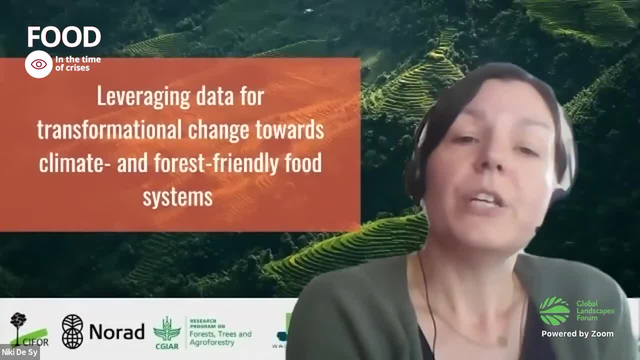 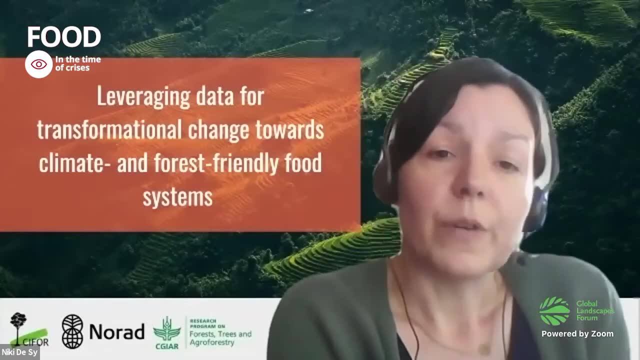 You will get to know them better throughout the session. Their information is also available in the conference website, And we will also share a link in the chat where you can find more information. So let's get started with our first topic of today, on sustainable food systems. 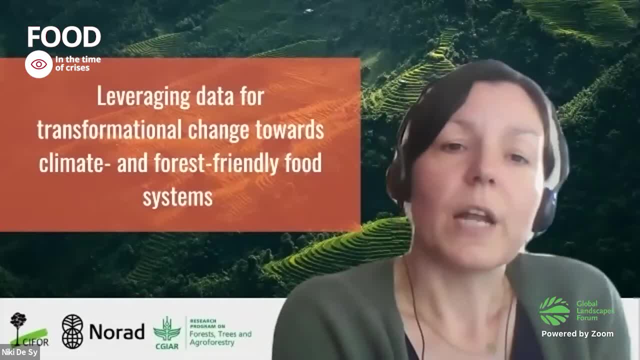 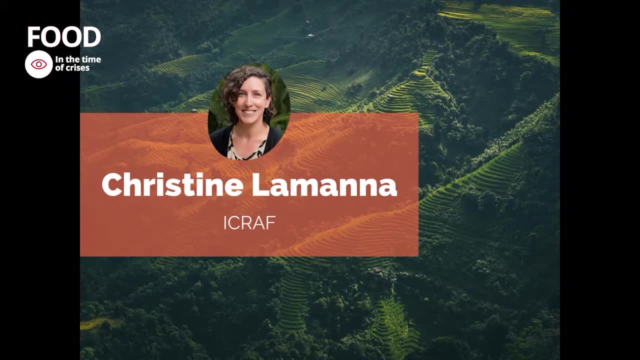 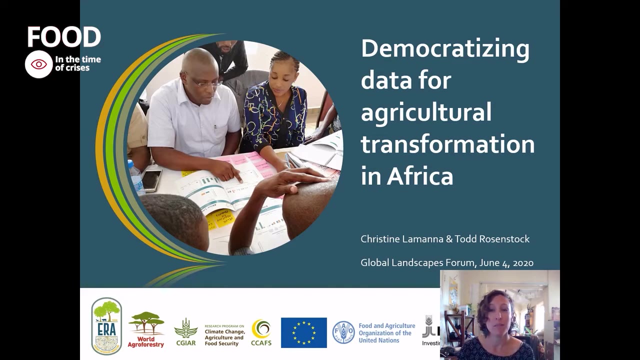 More specifically, the democratization of data for an agricultural transformation. So we can start the first video now. Hi, my name is Christine Lamona and I'm a climate change scientist at World Agroforestry, based in Nairobi, Kenya, And I'm going to be talking a bit about an initiative that's led by Todd Rosenstock and funded by these donors that you see at the bottom of the slide. 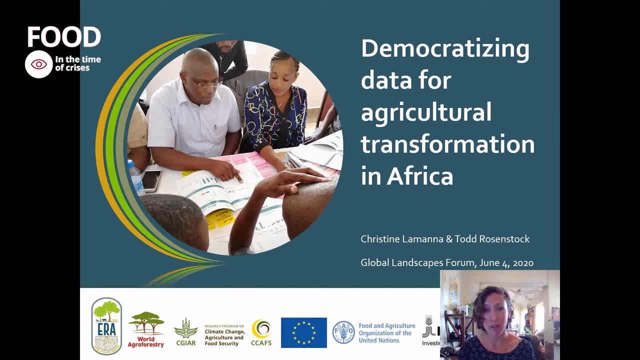 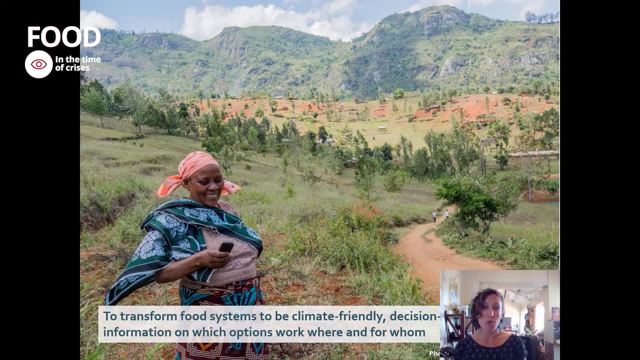 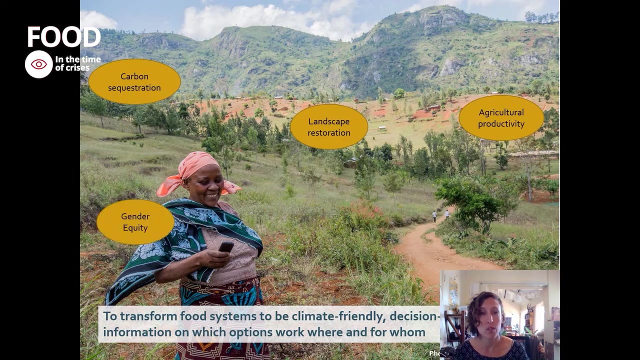 On democratizing data for agricultural transformation in Africa. So we're talking today about transforming food systems to become more climate friendly, But in order to do that, decision makers need information on which options work, where and for whom. This is especially true for thinking about more than just agricultural productivity, but also looking for outcomes: landscape restoration, carbon sequestration, gender equity, access to information and services, or even biodiversity conservation. 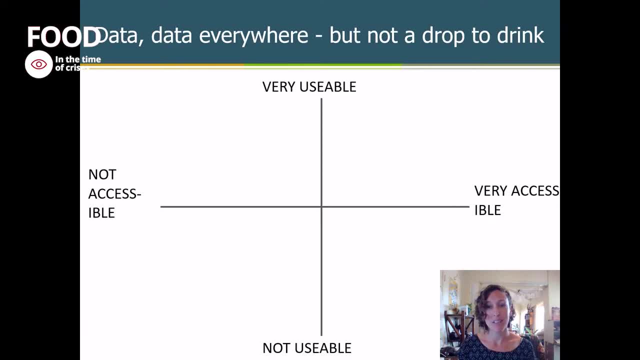 So where can this information come from? Scientists are really good at creating data, lots of data, But when we think about whether that information they create is accessible or not, usable or not, what we seem to find is that journal articles, which are the sort of bread and butter of scientific careers, are really not accessible at all. They're often behind paywalls. Raw data tends to be open access, But then you need all the technical skills and the computing power to turn that data into information, And the data aggregators and document repositories don't necessarily do all that much better. 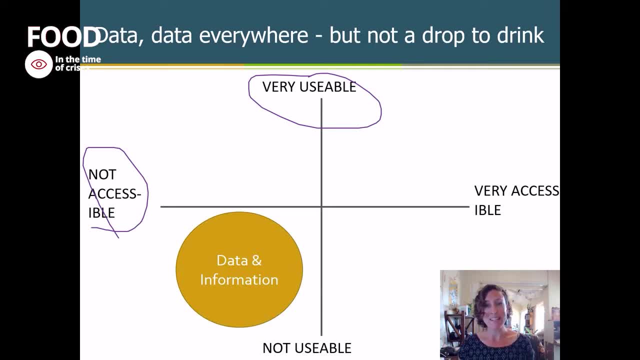 So what we have is a huge amount of data information, but it's sitting here where it's not accessible and not usable by the decision makers, policymakers, community leaders, NGOs and other people that can actually use it. So how do we move that data information from this quadrant to this one? 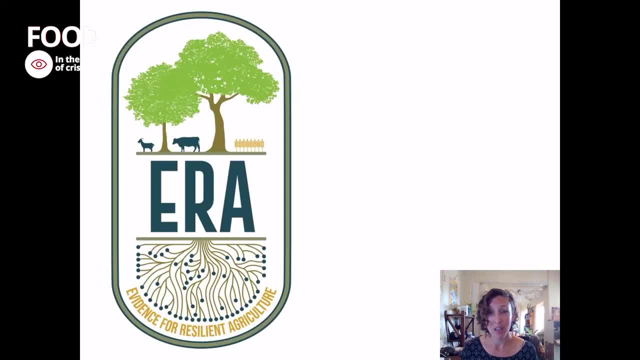 Where it's actually working for the people who could use it. And that was really the impetus for us to develop ERA, or Evidence for Resilient Agriculture. Now, this is a systematic review of the ability of agricultural technologies to deliver on productivity, resilience and mitigation outcomes, to allow evidence-based decision making for very diverse users. 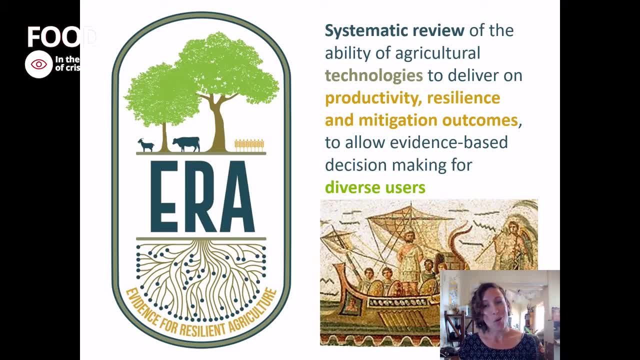 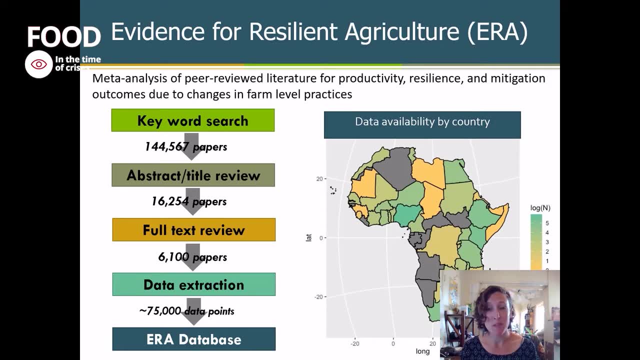 And developing. it was a bit of an odyssey, And so in the next minute or two I'll take you on that odyssey. So it's a systematic review, which means we searched the peer-reviewed literature for keywords that we thought were important for agricultural transformation and climate change adaptation and mitigation. 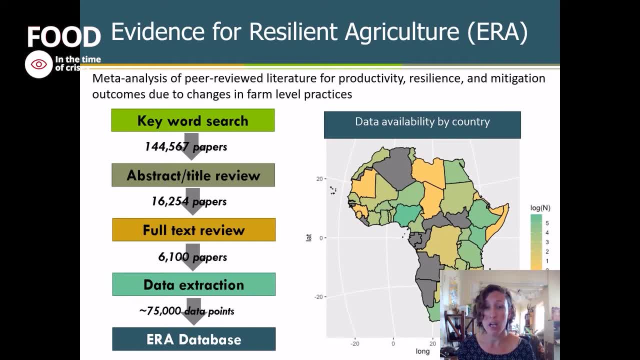 After lots of screening and criteria, we ended up with a pool of over 6,000 papers that we've worked on extracting data from. It's over 1,400 papers in Africa specifically, and over 75,000 data points and counting. 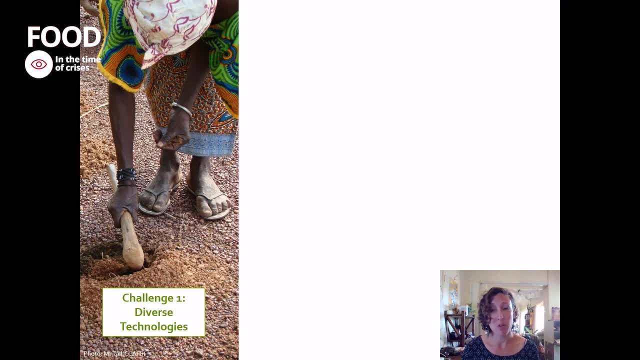 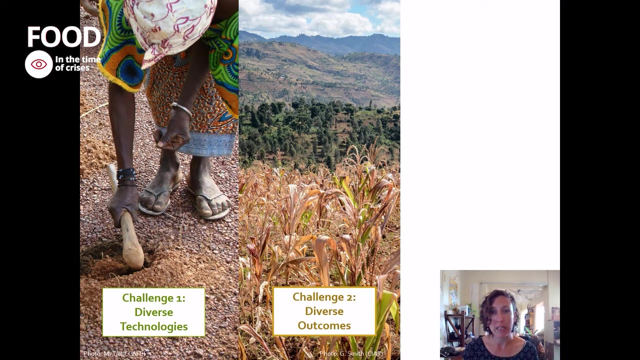 There were some challenges to overcome in order to go from old to new. We were looking at all this raw data into usable information, and one was that there's lots of technologies that can be adaptive or transformative in Africa. We're also looking for diverse outcomes, so not just agricultural yield, but income, labor, soil, carbon erosion, runoff, you name it. 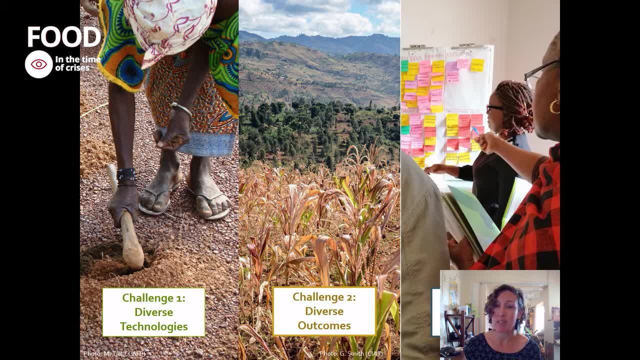 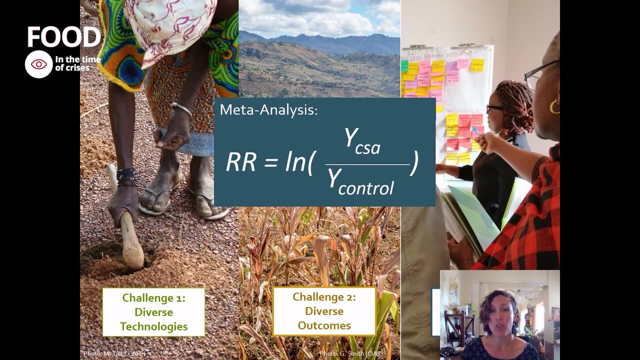 And we also have very diverse, different users who might be thinking at a community scale, or they might be thinking at national planning scales. So we needed a way to combine different technologies, different outcomes, And what we came up with- besides the ontology for all of these things- was also using meta-analysis. 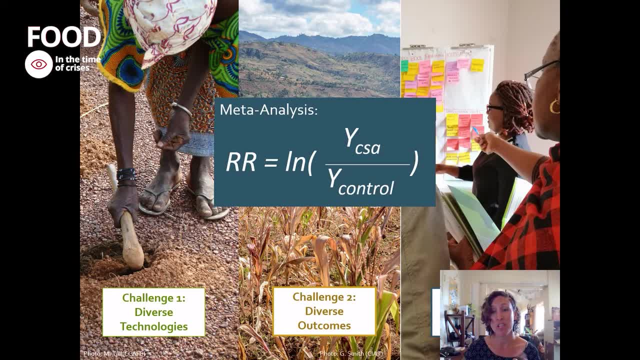 So, essentially, what we're doing is looking at the ratio of the outcome, whether it's yield or income or anything else, of the improved practice over the control, And that lets us lump and split outcomes for different technologies, crops, outcomes and so on, whatever way the user wants. 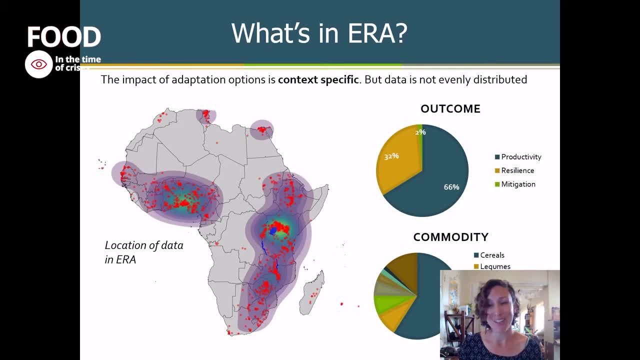 Well, if we look under the hood, what you're looking at here is a map of Africa and Egypt. The red dot is the location of a study in the database. You can see some hotspots here in East Africa and also in Nigeria. 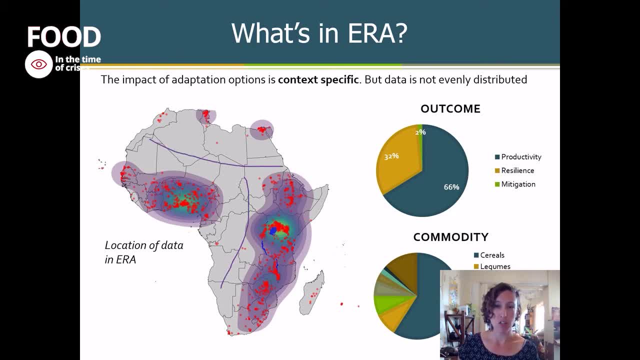 But then we have these big data deserts where there's very little information at all. When we look at outcomes, it's also not evenly distributed. The majority of our data is actually on productivity outcomes, like yield or income, and much less is on adaptation outcomes and very little on mitigation. 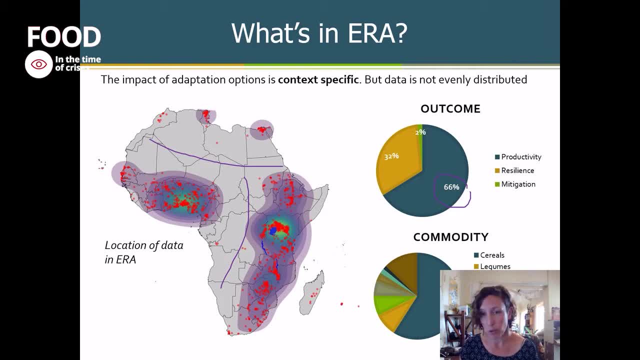 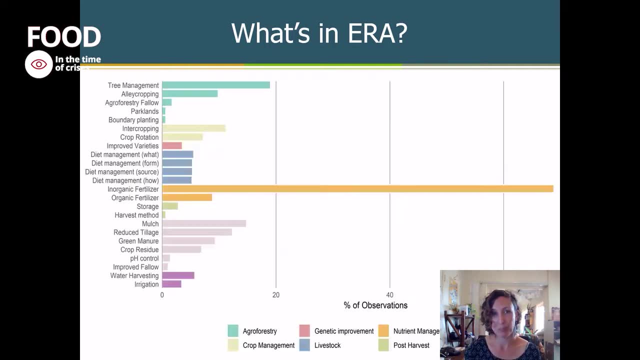 For commodities, the majority is on cereals like maize, millet, sorghum and wine, But there's still some information on legumes, vegetables, livestock and so on. If we look at technologies, so here we're looking at a list of different technologies and the percentage of our data that that technology makes up. 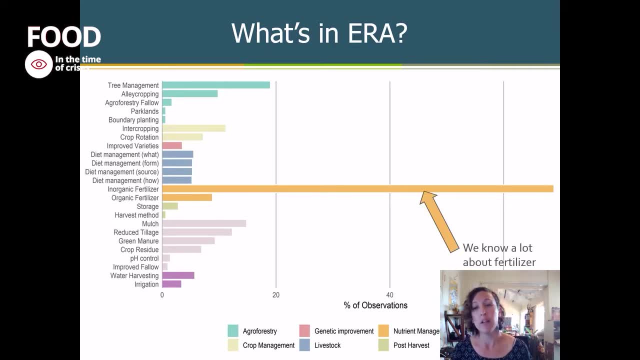 And the first thing that pops out is: we know a lot about fertilizer. This, essentially, has been over-studied in Africa for a very long time. But even these technologies like diet management for livestock or diversification practices, including agroforestry- 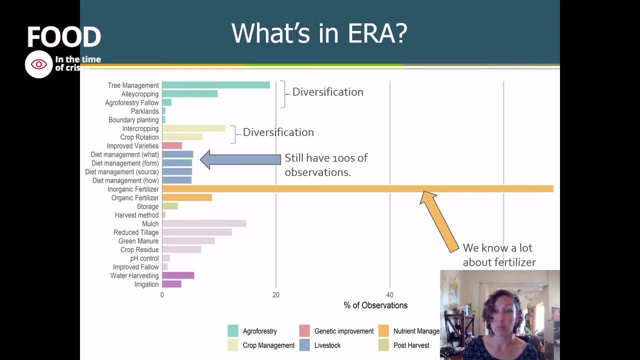 we still have hundreds of observations of these technologies that could be really important for agricultural transformation, And what's cool is that 52% of the data is actually on practices done in combination with others, So not just the practice alone, but also how it interacts with other technologies or practices in bundles. 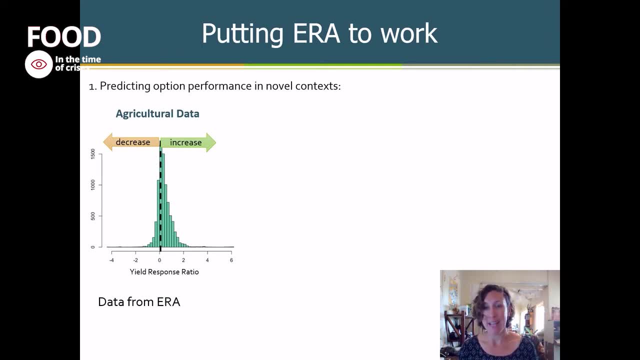 So that's what's in there. So now, how do we put it to work to actually answer questions that people have? One of the questions we've been working on is how do we predict how these options will perform in places where they've never been tried? 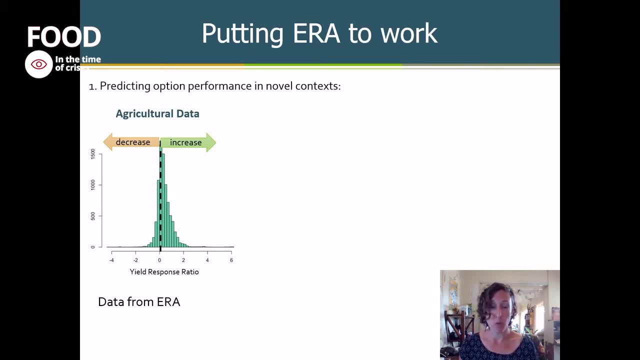 So in novel contexts. So we can look at this diverse data that we have with those spatial locations and correlate that performance, whether it's a positive or a negative outcome, with the context. So the climate, the soils, the agroecology, even the social context. 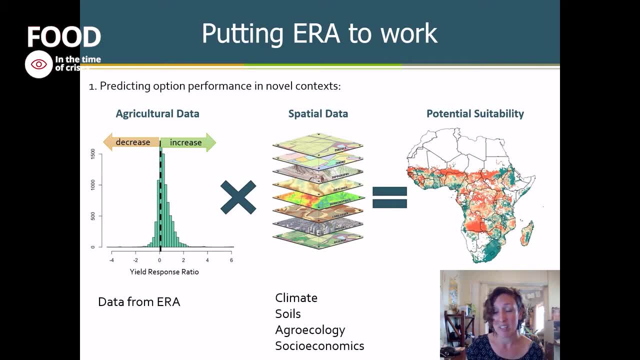 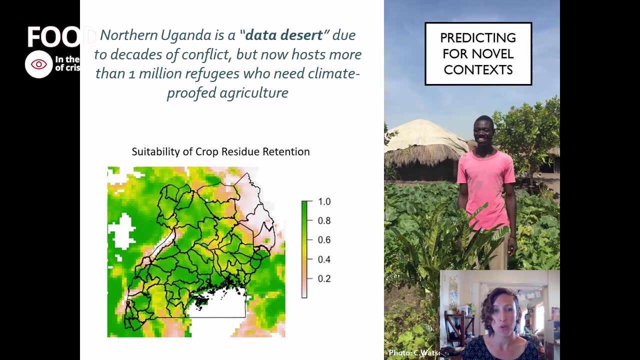 And that lets us predict the potential suitability of a technology in a place that's never been tried. This is especially important in those data deserts we were mentioning earlier, One example being northern Uganda, where, because of conflict, they don't have any primary research that's been done on the ground in the last few decades. 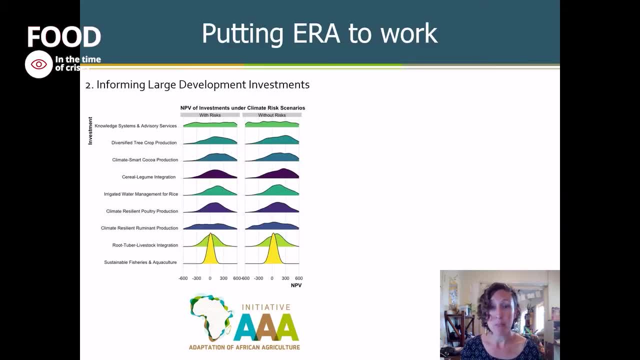 We've also been working on informing large scale development investments, using data to look at how the different potential investment packages might perform both with and without climate risks, And this has been done with the World Bank, which is one of the five countries now in West Africa. 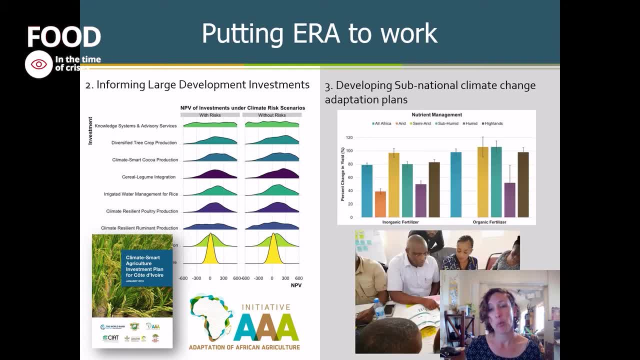 And we've also been working at subnational scale here in Kenya, helping decision makers in the counties look at their specific context with data to make climate adaptation plans for the agriculture sector, And Veronica and Dettu will tell you a bit more about this in a minute. 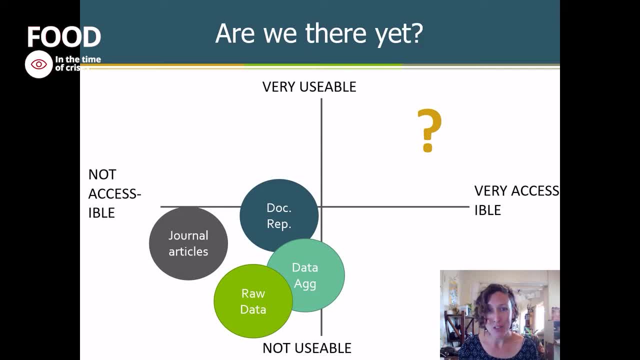 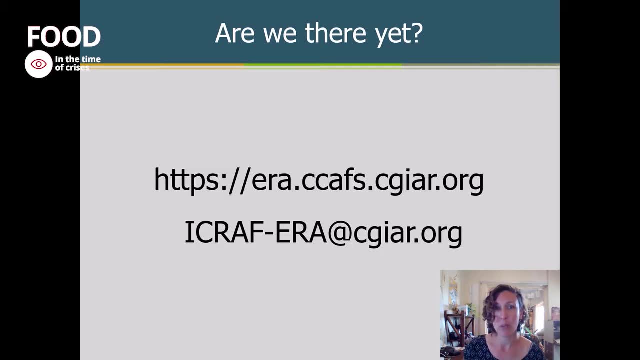 So are we there yet? Have we moved all this information over into the usable and accessible category? Well, probably not, but hopefully we've made some progress and we'd like you to see for yourselves. So you can go to the website, check it out, play with the data. 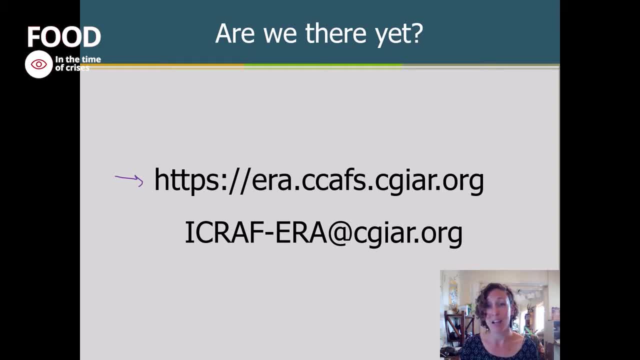 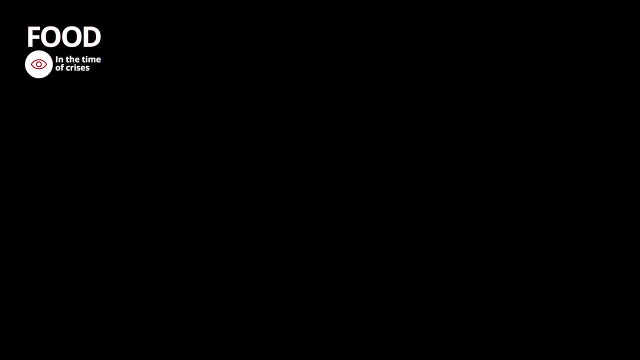 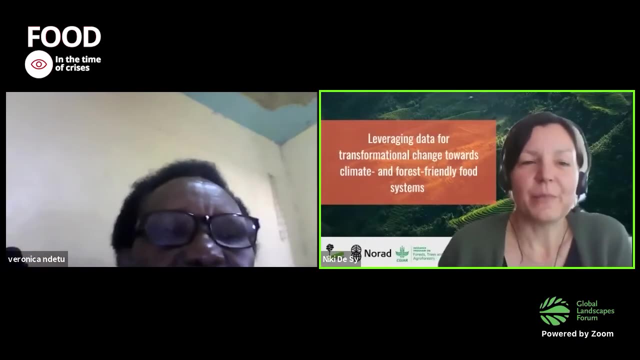 There's visualizations and a lot of things to look at, And please give us your feedback, because the database only works if it's working for you. So thanks so much. Let me unmute myself. Thank you very much, Christine. So I want to invite now Veronica and Dettu. 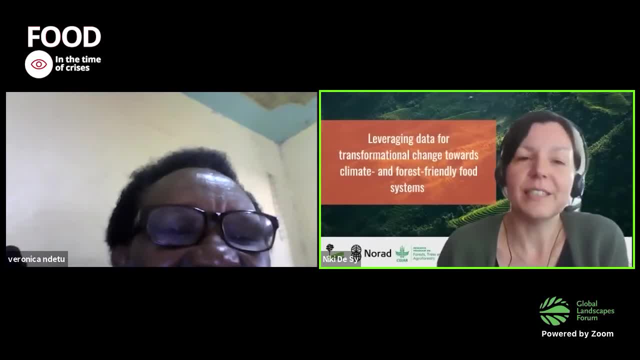 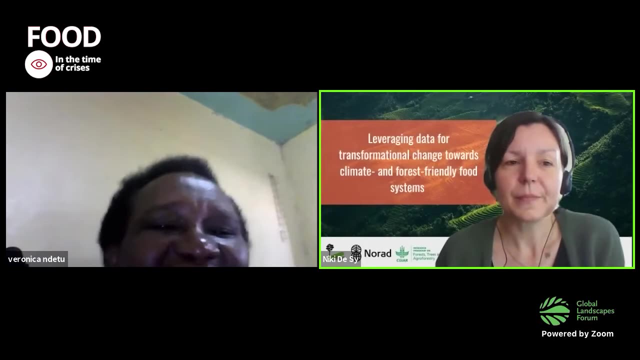 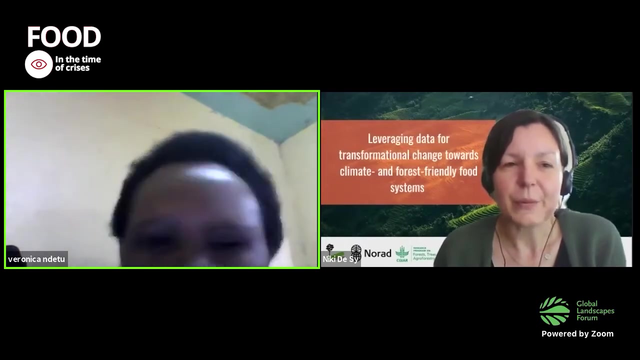 head of the climate change unit of the Ministry of Agriculture in Kenya. Veronica, please tell us a little bit about yourself, And can you tell us how and with what aim you use this ERA database or tools in Kenya? Thank you, And good afternoon everybody. 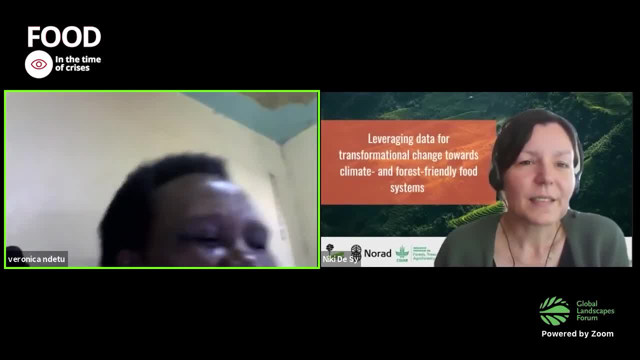 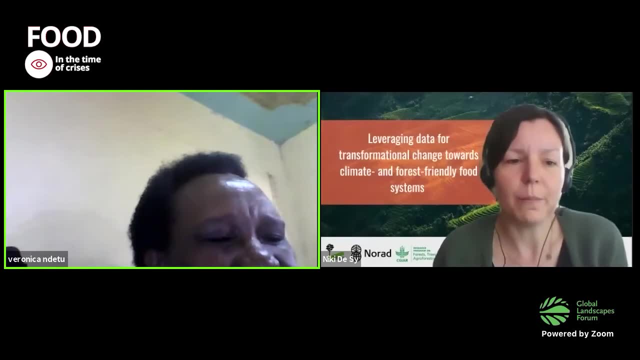 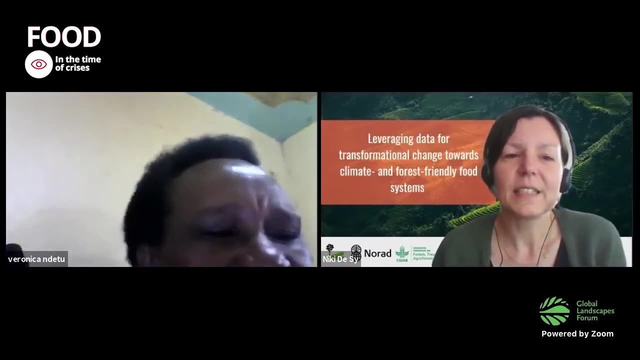 So we do hear you, Veronica, but there is some feedback. Maybe I will put my microphone off to see if that works better, But please go ahead. Thank you, Sorry. I will say that in Kenya we used this data when we were. 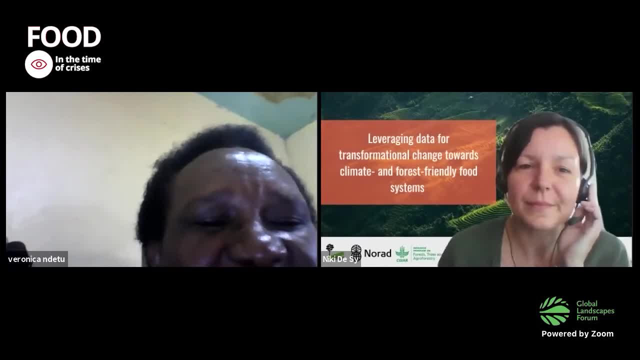 Sorry, my name is Veronica and Dettu. I work for the Ministry of Agriculture in Kenya. I sit in the climate change unit that is charged with the responsibility of mainstreaming climate change issues in agriculture sector, And in the ministry we have developed climate smart agriculture strategy because the sector has committed to implement climate change issues through climate smart agriculture. 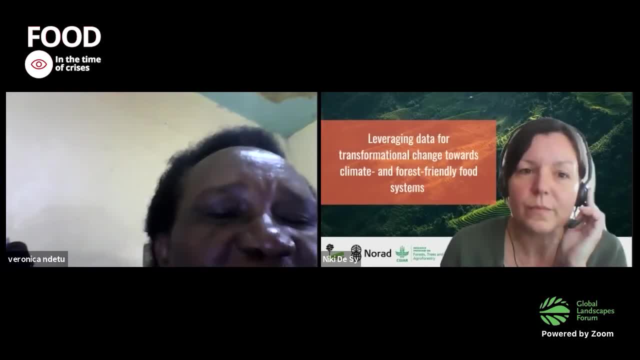 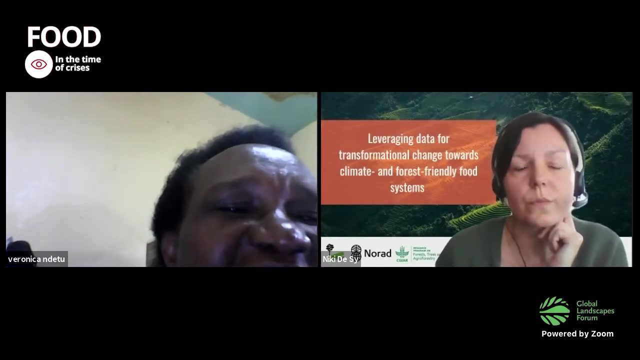 Now, after developing the strategy, the ministry felt there is need to disseminate this policy to the counties, where implementation takes place and where the officers in the counties are charged with implementing or agriculture activities and extension services. So then we partnered with the department of all the departments in agriculture, and we partnered with the CGR centers, FAO and some other institutions to disseminate the climate smart agriculture to ensure that the counties domesticate and they implement, to ensure that farmers adopt climate change, climate smart agriculture. 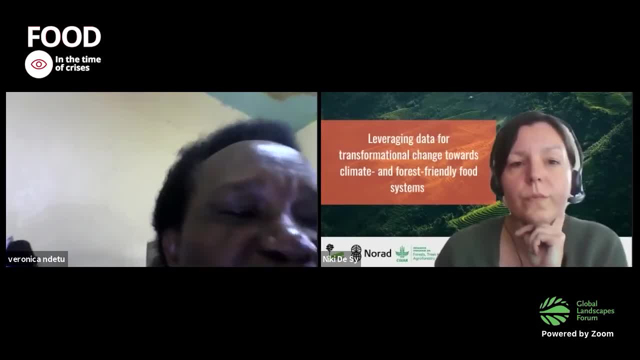 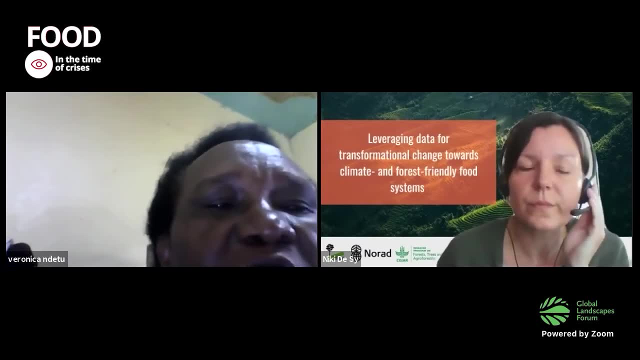 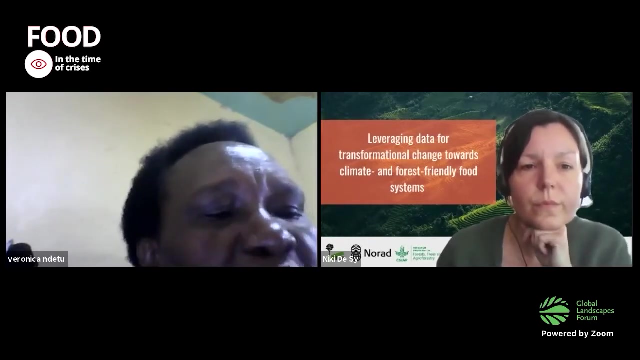 Now, during this dissemination exercise, we were holding workshops with the county officers, both the executive and the technical officers. During this exercise, we were watching in the workshops, which were very participatory. what was involved in is that we ensured that the officers understood and we participated in the workshops. 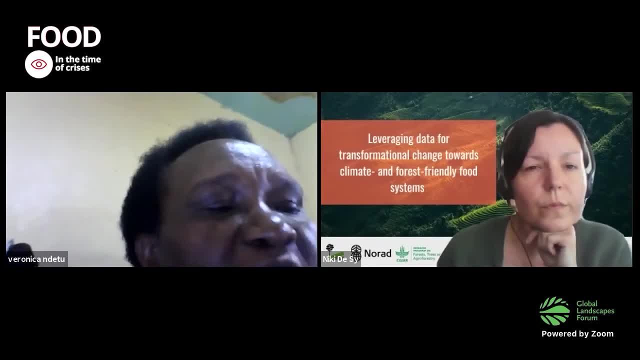 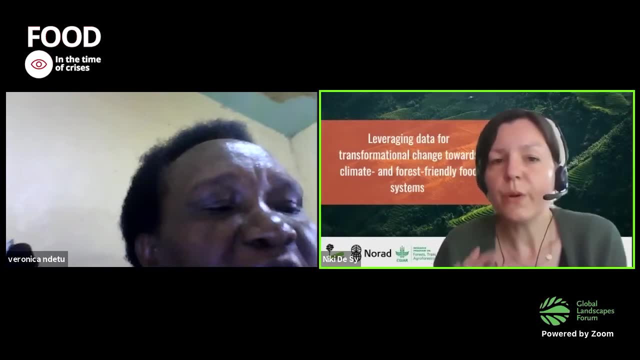 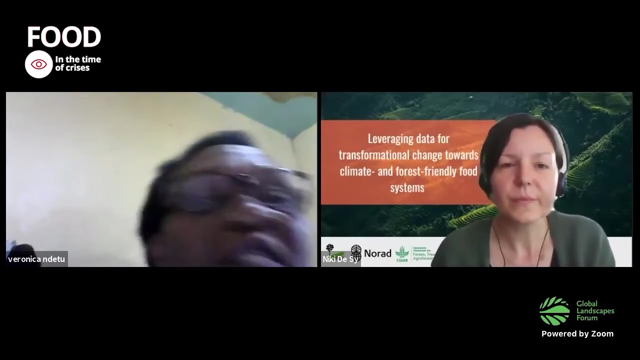 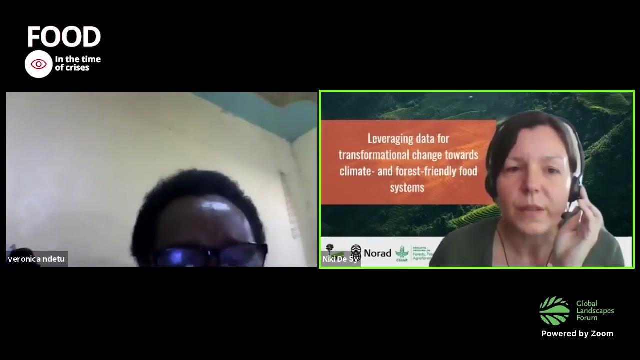 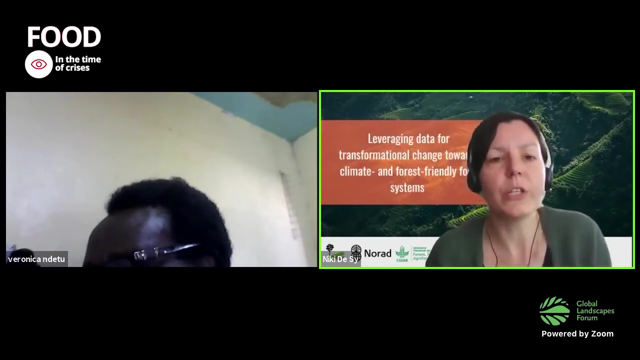 We demonstrated the rule of climate, So now you're falling away a little bit. Veronica, Could you repeat the last thing you said? Okay, we're having some trouble hearing Veronica, So what I understood is that you used this knowledge that came from the ERA database. 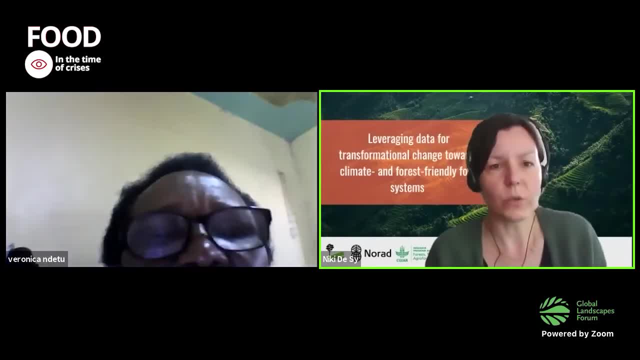 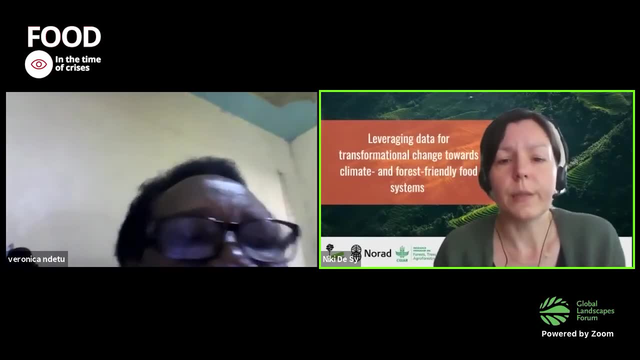 to really implement agricultural practices also at the county level, right For adaptation plants. So what would you say very shortly is sort of one of the biggest lesson learned from that experience, Or one of the challenges. What you learn from this experience is that there is need for continual enhancement of 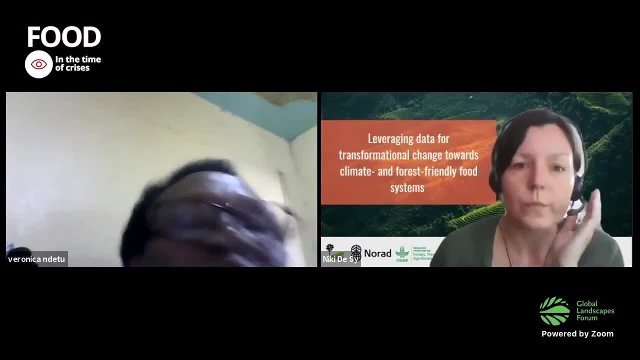 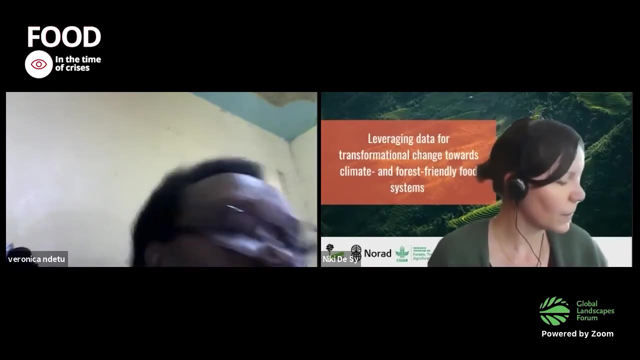 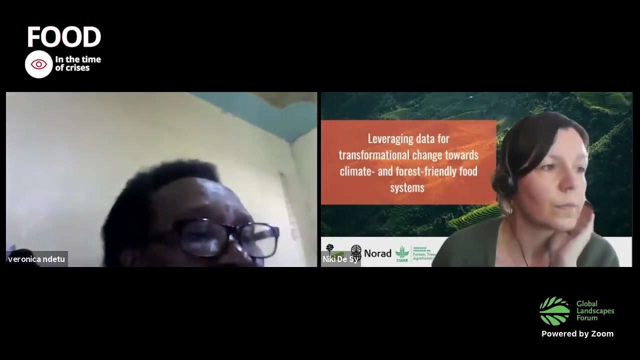 appropriate capacity, especially for the people that interact with the farmers, And there is also need for collaboration between the different players, the researchers, the policymakers and the extension services. So we need to have platforms to create awareness and we also need platforms where we can be. 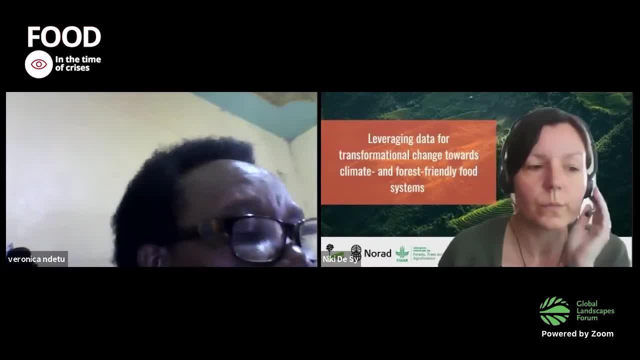 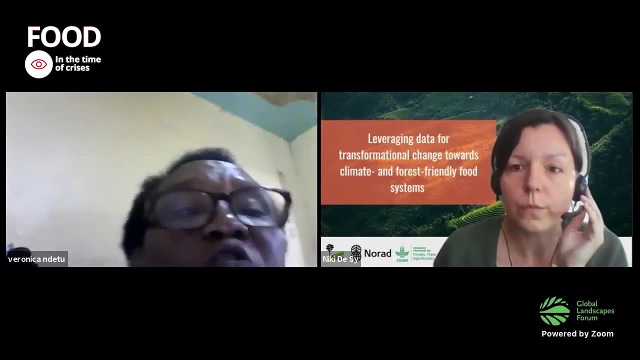 having a sharing understanding of the findings, what the test looks like, getting evidence for options and then choosing the right options to enable the field workers to choose the right options for their patients, for their doctors and their life-threatening plants. Thank you, 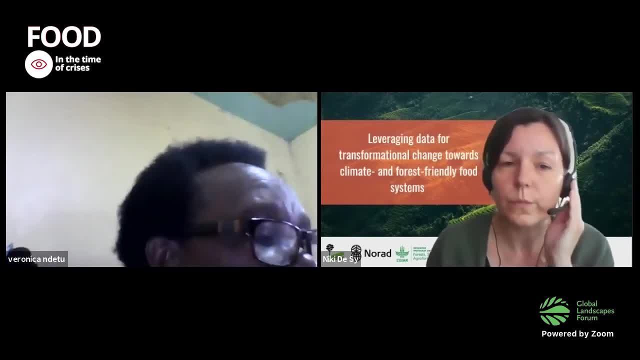 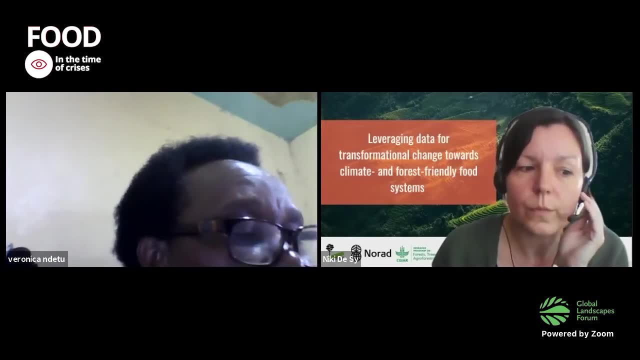 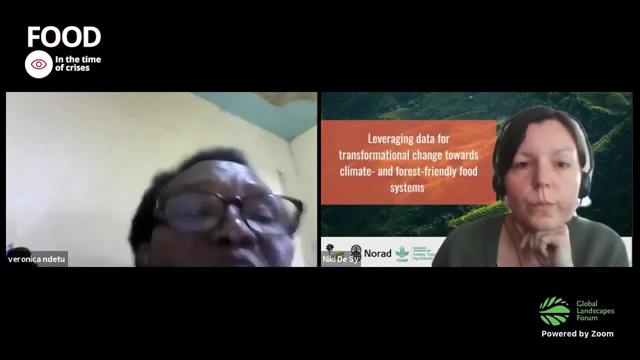 Thank you very much, Thank you. So that is some of the things, And we also need to define data needs and develop tools for data presentation and also easy access and use by the policymakers and the service providers. Thank you, Thank you very much for that. 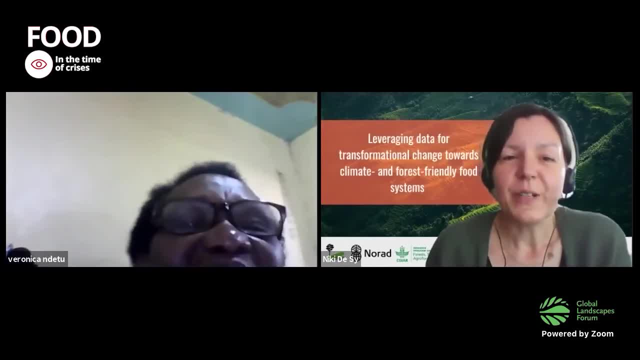 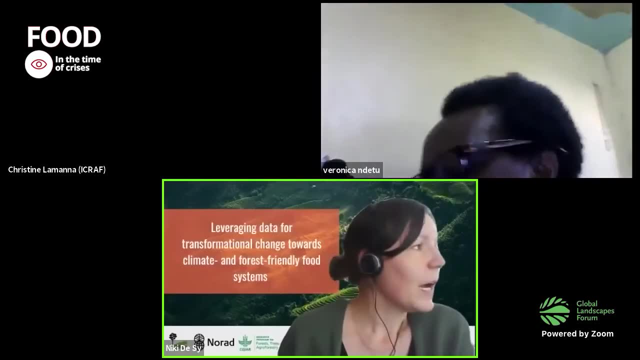 I also want to invite Christine to join with her video. I at the moment don't know whether or not I can get her to join us, But I have the pleasure to be here with her. I at the moment don't see any questions popping up from the audience. 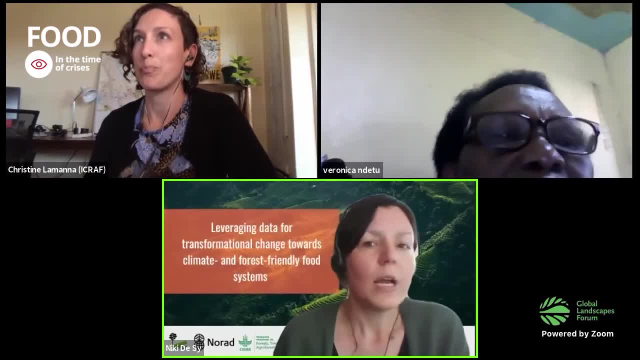 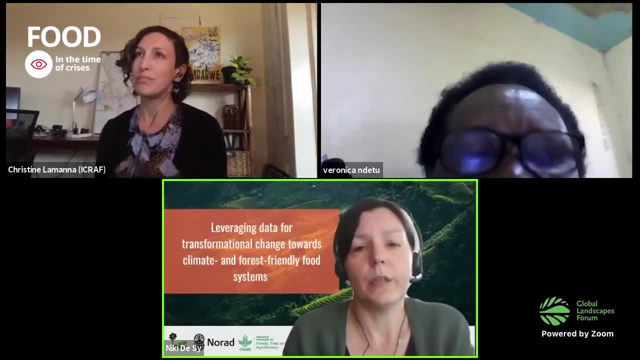 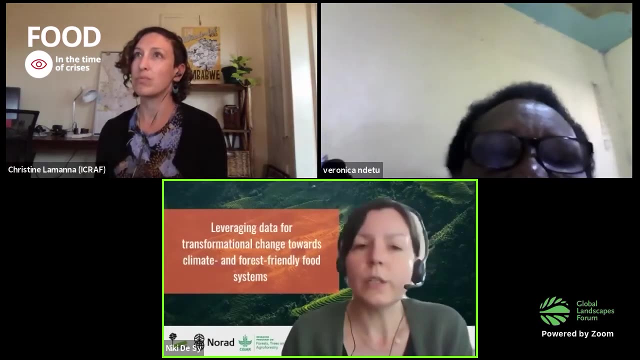 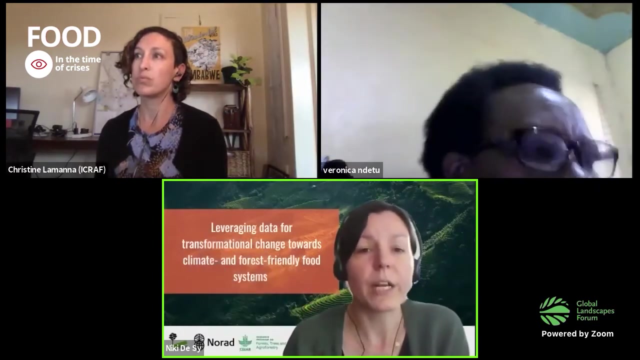 So please, people watching, feel free to pose your questions, But I do have a question, maybe for the both of you. So also, when you think about changing, really transforming, the agricultural sector, So is there still specific data or something that is missing to really develop long-term strategies towards more sustainability? 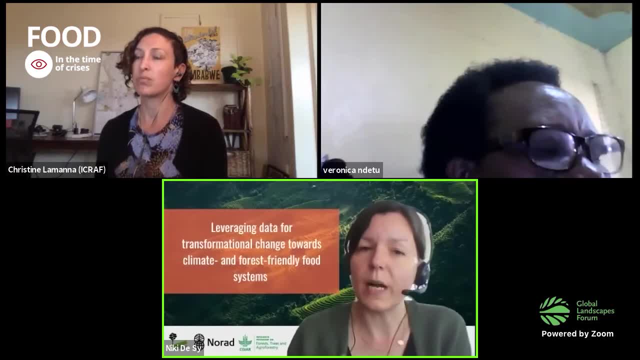 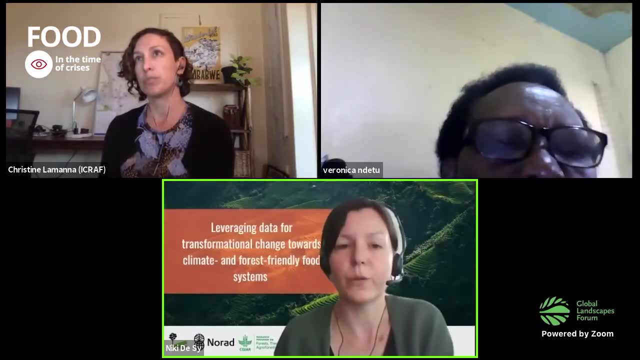 I saw also from your presentation, Christine, that there's a little bit of a disbalance in the data or the kind of things that are being researched, So I would like shortly to hear your reflections on that from both of you, So maybe Christine can start. 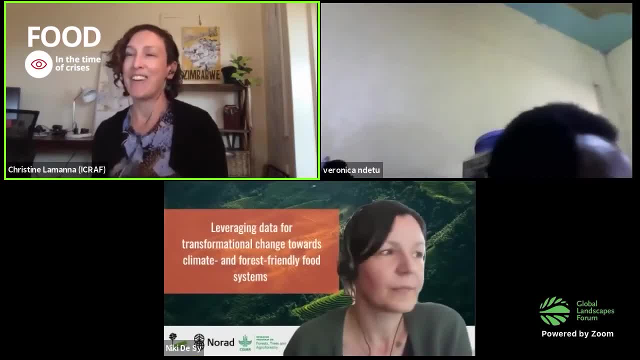 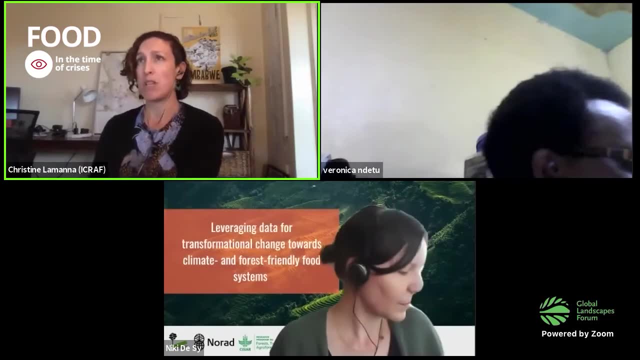 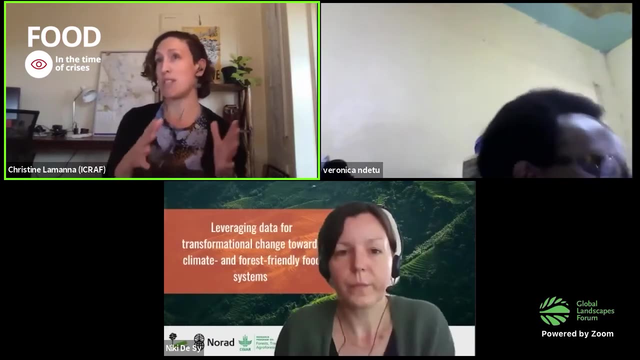 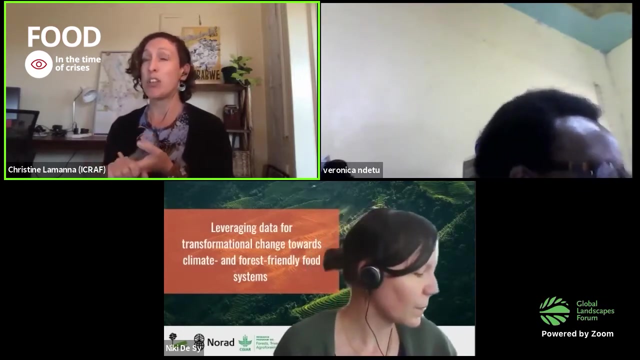 Sure. Thanks so much, Nikki and Veronica. It's great to be able to join you on this virtual conference. One of the things that was really surprising to me when we started putting together all this data was that there were big gaps in the information that was available compared to the crops, the farming systems and the technologies that smallholder farmers, especially, are actually using or actually depending on for their livelihoods. 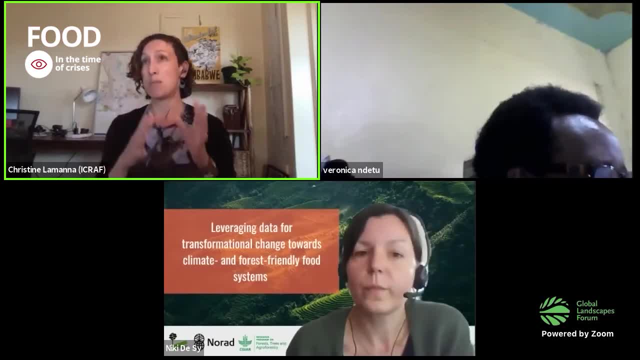 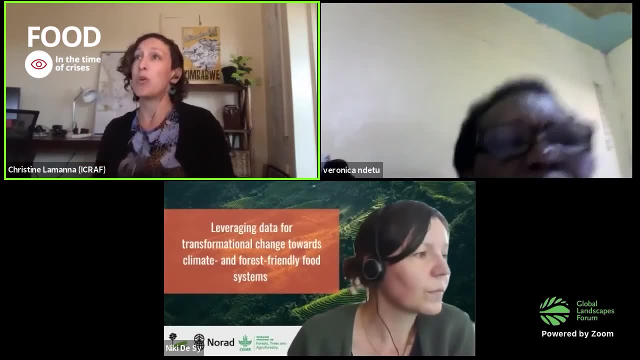 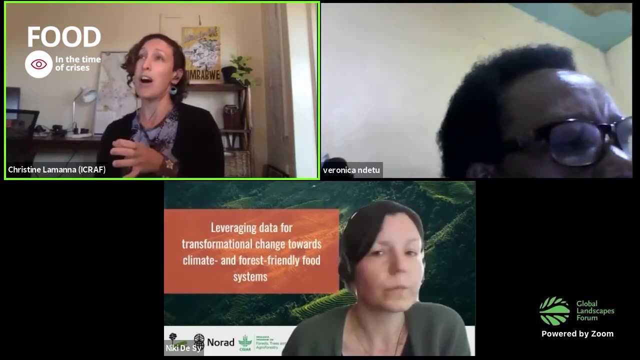 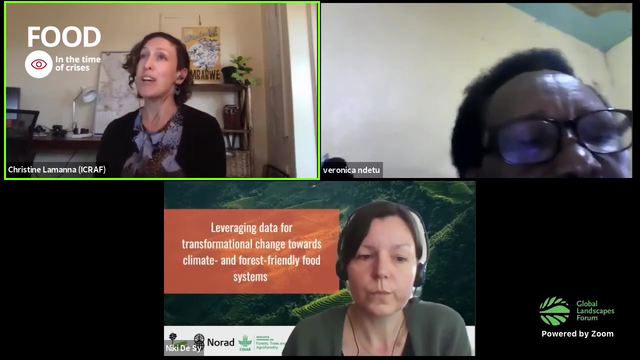 There is often big disbalancing, There's a disconnect between what's been studied or tried and more indigenous practices or locally relevant crops or even whole farming systems that have often been skipped, And so I think what this does is actually sets a really clear research agenda for both international, national and regional kind of research groups to really start kind of gathering the evidence that we need for this agricultural transformation. 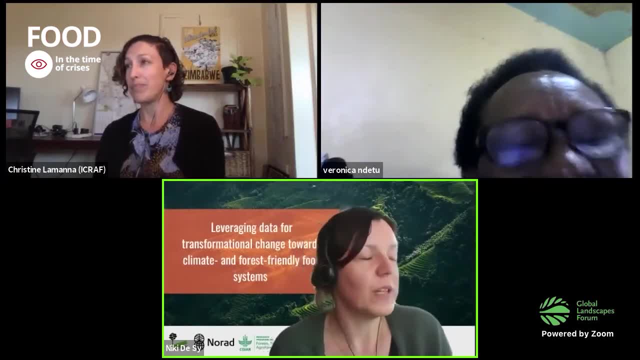 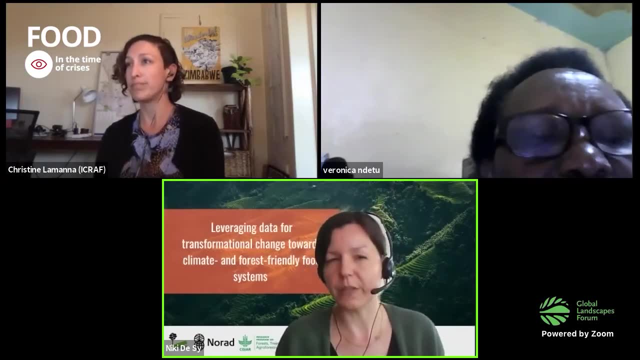 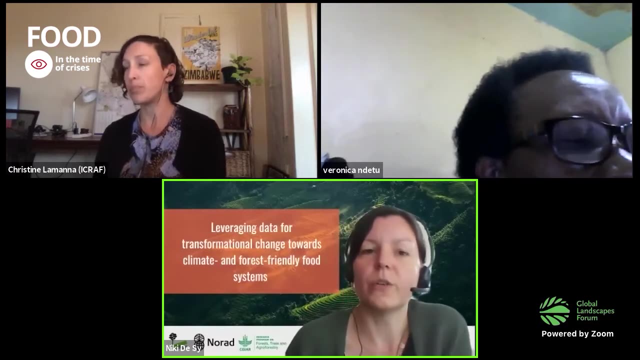 That's very interesting, because now a question came in and asking what are the most important steps to start solving this desert, this data desert. But I think you already kind of answered that right, that you just really, you know already identifying them as a first step and really focusing more attention on closing some of these gaps when it comes to crops or systems. 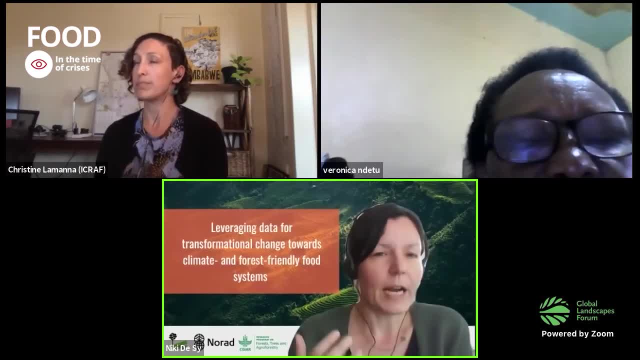 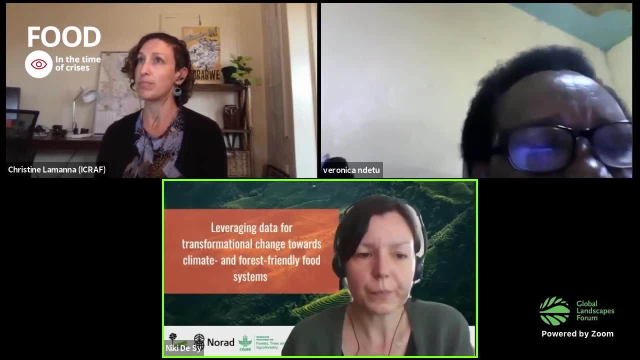 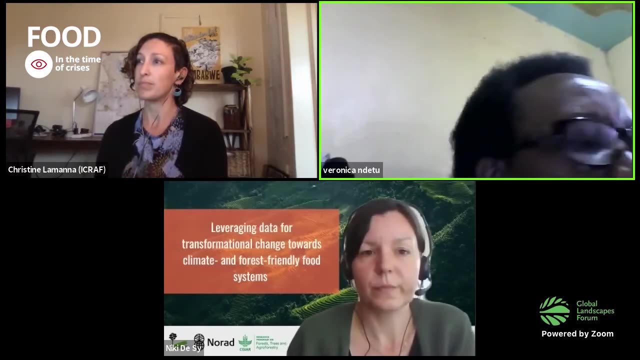 So, Veronica, from your perspective, do you have anything to add on that sort of what? what did still the data needs are for for making you know more long-term plans? yes, thank you. uh. what we observe is that there is great need for uh data and information, and especially uh on future scenarios and the 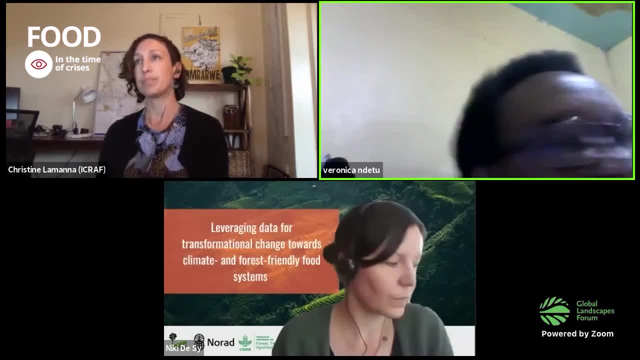 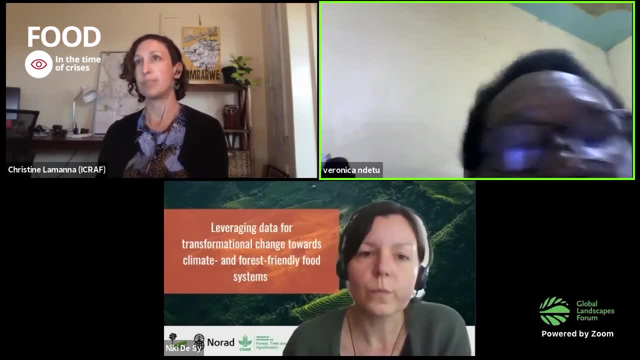 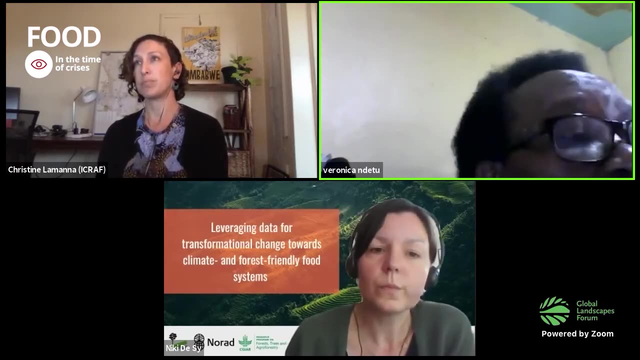 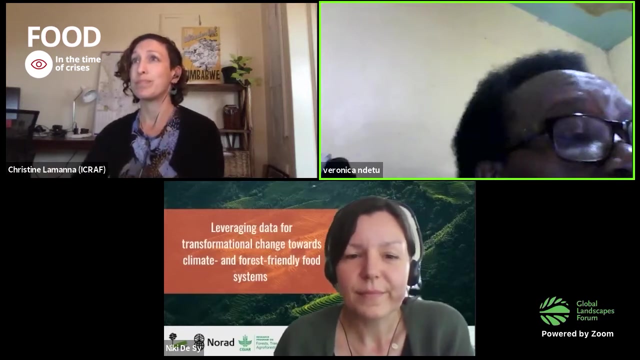 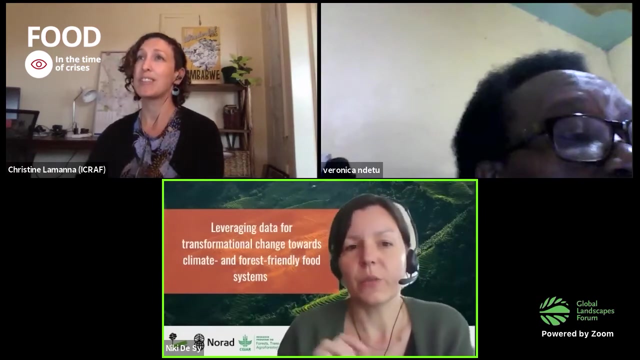 current climate change scenarios, because we need to understand, or the actors need to understand, the impacts and vulnerabilities of the agriculture in the country, of agriculture in the country. we also need to look at the enabling. so it seems like your sound is failing again, um, but we can come back to that later as well. um, environment, so, which can be. 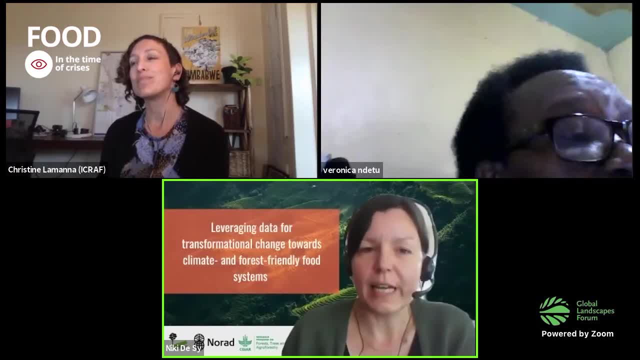 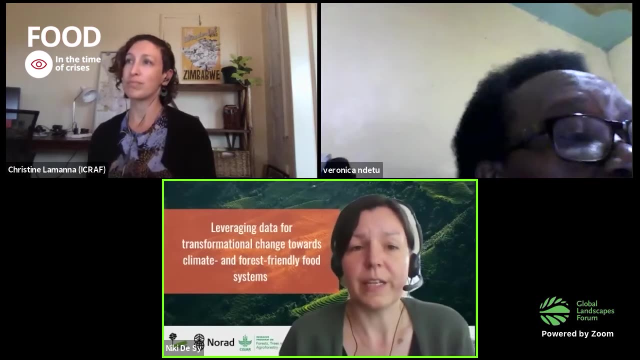 so what i understood from what you just said is that we, that you, also need an enabling environment to make that happen, right? um so, um. so your sound is falling away now a little bit, so i suggest that we move on to the, the next topic already. yeah, we just have a short time now. we'll come back also to some of these. 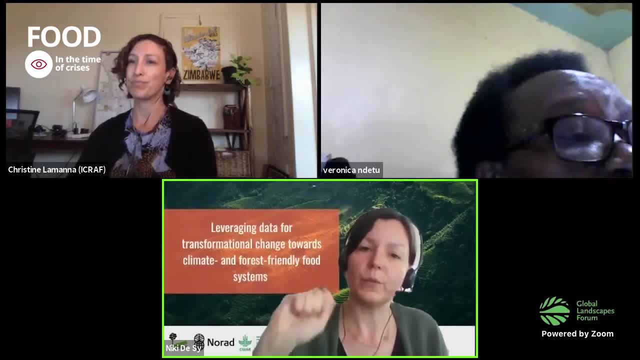 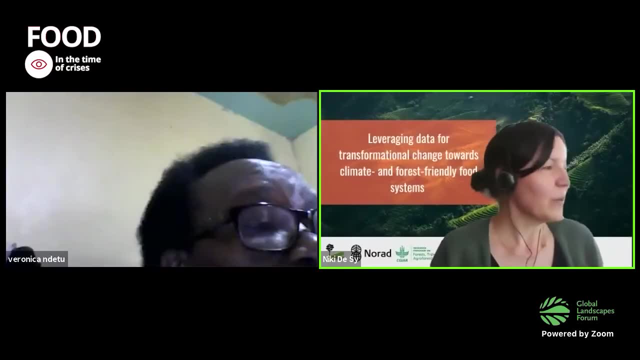 topics in the panel discussion. so if you could just um turn off your video again and mute yourself, then we we can move on. uh, great, thanks a lot. i think it was already very interesting. um, so our next topic is about near real-time monitoring using satellite imagery. 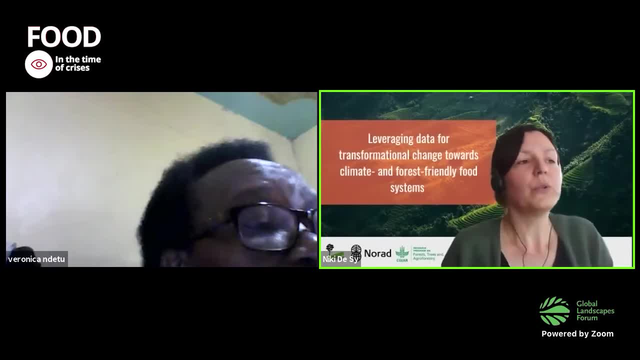 which is a fairly innovative technology that is, for example, used for deforestation alerts, for sustainable commodity supply chains chains and for natural resource management. so we'll we'll watch another video now. this video is a little bit longer, about 10 minutes, because we have, uh, three perspectives. we will hear from the science side, from the, the provider. 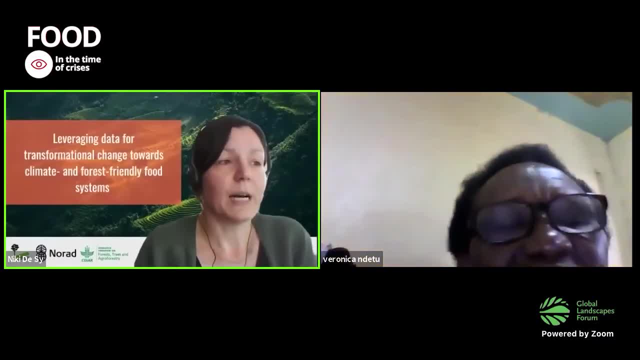 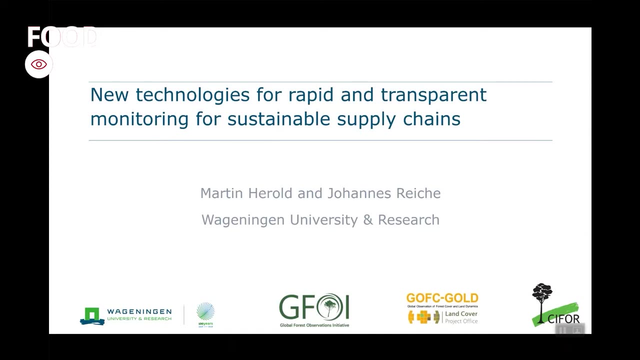 of the alerts, and we also have a wonderful, wonderful example of an operational system that the government of peru uses for their protected area. so please start the next video. hello and my name is martin harold. i'm from wagner university in research. i'd like to 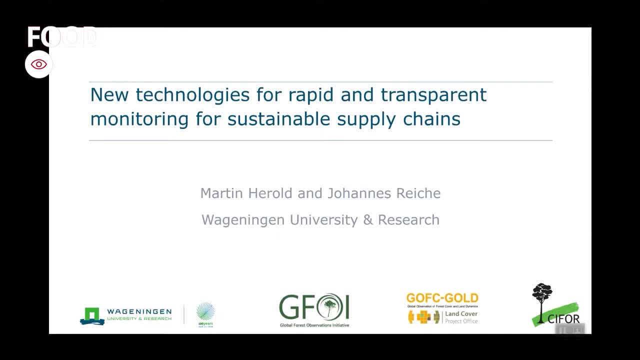 kick off that part of the session to talk a bit about developing technologies and their usefulness for sustainable supply chains. uh, sustainable supply chain? of course we're trying to solve environmental issues along with providing important goods and services, and we have to really do that. quite differentiated observation needs, quite similar to the policy cycle, so we 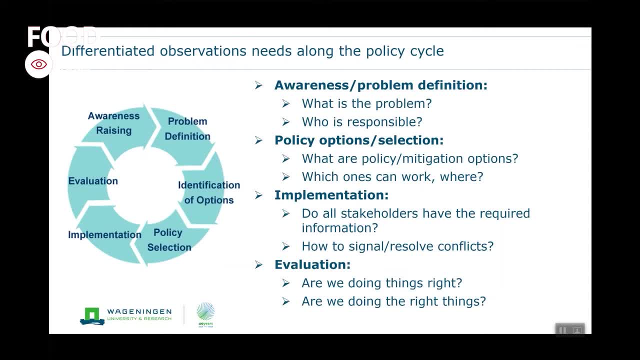 have to first understand the problem. we know that tropical deforestation is an issue. it's driven by also agriculture expansion and commodity expansion. we have identified that managing these supply chains more sustainably zero deforestation pledges and, for example, we can actually do something about it, and then we would like to implement that, and for that we need to know. we need to know whether all 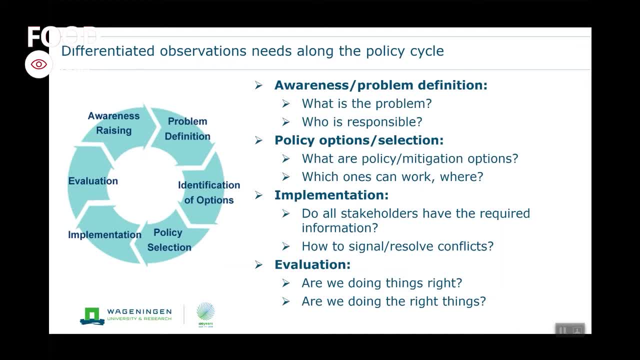 the stakeholders have to require information. is the information it's needed on the ground to do the right things? is it really available, or can we signal conflicts, uh to resolve them, and things like that, and of course we regularly want to evaluate. so how are we doing, uh, is divorce station really? 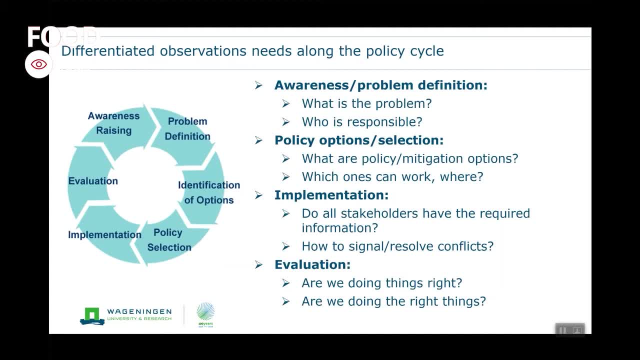 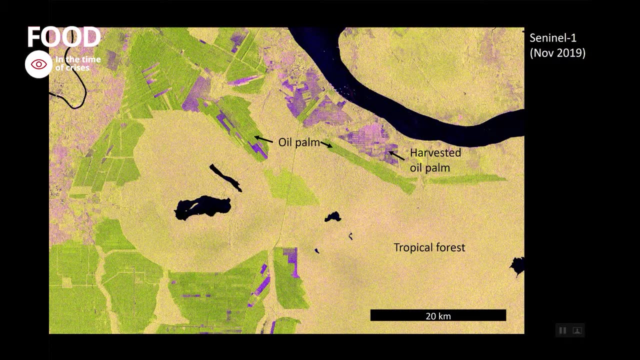 going down, or is it actually the right approach overall? so are we doing the right things? and so, to give you one example on how such new technologies can help us to do exactly that, and I'm gonna show your landscape in indonesia, where there's oil palm, tropical forest. you see green, a lot of. 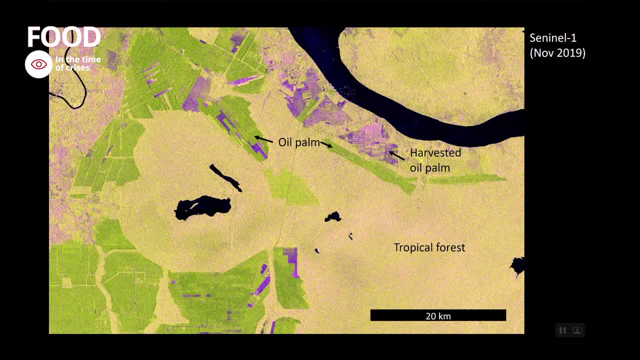 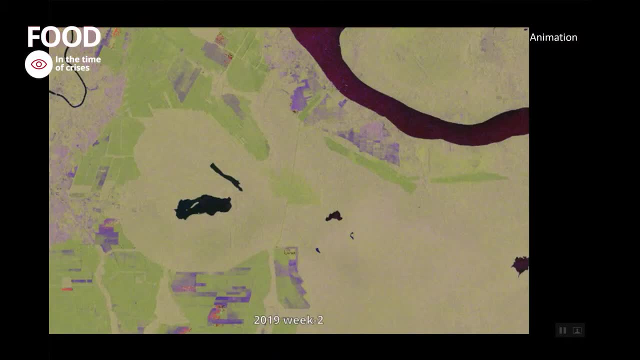 oil palm, and this is a radar satellite from the European commissions and the one that radar looks through clouds, which give us the opportunity to get quite frequent observations. so we're looking at weekly data and everything in red is basically new clearings. these clearings happen a lot in. 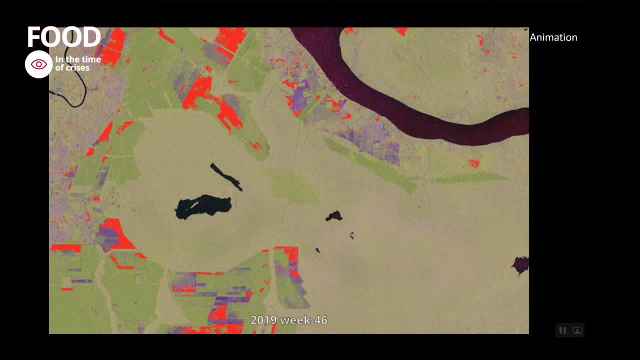 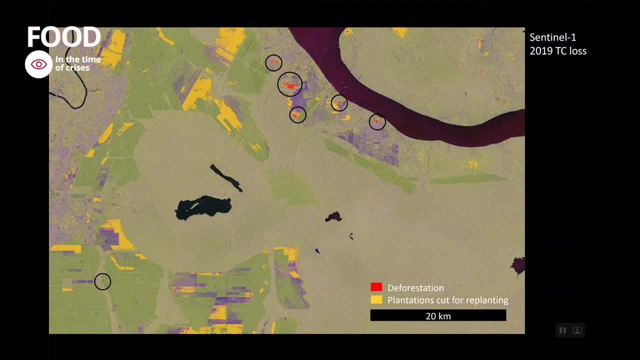 existing oil palm plantations, which is basically plantation management, But occasionally we also see that clearing is happening in natural forest next to plantations, And that's what's signaled here in the red color. So this is actually in terms of sustainable supply chain management. 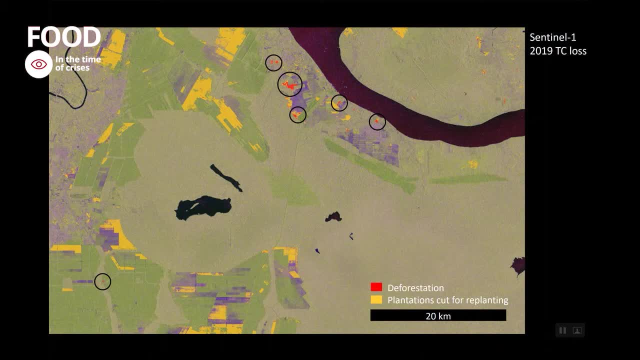 some unwanted changes, and having information about these changes quickly, So on a weekly basis, having it openly available to all stakeholders, ranging from the supply chain company, the local land manager, the civil society as a whole, the consumers as much as other local stakeholders, is very important, So something can be done about it. 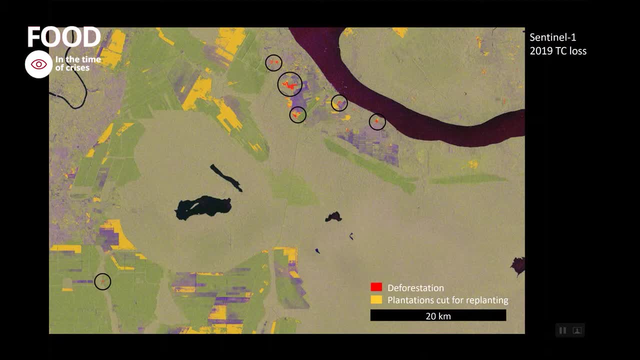 And that is a good example where we see, OK, we have understood the problem, but really for implementation, also doing the right things, We have information that's actionable because it's timely, It's very accurate to provide to the local level. 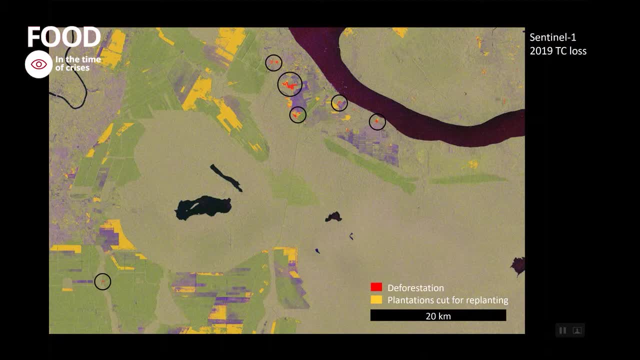 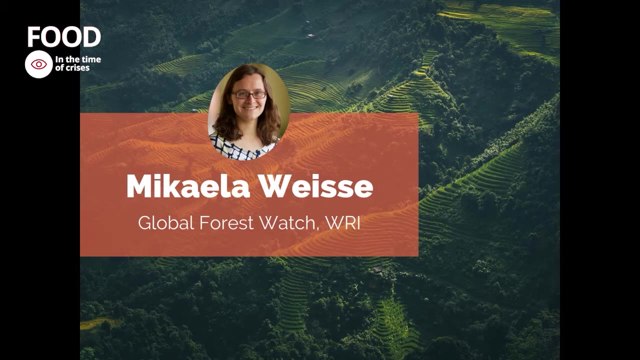 And we can basically do that globally. All these systems are globally, but with local relevance, And that's where we have a nice example on how we can really make sustainable supply chain monitoring a reality. Hello everyone, my name is Michaela Weiss. 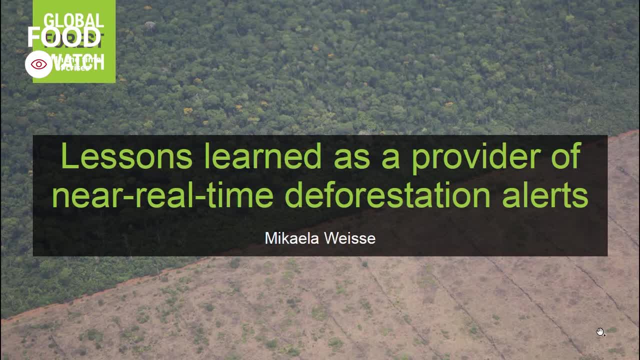 and I'm a project manager with Global Forest Watch at the World Resources Institute, and I'm going to talk to you today about my experience working with Global Forest Watch and providing your real time deforestation alerts and also as part of a case study, to try and understand how users in Peru 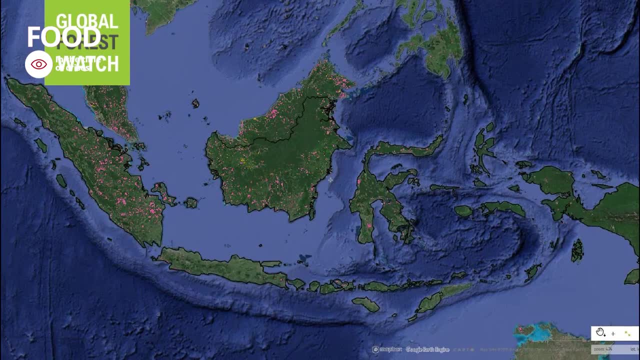 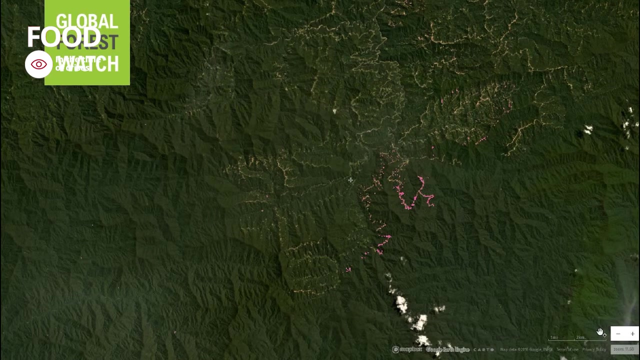 make use of this information. So, first of all, for those of you that aren't aware, Global Forest Watch is a free online platform that provides information based on satellite information about where forests are changing around the world, And in recent years we've been focusing especially on near real 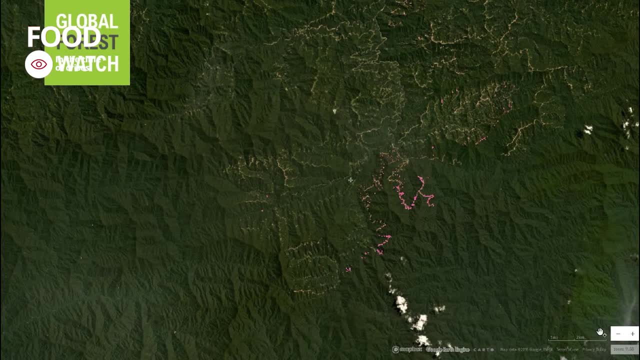 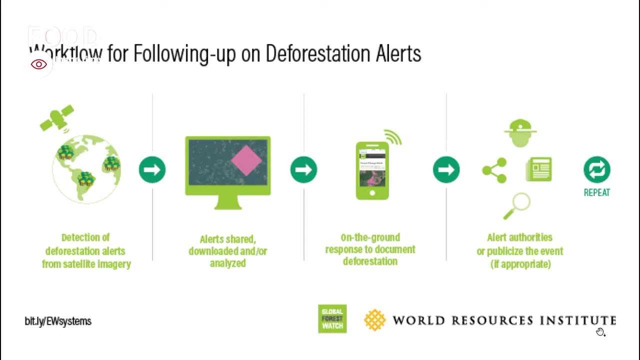 time alerts that show where changes happens as quickly as possible. In our work we've seen that there's generally a workflow of how this information is used and followed up on. First, an institution like Wageningen University or University of Maryland is actually doing analysis of satellite imagery to detect where deforestation 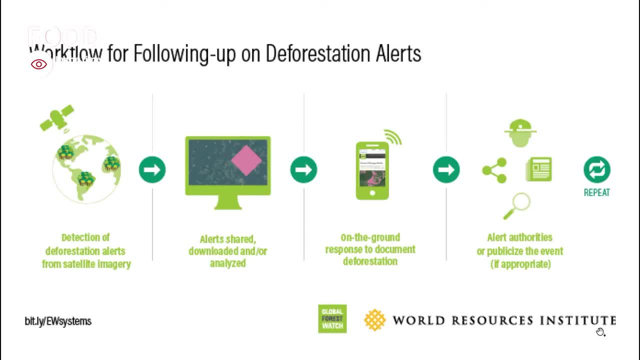 might be happening. and then Global Forest Watch comes in really in the second part of making those alerts available to download and view and analyze so that people can really get a sense of what's happening in their area. And then the third and fourth steps are really happening more on the ground. 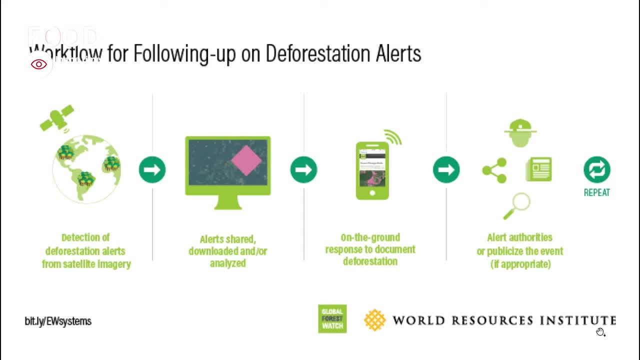 Right. So in the third, having some kind of response to document the deforestation, whether that's a field visit or talking to local people or using high resolution satellite imagery, and then the eventual goal is to have some kind of an outcome of the alert arriving to authorities or having some 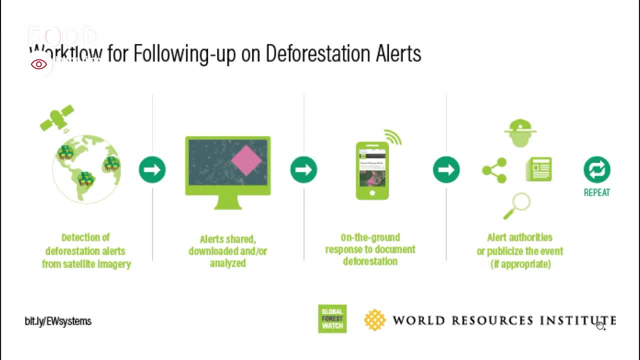 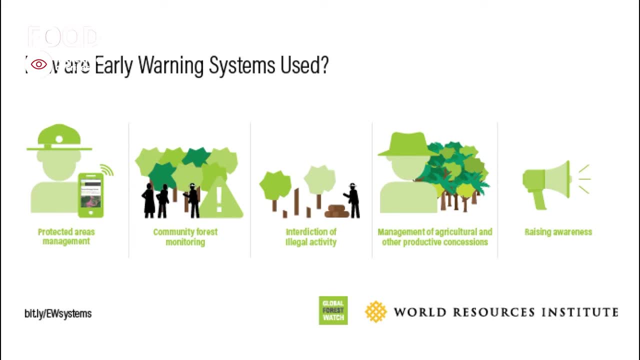 kind of public information about what's happening in a particular area. In our work we've seen that there are a number of different users of these near real time deforestation alert systems, Everything from understanding or protecting protected areas and other federal lands to indigenous territories, to private company land holdings and also 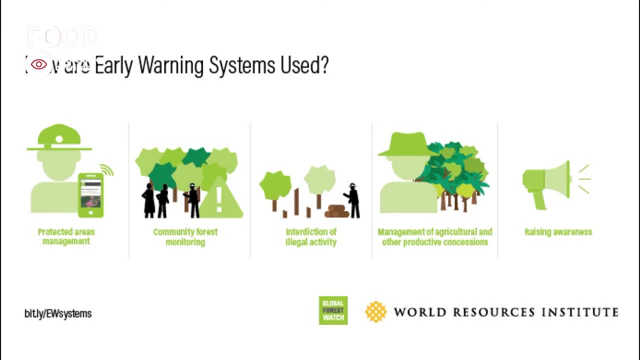 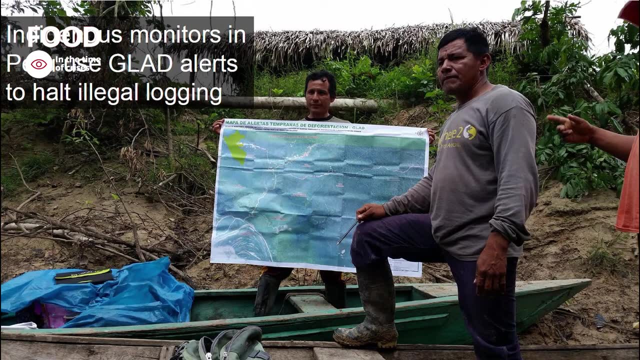 just by media and civil society trying to raise awareness about recent deforestation. So I'll give you just a couple of quick examples. This is a community that I've worked with quite a bit in Peru, along with our partners, the Rainforest Foundation US. 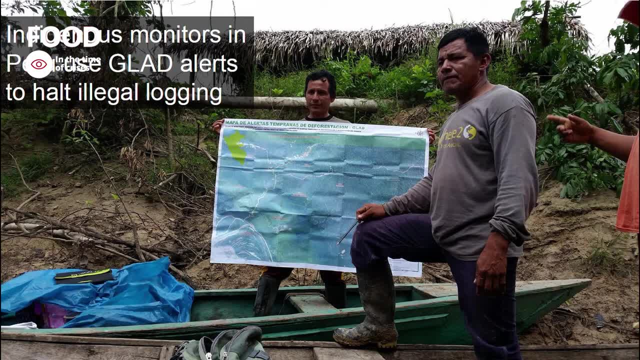 that are following up on deforestation alerts within their territory and then documenting what's going on and presenting formal legal complaints to the local authorities, And they've actually been so successful that in the couple of years since they began monitoring, they now have almost zero deforestation alerts in their territory. 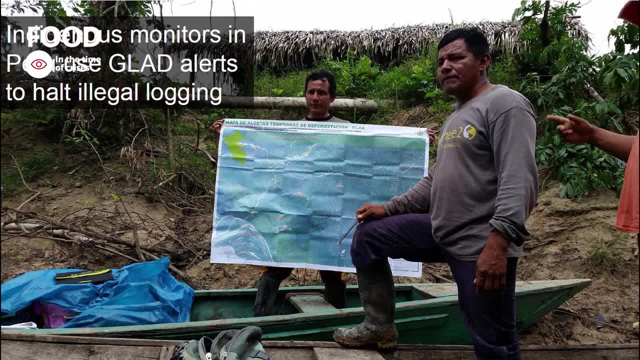 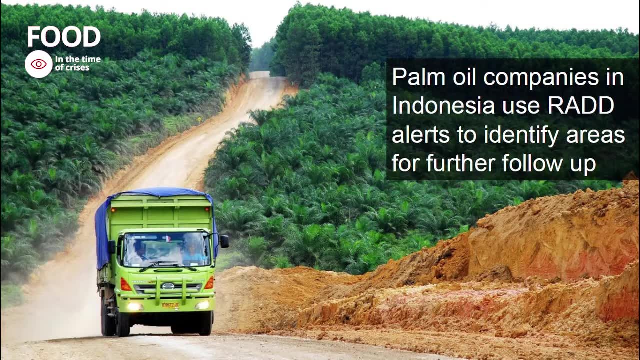 And so they're trying to figure out what this monitoring unit that they've established can do now, potentially on actually restoring the areas that had been deforested in the past. On the other side of the world, we also work a lot. We're working with palm oil companies and, in particular, are working with a number 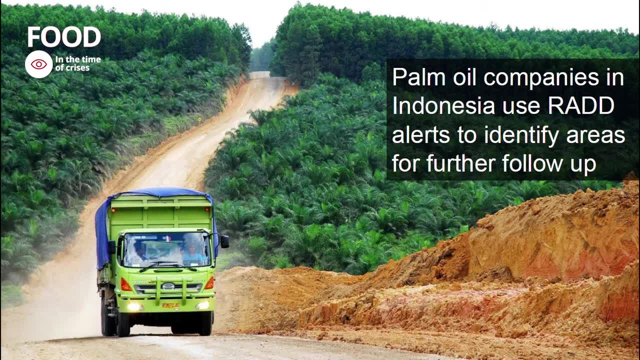 of companies in Indonesia around using radar based deforestation alerts to identify those areas that are highest priority of recent deforestation. So, whether they're overlapping with protected areas or peat or somewhere in the palm oil supply chain, we have a whole protocol for how. 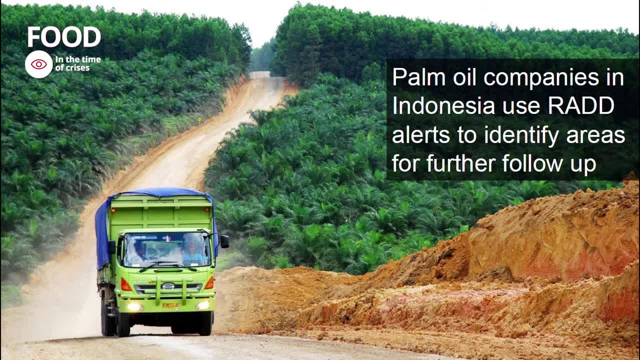 there is a response generally involving sending the agricultural extension workers to document what's happening in a process To ensure that the proper action gets taken by law enforcement and that those areas that have been deforested don't end up as part of palm oil supply chains. 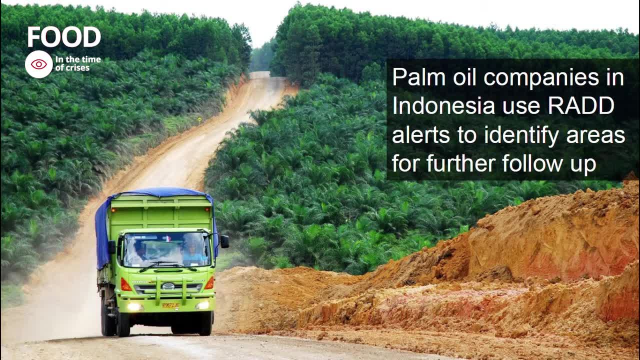 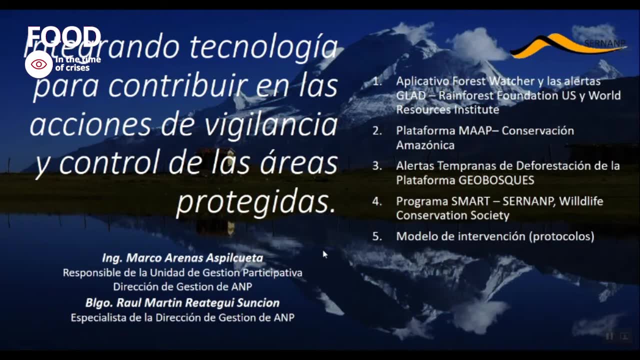 So there's just a few concrete examples of how this information is used across the world. My name is Marco Arenas and I'm accompanied by Martin Reategui. We both work within the service of protected areas in Peru, which is the entity that manages. 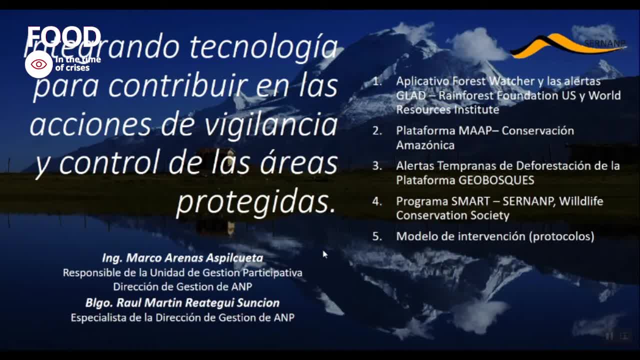 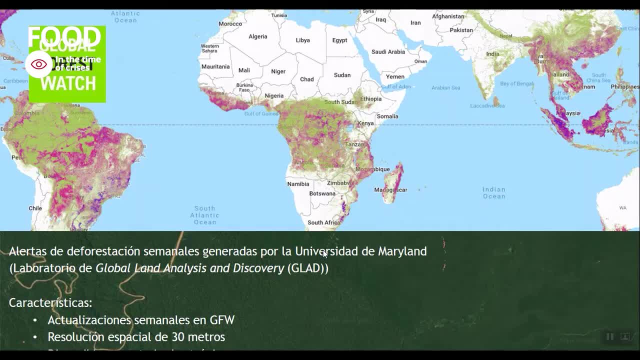 the national protected area system, 75 NPs and more than 17% of the territory protected by the Peruvian government, and a major security block in the Amazon. Let's start with this effort, which is the engine that brings us to this meeting, which is the joint work that we develop with WRI. 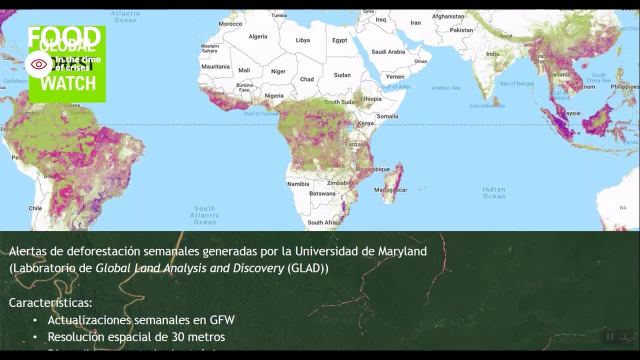 and other organizations, and it is the use of these tools, such as the Global Forest Watch, to have deforestation alerts in this new context that we have in Peru from remote surveillance. So we have a whole process of direct surveillance associated with interventions or properly the park guards, in a direct way with the communities and also 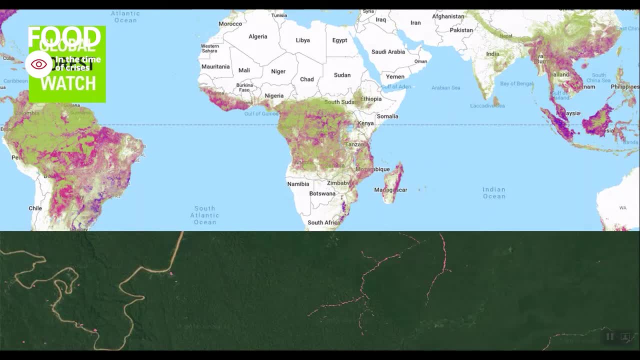 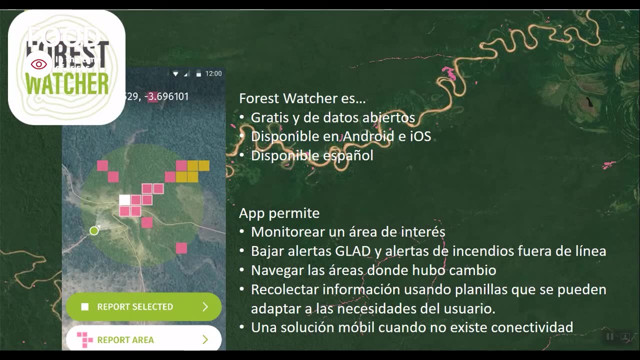 the use of technologies within the framework of remote surveillance. So this type of information is important, especially that it is of practice and easy to use and the language is basic, even more so when we have different languages in the territory, and the Spanish language. 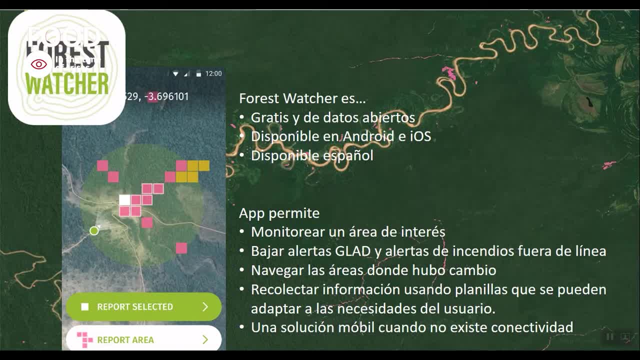 which is the medium with which we communicate with our local partners or, for example, between park guards with which we develop. So this topic is basic, open data and allows us to attend many things, from fires to issues such as the central associated with deforestation. 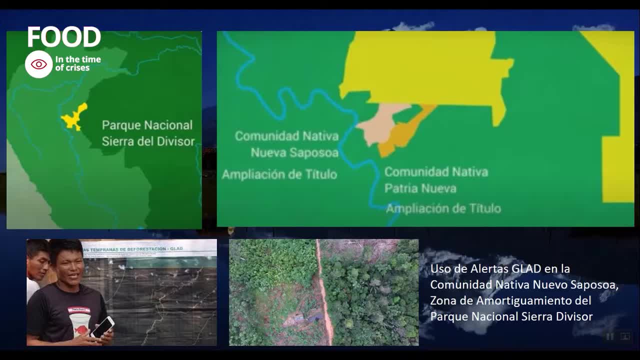 And one can work in the field without being connected with these applications. And here we show you an exercise that we have been developing in this effort of the Peruvian government And the opportunity of initiatives such as DOLRI to work together. So this is an effort that we are developing with a community in the Morte de Viento area. 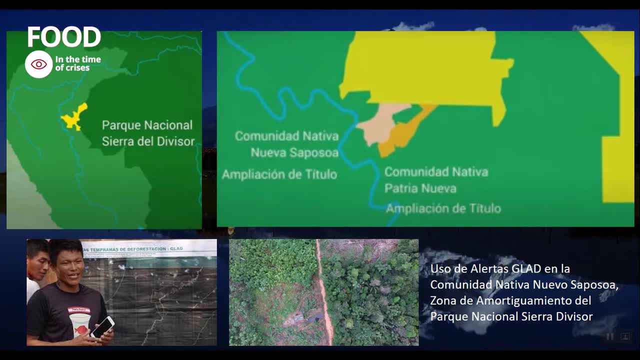 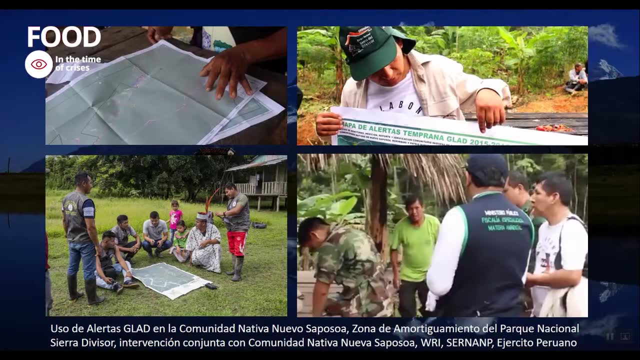 of the Sierra del Divisor National Park for issues, for example, such as deforestation alerts when designing a road or when building an illegal safe road, or other types of interventions such as crop crops that generate deforestation. So here you can see these images. 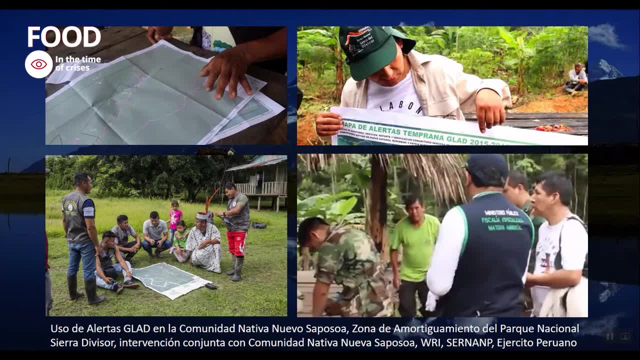 And the interesting thing about this effort, for example, is that not only the army participates, but there is also a representative of the army and also a representative of the prosecutor's office. So with this tool we are more appropriate in our interventions, And part of this great context that we have in this pandemic goes that way. 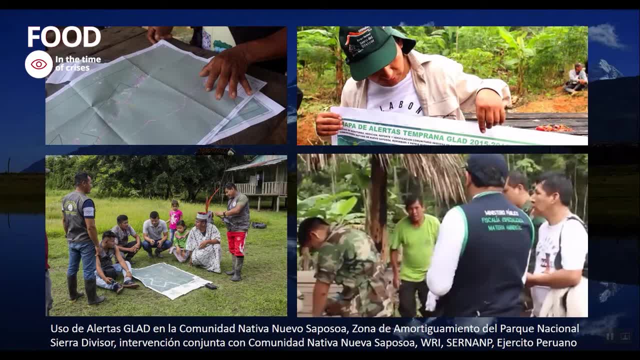 We just released a survey and the needs at the moment is the need to reinforce remote surveillance. so for that we need the use of technologies, that is, information that gives us alerts to be more appropriate in the intervention. Yes, then, because we are going. 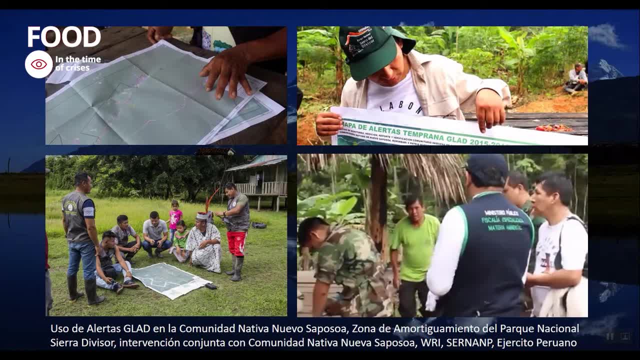 to try to avoid, in many cases, the encounter of people, of people that we would have to develop when precisely an alert that tells me that it is by human activity and I can intervene in a more efficient way. That's where we're going right. 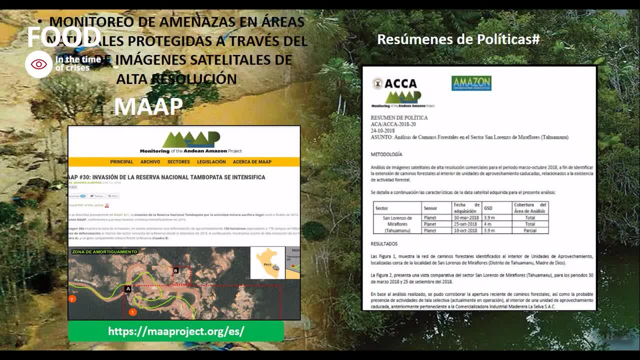 Monitoring is going to be very important in this context. Here we show another experience that we have with ACA for the issue of illegal mining, in the same way with heat fixtures and the use of other images as plans and a report of a political summary. 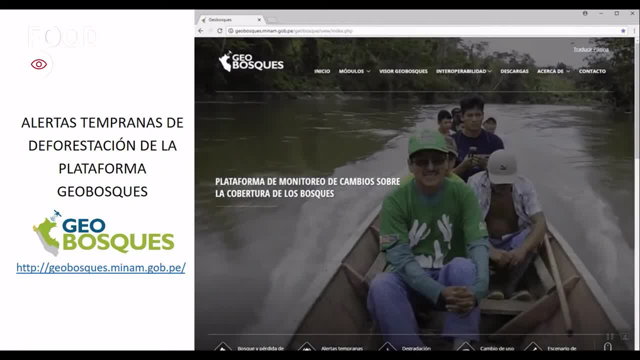 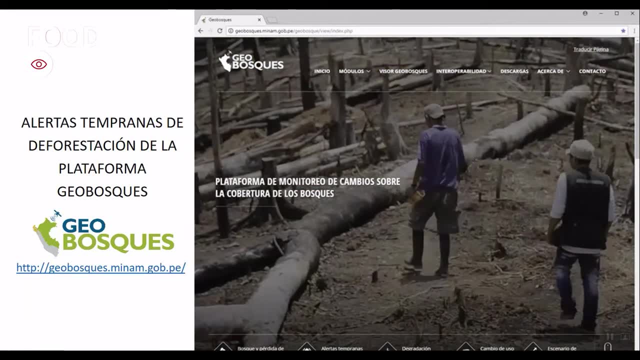 Here we have the other alert of deforestation that we have with the forest program, with which we have been adjusting, calibrating in greater detail with the information of, for example, the loss of forest by natural activity or non-natural right, Or anthropic right. 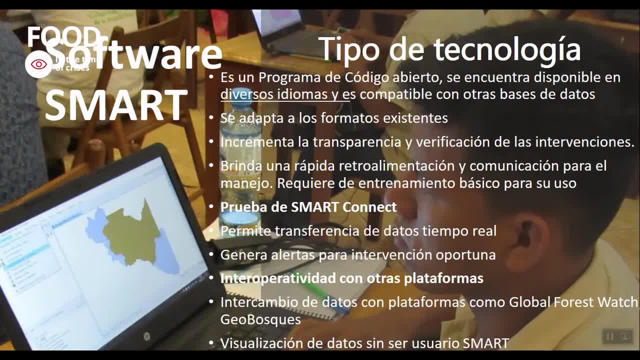 So that's where we've been calibrating And we have a tool that is unlike the other three, which is the one that reports. it is a reporting mechanism which uses the information product of the information, of the alerts, of the technology and of the implementation in the field of the patrols. 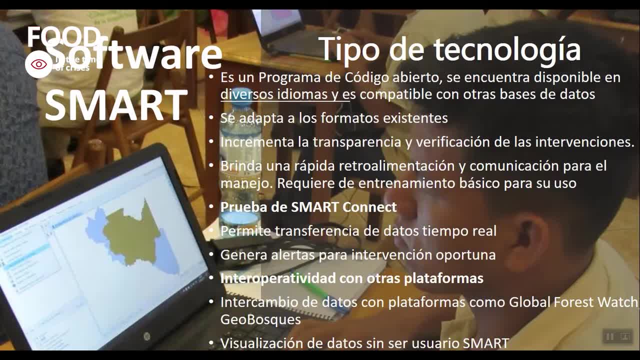 or of the interventions that we will develop for these alert activities as a result of these alerts. sorry for the redundancy. So the ESMAD collects that effort and it systematizes it, it spatializes it and generates reports both for the authorities of the authorities of the ecologies in the territory and also at the national level. 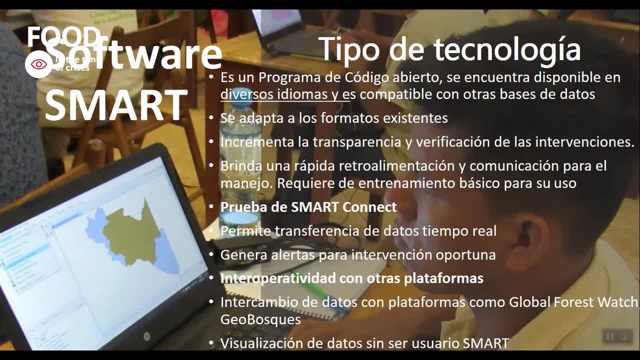 And now the issue At the level of the Ministry of Finance, because it is the one that gives us the resources then for efficiency and to avoid self-reporting in the sense of monitoring these actions. So that's why it's important now, in this context of a great component. 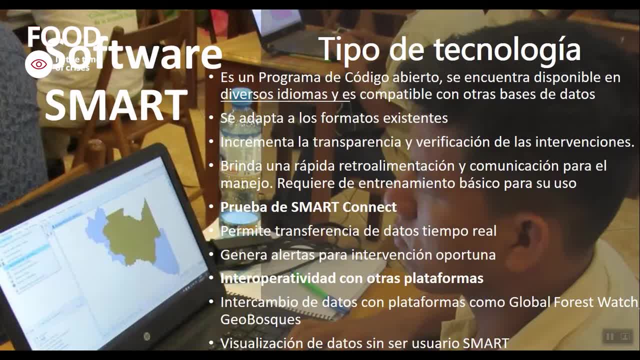 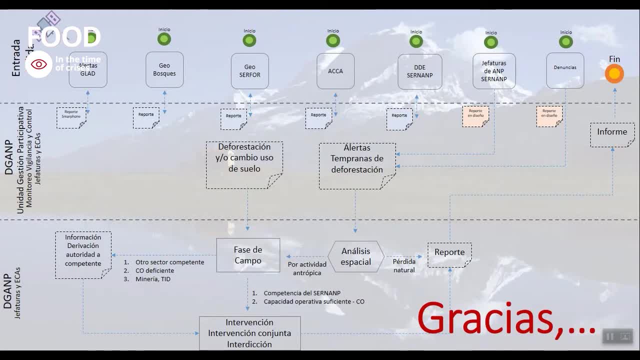 of remote surveillance, and that's why I reiterate the importance of this topic. in Peru at the moment, This is the tool that generates these reports at the system level. And, to finish, this is a process of how alerts are developed, how alerts are consumed. 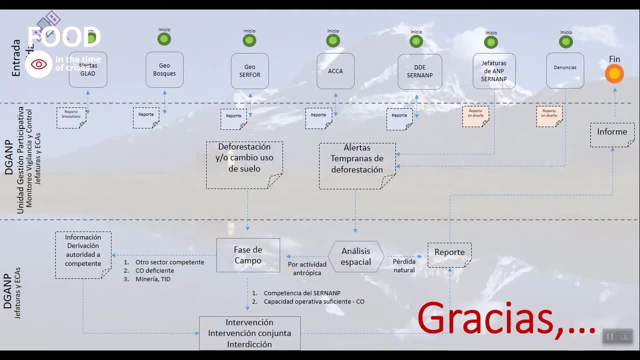 how in the chain of command, within the authority of protected areas- in this case us- and how in the field, interventions are developed and decided. So that's all, Rather to reiterate the opportunity that we have now in this context, where the territory is not demanding greater efficiency. 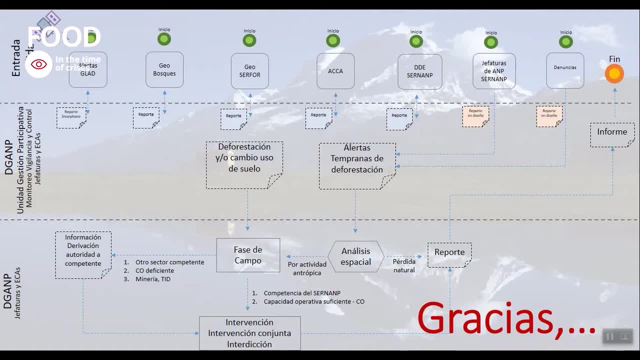 in the interventions and for this the use of technology is going to be the way. So I move the question to WRI and other forces like you to help us in this effort, From capacity development, from innovation in the tools and other activities in a joint way that we can develop. 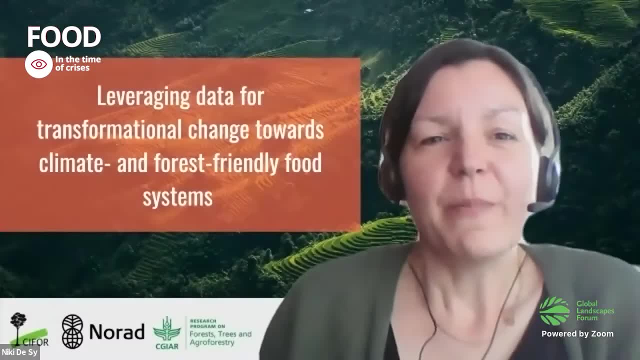 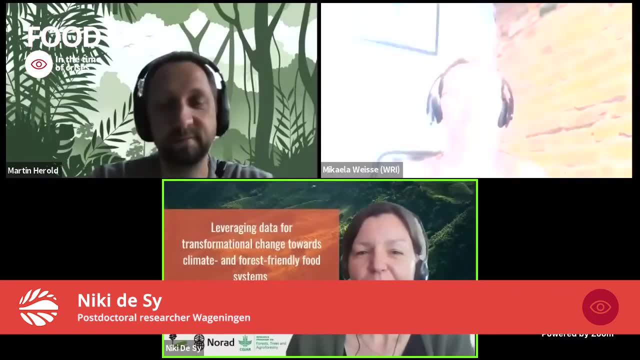 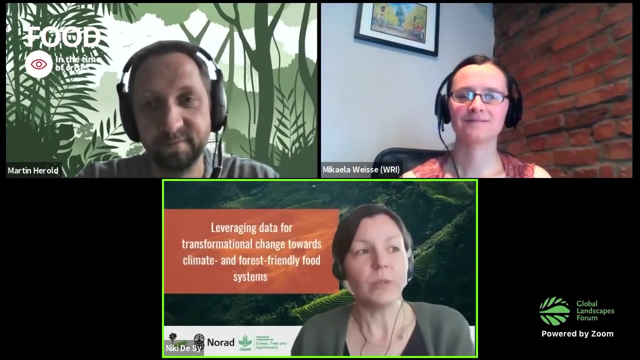 Thank you again. So, hi everyone, We're back again. So I want to invite Marten and Michaela to join me here in the Zoom room. Hi Marten, hi Michaela. Unfortunately, Marco and Marten and Raúl are not here in the live session, but don't hesitate to us. 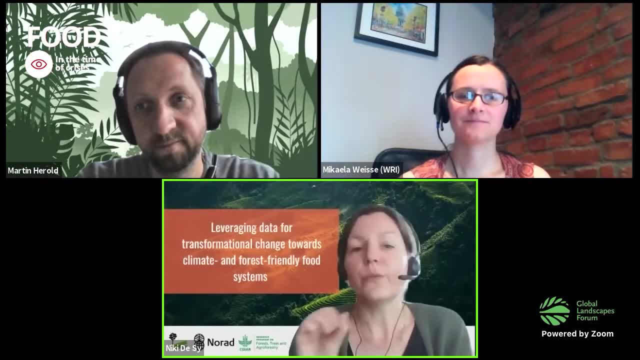 to ask questions that are particularly relevant for them, as we will follow up on those questions after the session, And I know they're very happy to share their experiences with their very elaborate system. So I see some interesting questions popping up from the audience. 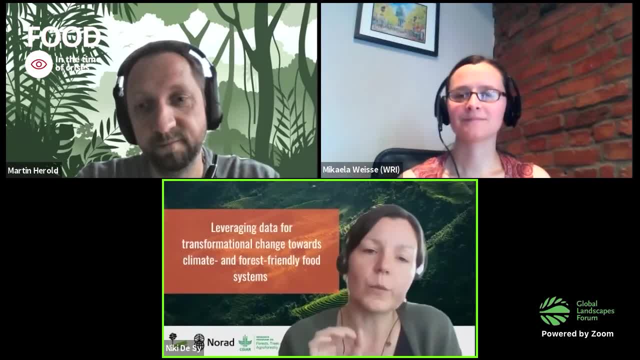 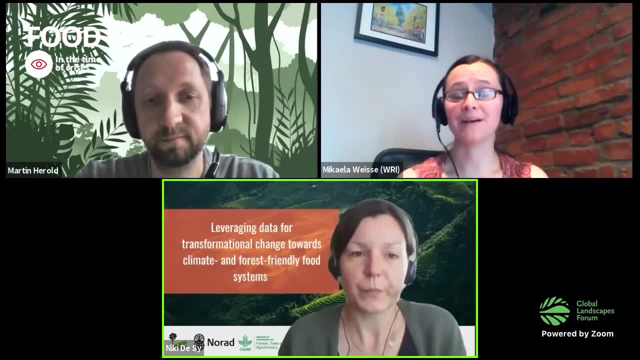 I want to start with asking Michaela if you can share a little bit from your perspective. what are particular challenges that you're facing in this whole chain and in your role? Yeah, that's a great question. I definitely think there are some technical challenges that we have yet to resolve. 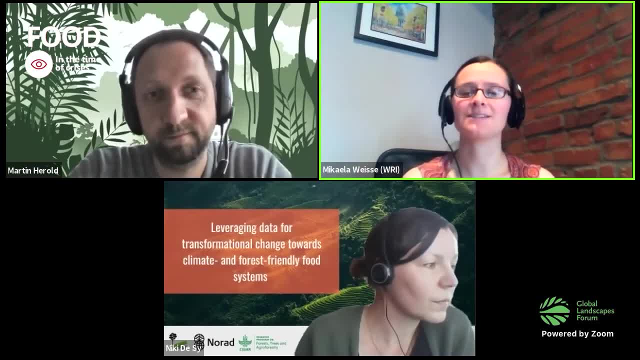 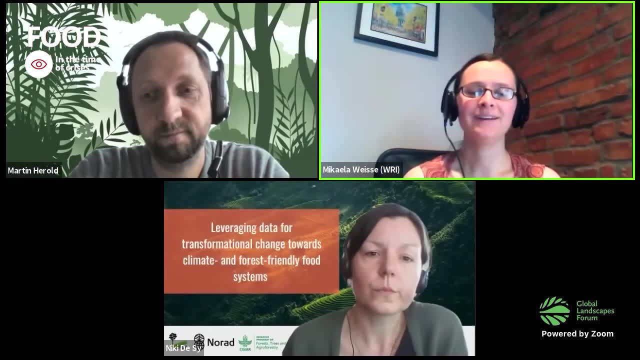 For example, we see a lot of problems with cloud cover in the tropics delaying how quickly we can actually detect deforestation. So doing work with with Marten's group on trying to use radar, also always trying to improve the way that we get these alerts out into the field, 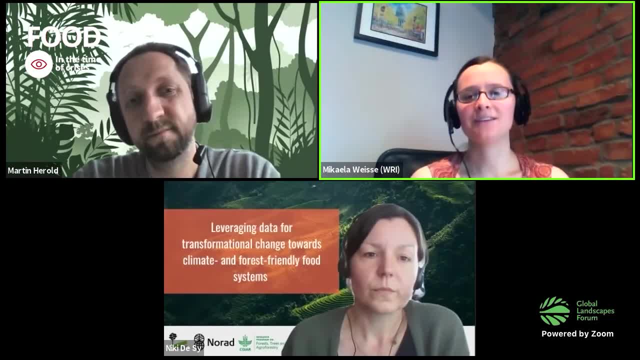 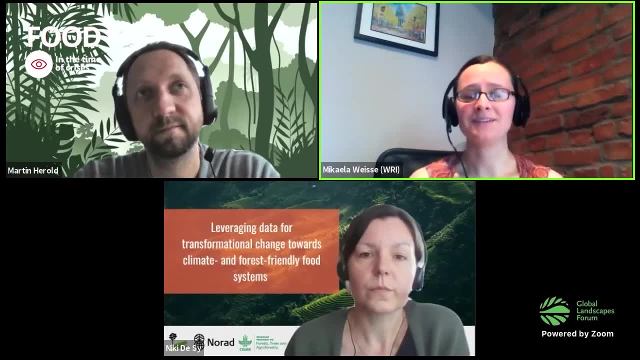 for people who don't necessarily have Internet access. But I also see that there is a large area of challenges, that's more, around the implementation and use of this technology on the ground. So, for example, even just having enough money to buy gas for your boat to get to. 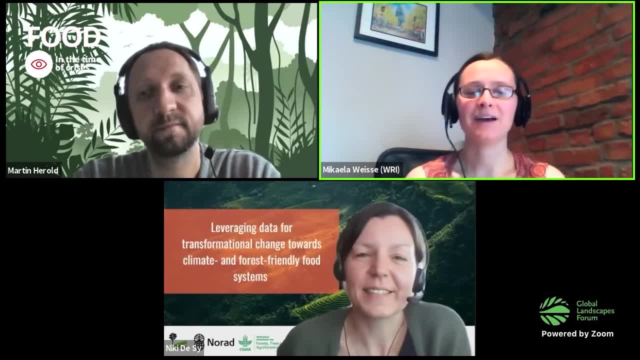 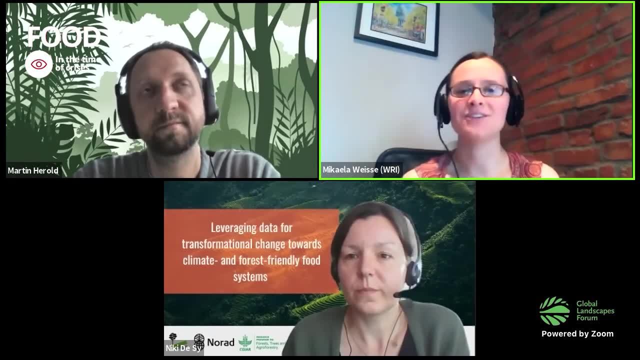 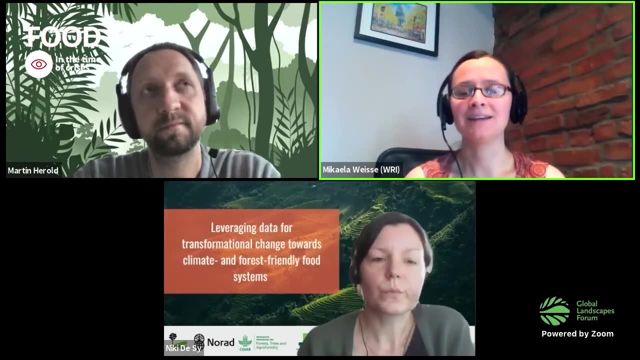 some of these very remote areas of the Amazon can be a challenge- and also different agencies deciding who is responsible to follow up and how do those agencies work together and work with communities on the ground to actually respond when there is illegal activities. And so I think it's really important we think not only about how can we improve these data and make 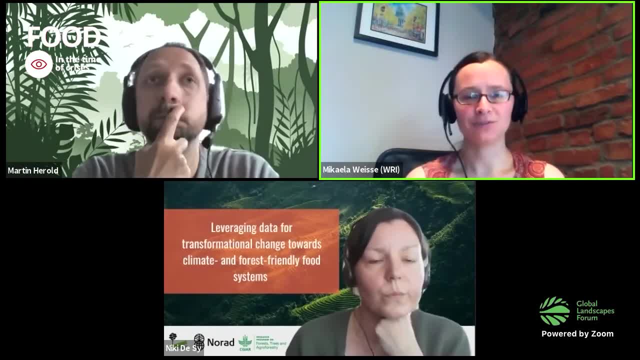 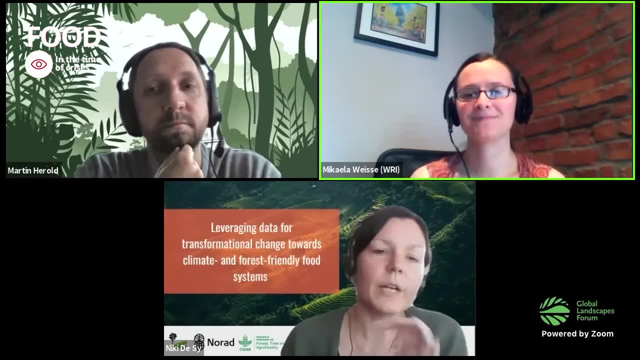 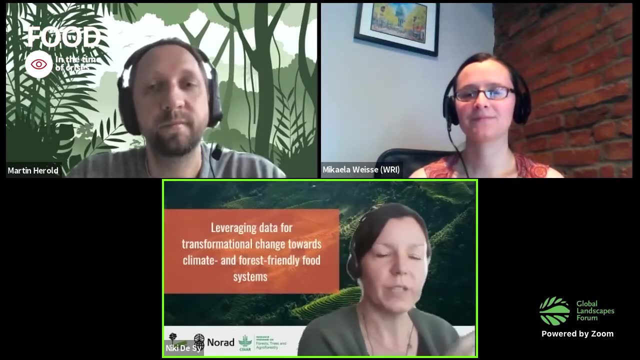 them useful and actionable? but also, how do we make sure that the resources are getting to the ground and that we actually have ample attention to those challenges as well? So it's a bit of a follow up question that also came from the audience. So do you think that the biggest challenge is now in sort of improving? 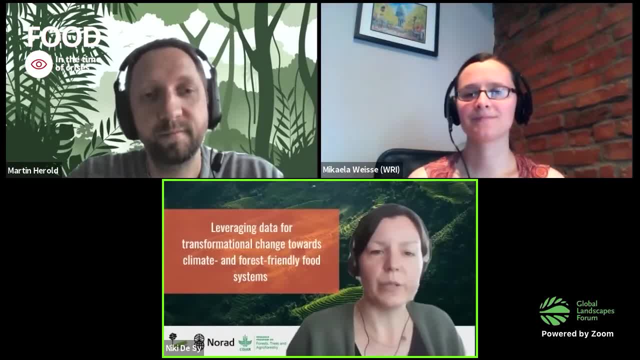 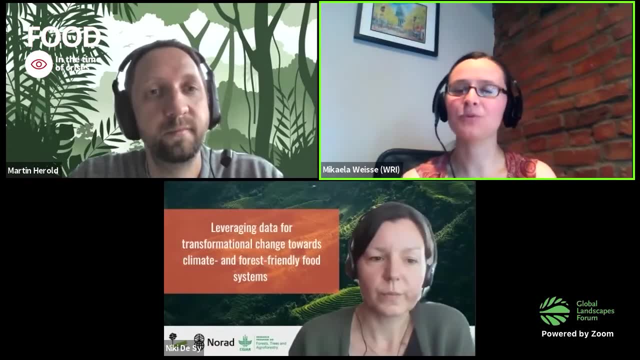 the data side, or really more in this whole chain, or is it a little bit of both? Yeah, I think there's always things we can do to improve the data, And certainly we as Global Forest Watch are kind of aspiring to that and trying to remove any of the remaining challenges. 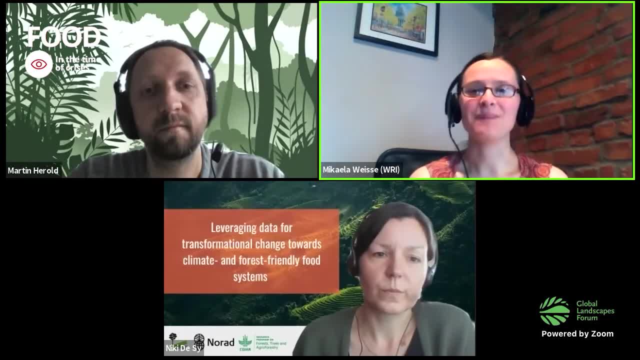 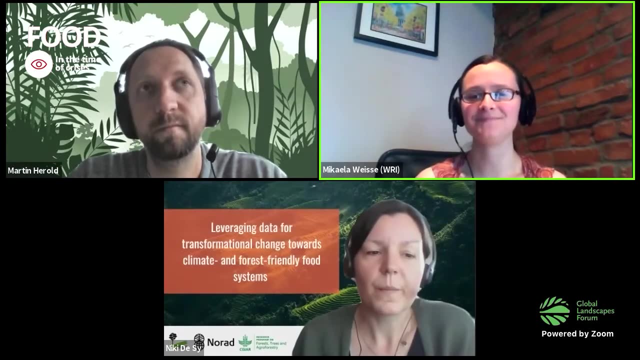 But I think the fact is that we are actually quite good on the data side now. We've made a lot of progress in the last few years and we actually have systems that work And we have examples of how those work on the ground, And so I do think actually the biggest challenge is more on the implementation side. 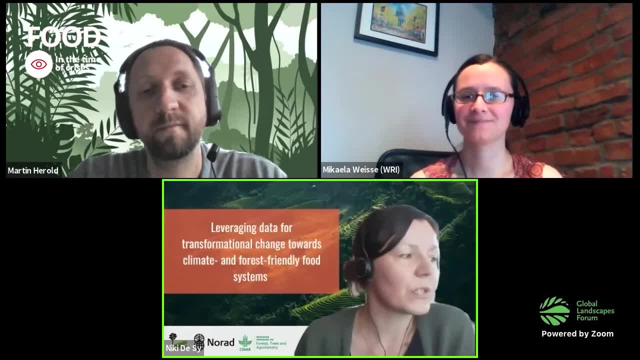 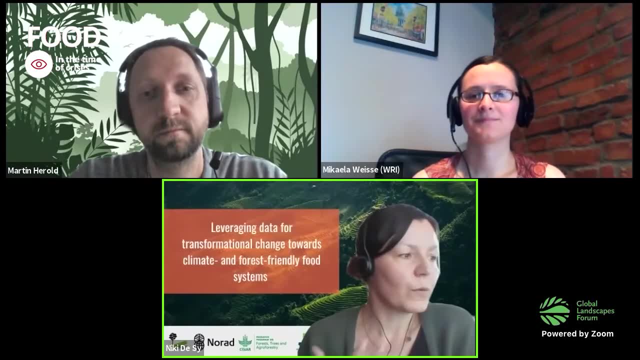 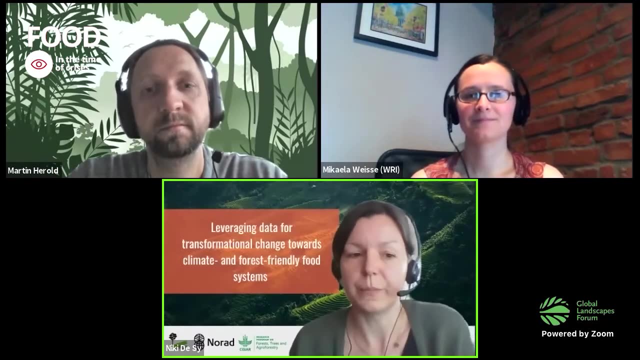 OK, thank you. I'm going to move to Marten now. So there's also questions sort of: So how available or how good are these data also for developing countries? There's someone from Nigeria asking that And sort of: what are the innovations there or what is the outlook there? 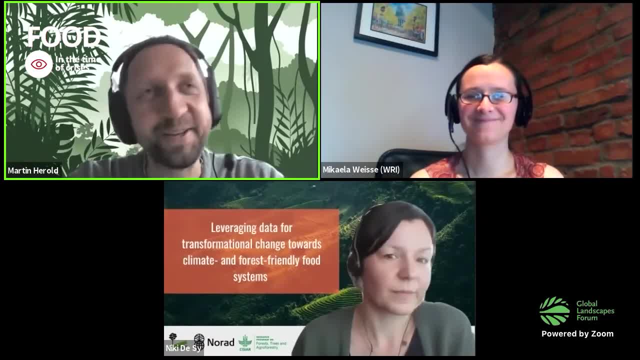 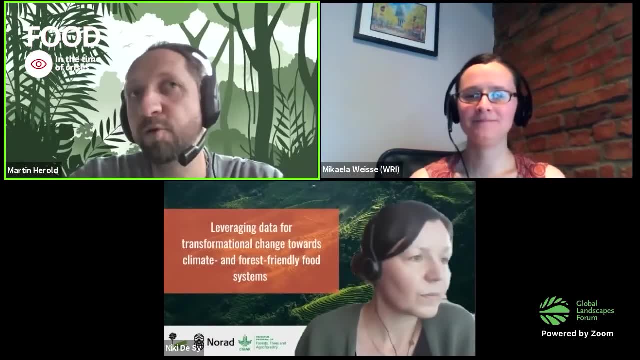 Yeah, thank you and welcome everybody on the on the session, also from my side. Yeah, so technology and these technologies, these global data sources, are improving, and they are improving quite a bit. Our whole research team is working on that, trying to. 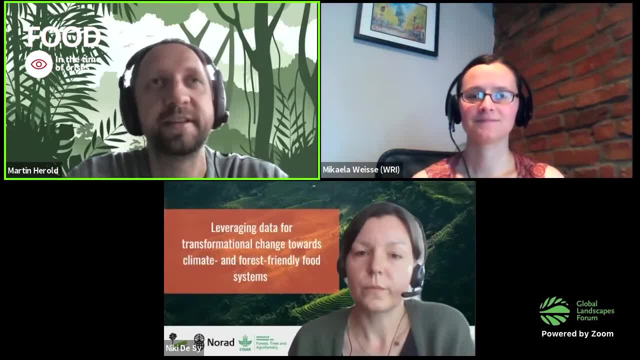 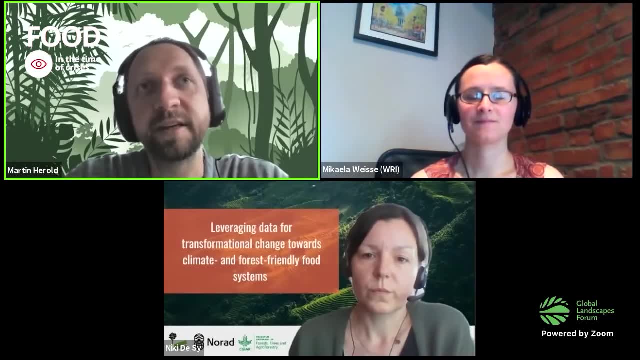 make data more detailed, more accurate and more accessible for these kind of purposes. For example, the example of Nigeria. we know, particularly in Africa, that these near real time systems or these fast delivery of, let's say, land change information is really there's not a lot of good examples on that. 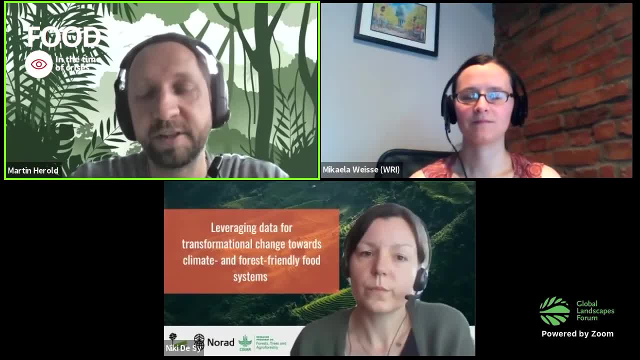 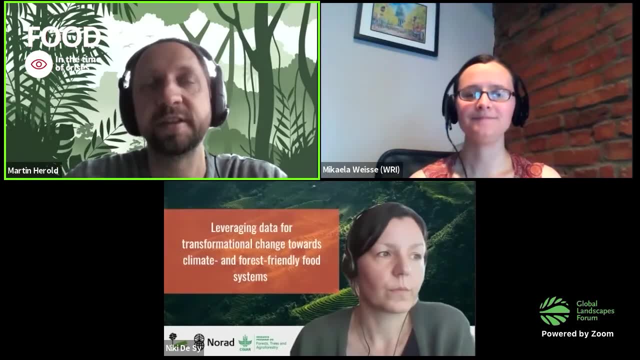 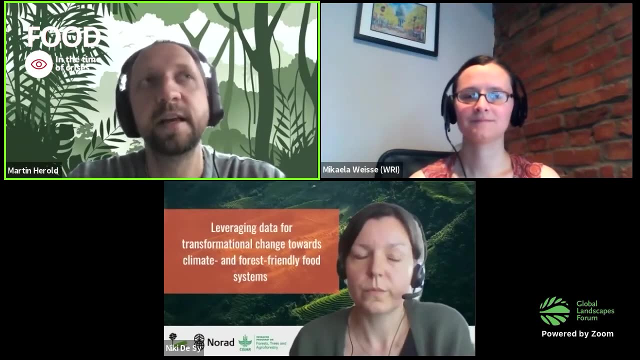 And, for example, there's a lot of focus now, particularly in Central Africa in particular, but also in other parts of Africa, to really make these global data assets more useful for their purposes, For Nigeria in particular. it's maybe good to mention also that we want to get into some of the technicalities. 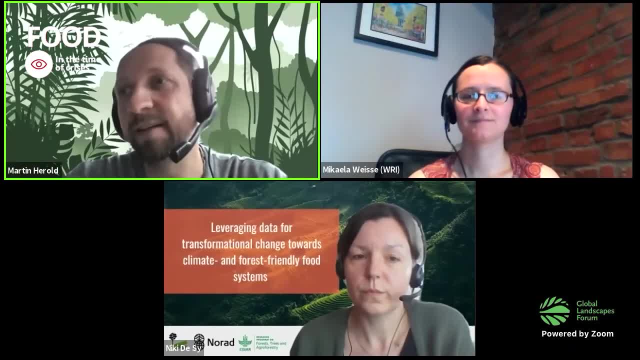 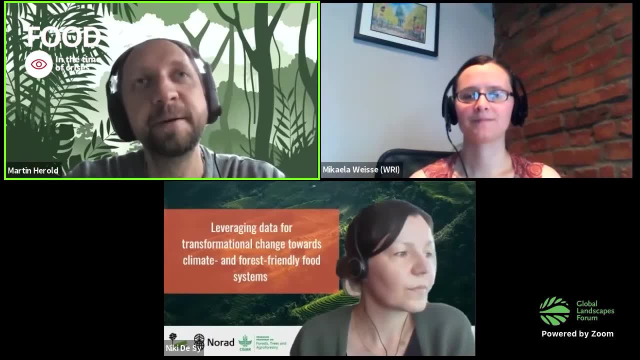 It is now, from a data side, easier to monitor changes in evergreen forests or these kind of evergreen kind of tropical forests, If you move into more dry forests but there's seasonality and you have leaf on, leaf off conditions that 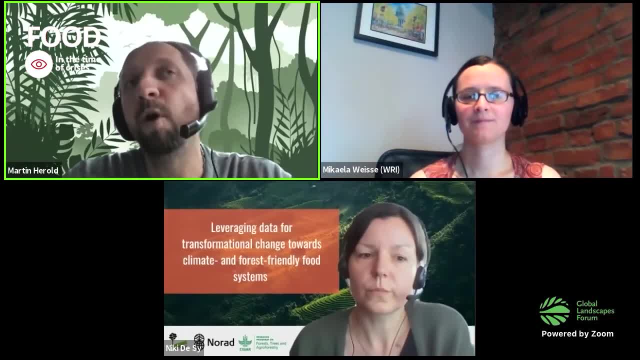 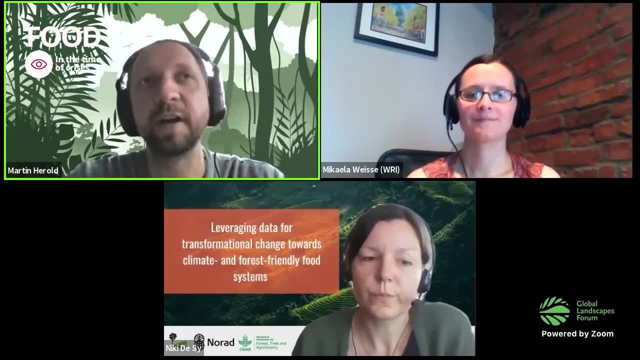 of course, make things a bit more complicated and you get usually lower quality data out of that. But that's also. people are working on that, So we also expect improvements there. but just to give you a bit of an idea that it's, for example, easier to do that in the in the Democratic Republic of Congo. 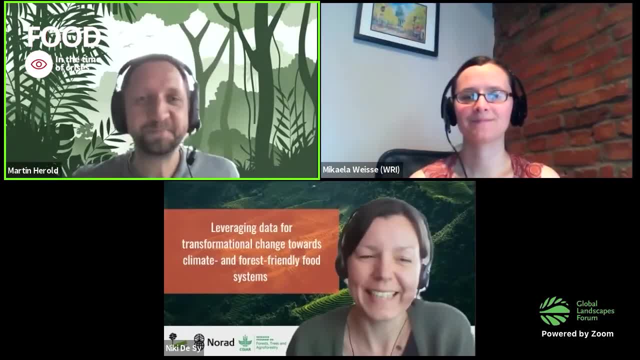 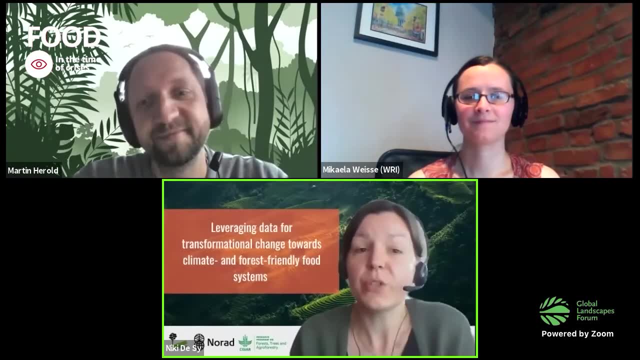 than it is, for example, in Nigeria at the moment. Oh, thanks a lot. I don't see more questions popping up at the moment, so I suggest we just move on to the next topic, and I'm sure there will be more questions for you also. 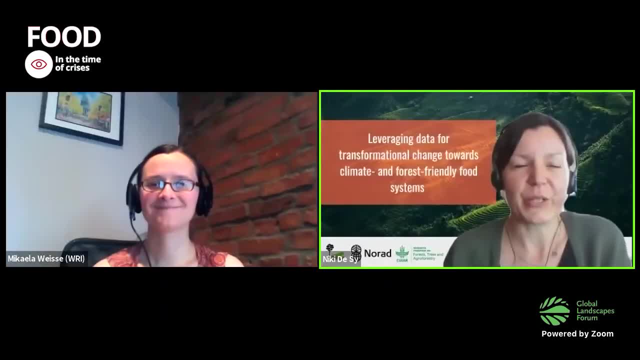 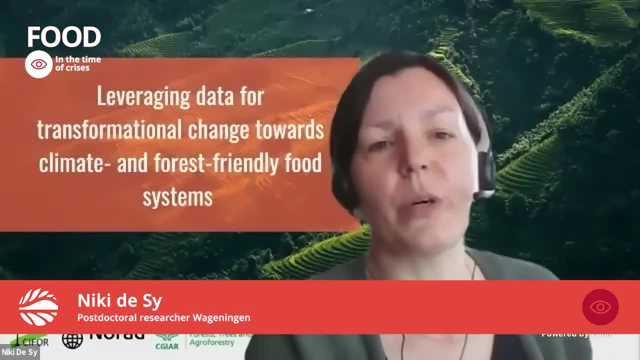 in the panel discussion, but thank you for your contribution. So if you could, please turn off your video. thank you, And then the next topic we're going to. we are going to talk about Indonesia, And Indonesia has committed under the Paris agreement to reduce its greenhouse. 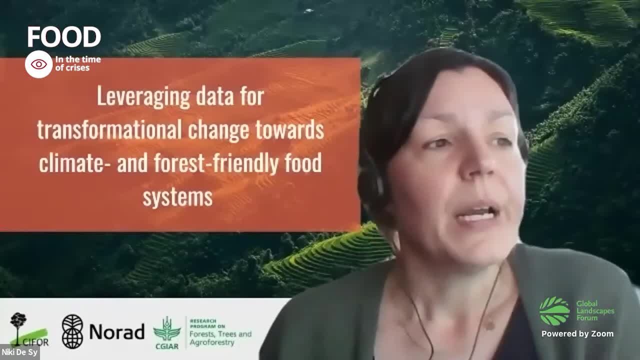 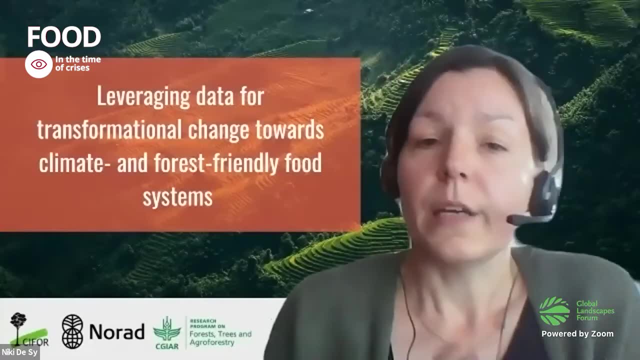 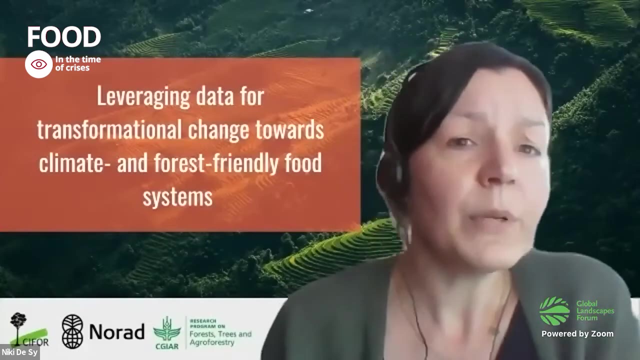 gas emissions compared to a business as usual scenario. And of course for this you need a benchmark for seeing this progress toward your goal. And Indonesia has developed already a few years ago a forest reference emission level as this benchmark, But then they've recently decided to improve their emissions at their reference. 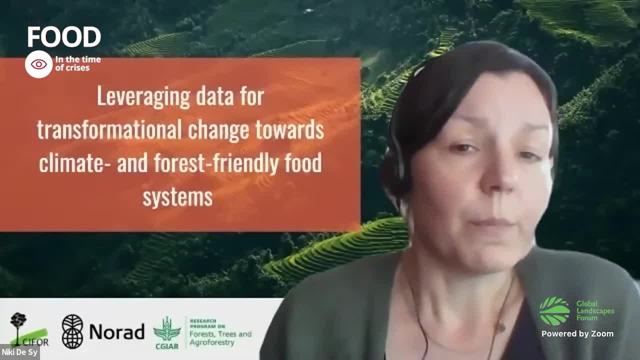 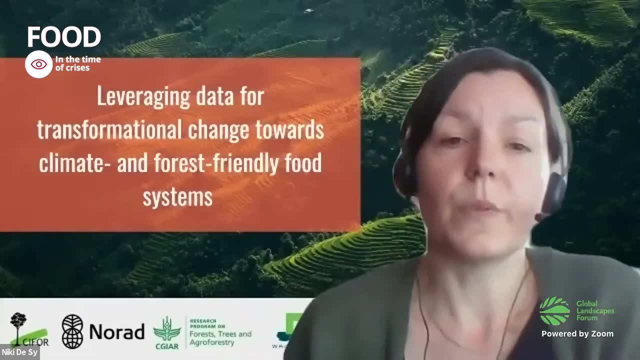 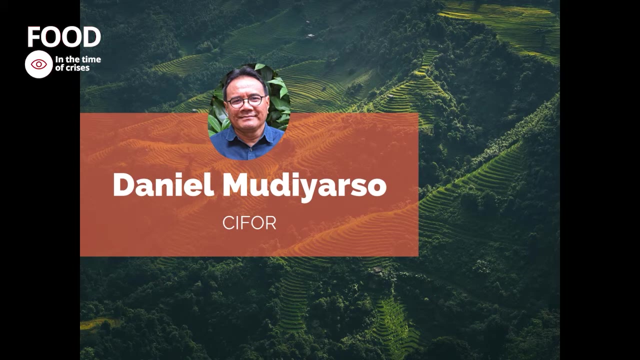 level, also drawing on scientific data and methods, for example from the IPCC wetland supplements, And we're going to hear a little bit more about that in the next video, So please start the next video. Hello, my name is Daniel Mouriarzon. 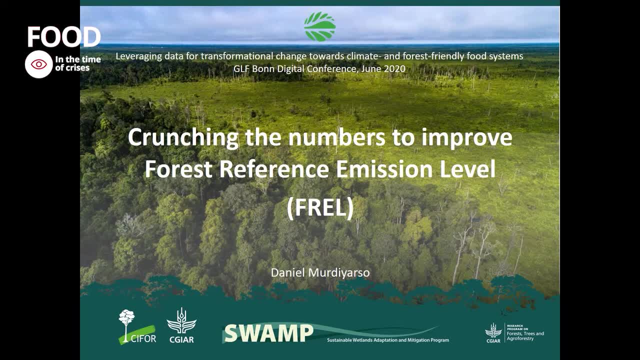 I'm with the Center for International Forestry Research, C4, and I'm speaking on behalf of my large group in the Sustainable Wetland Adaptation and Mitigation Program called SWAMP. When I was asked to speak on this session, leveraging data for transformational change, I thought it's very appropriate. 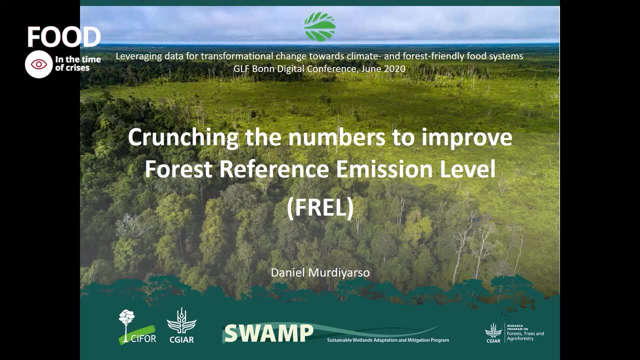 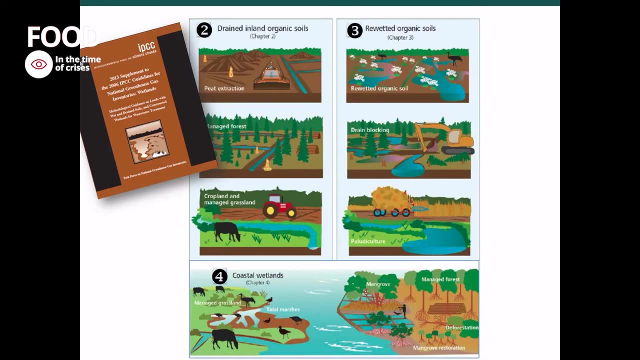 title for me to share with you how to crunch the number when we are trying to work in the field and use that data to help improve the forest reference emission level. F-REL, C4, and particularly SWAMP team, were heavily involved in the development. 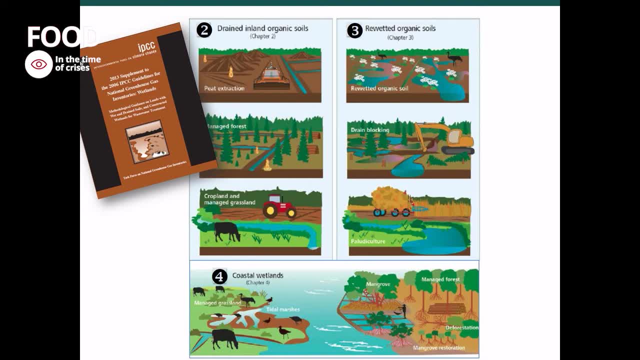 of this 2013 supplement to the 2006 IPCC guideline, which was specially designed for wetland. I just want to bring your attention to chapter two, three and four of the guidelines which are dealing with wetland, namely peatland and mangrove. 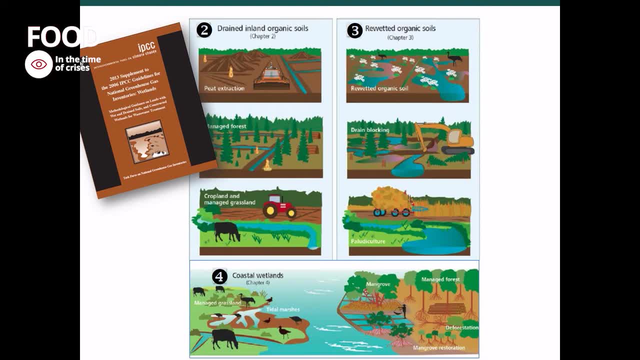 In chapter two we were talking about drain organic soil, which is basically dealing with the development and also degradation of peatland, And chapter three dealing with rewetting of organic soil, which is basically related to the restoration and conservation of peatland. 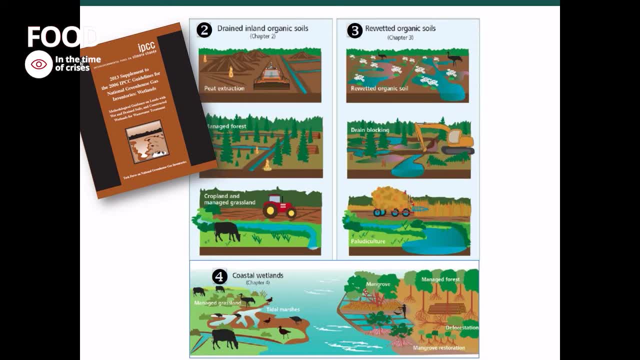 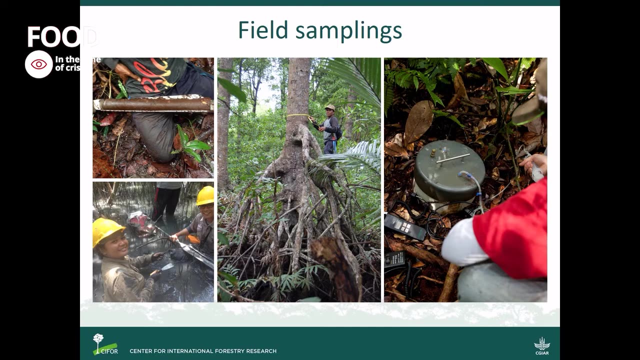 And in chapter four, it's all about mangrove, which is very much affected by also land development for aquaculture. Since the guideline was released in 2014,, our scientific journey began with field work to collect data By which we derive emission factor from peatland and mangrove. 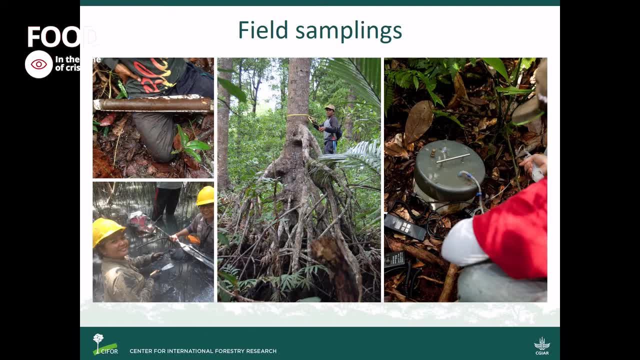 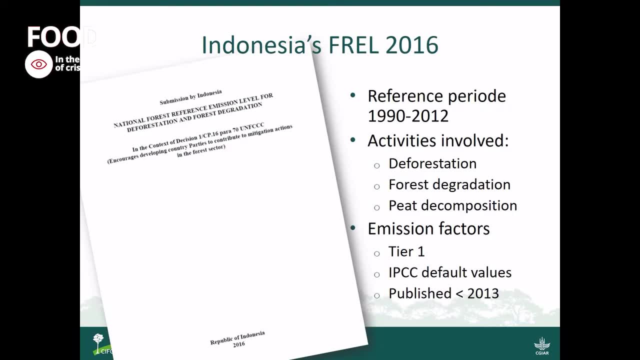 What we did was assessing carbon stock from various compartments and also measuring in-house gas fluxes from the ecosystem. Now let's shift our journey to the policy process, And let me take an example of Indonesian F-REL, which was submitted in 2016.. 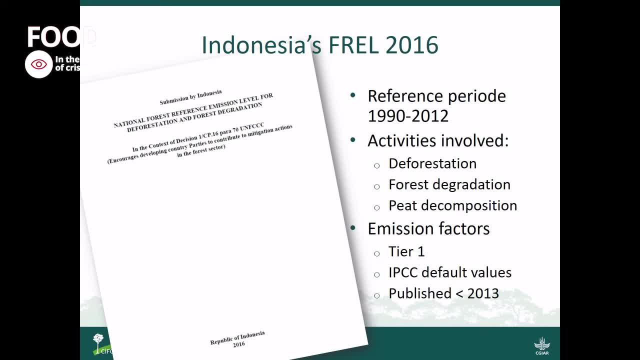 The document used the reference period of 1990 to 2012.. And the activities involved in this document were deforestation, forest degradation and peat decomposition. And the emission factor adopted in this document were Tier 1, which was the IPCC default values. 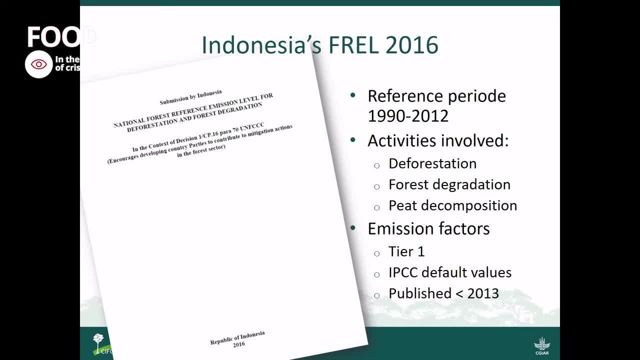 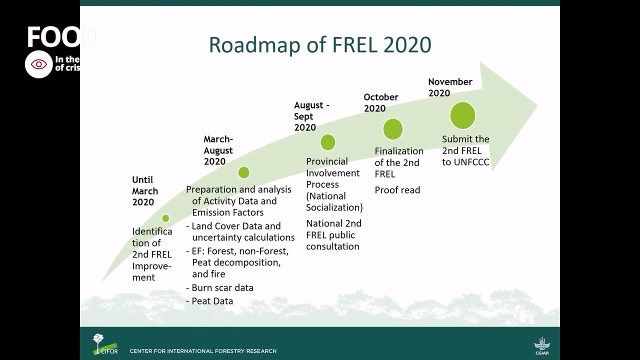 And these numbers were from the literature which was published before 2013.. After having been used for almost five years, the F-REL 2016 needs to be improved, And this is the roadmap of the improvement towards F-REL 2020.. 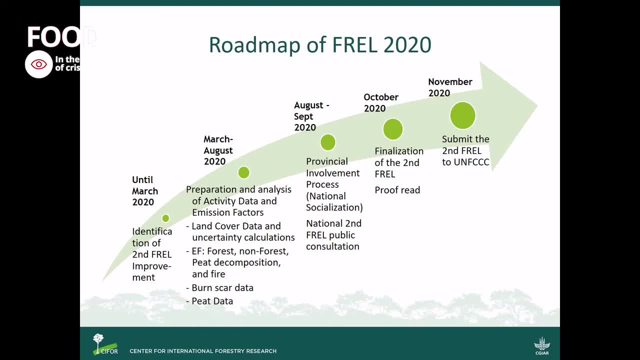 Now is the month of June. The government is preparing a number of things, including analysis of activity data and emission factors. These are new activity data and new emission factors. Those include emission factor from forests and non-forests. peat decomposition. 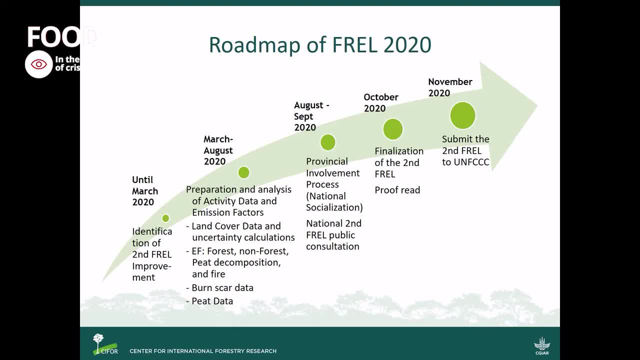 and then peat fire and also new activities in mangrove and wetland. So the improvement will cover a lot of ground and needs a lot of support scientifically Towards the end of this year. there will be several processes, including consultation at national and subnational level. 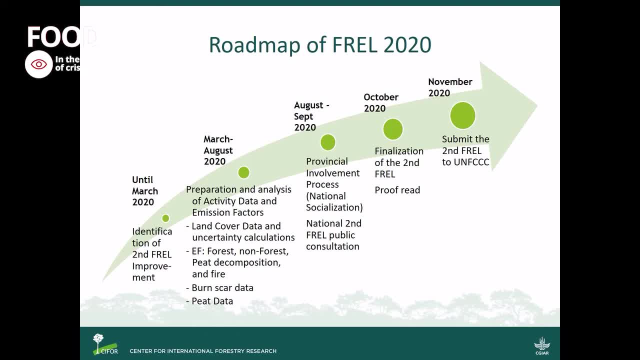 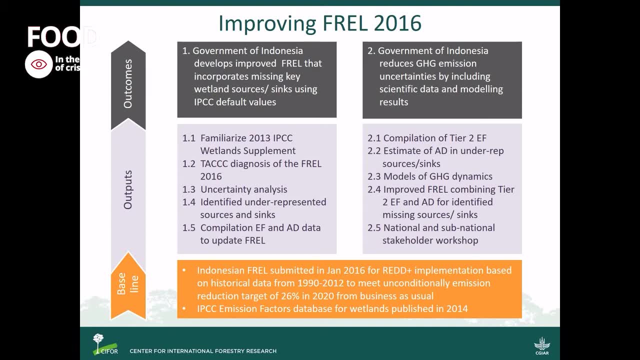 before the new F-REL will be submitted Sometime in November this year, Since wetlands are central in the improvement of F-REL 2016,. scientifically, we can provide a number of supports, including the familiarization of the 2013 IPCC wetland supplement. 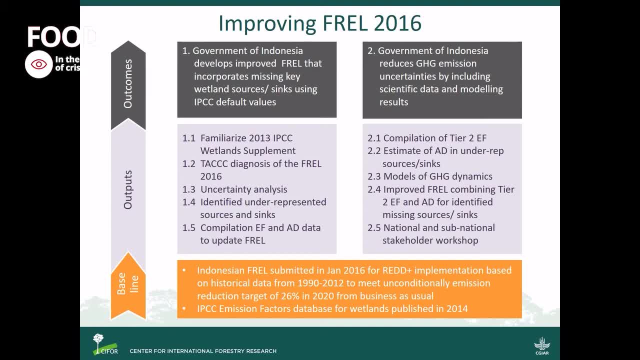 the diagnosis of the current F-REL in terms of its transparency, accuracy, consistency, compliance and performance. We can also provide a number of supports, including the availability and completeness and analysis of the uncertainties of emission factor and activity data, Also identifying the underrepresented sources and things. 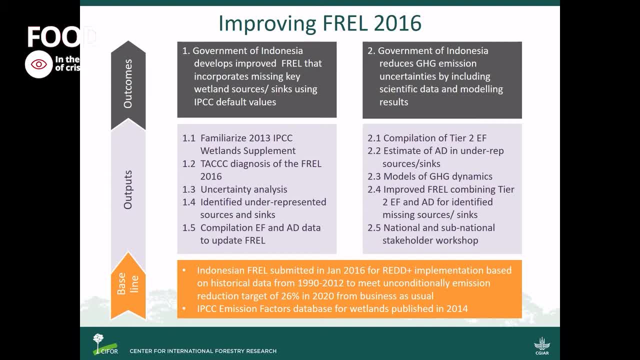 And more importantly, is providing the new emission factor and activity data. So with those in place, the government will be able to improve F-REL. by incorporating those new numbers For further improvement, we can provide higher tiers, more accurate activity data. 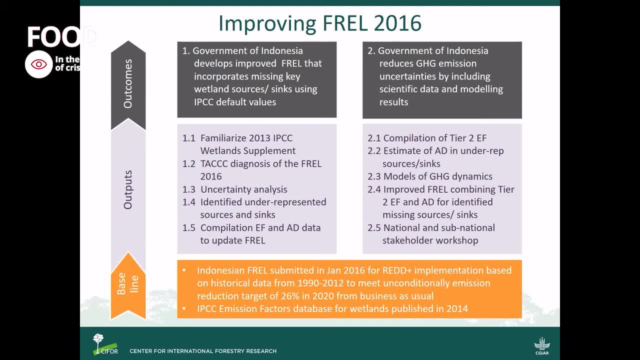 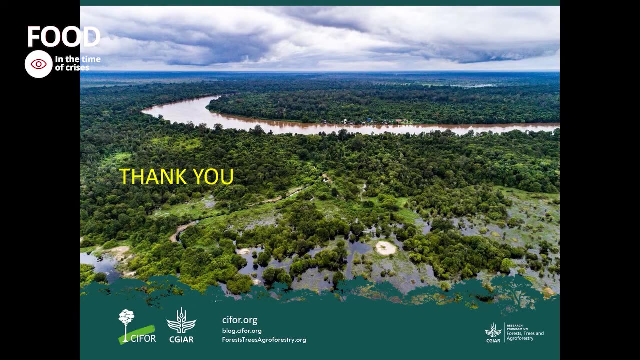 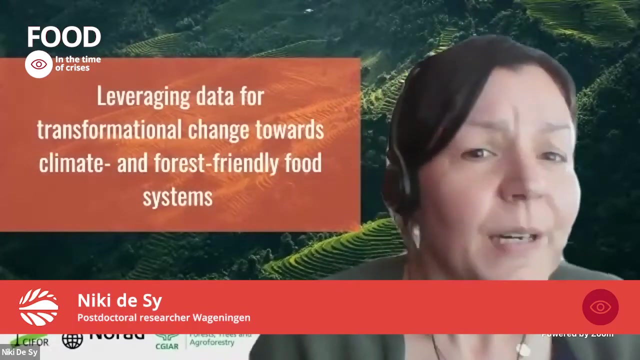 modeling numbers through greenhouse gas dynamic models. So with those things, the government will further reduce the uncertainties of greenhouse gas emission. So this is the end of our journey. Thank you for your attention. I'm happy to entertain any questions. Well, thank you, Daniel, for this. 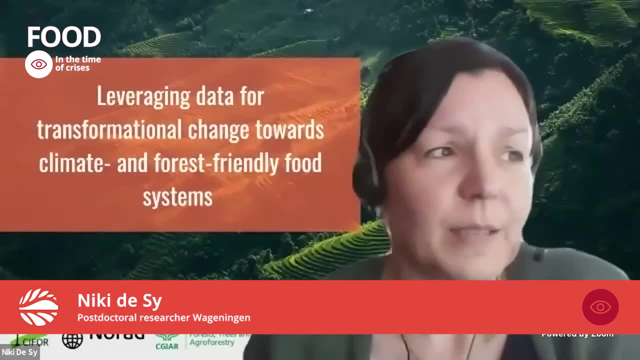 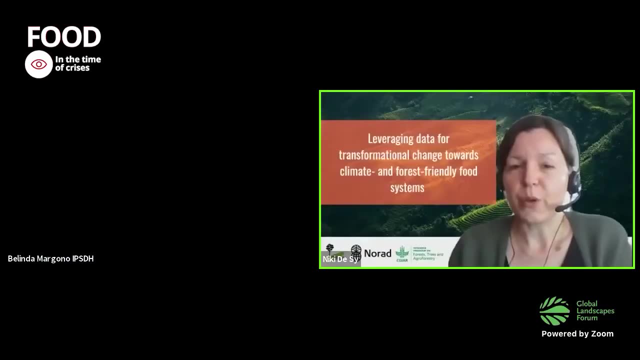 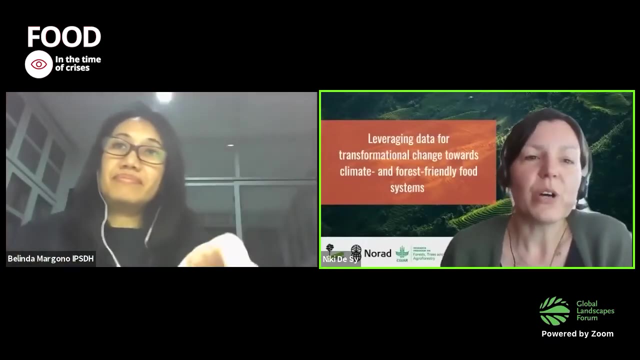 Introducing us a little bit to the topic, and I want to invite Belinda Margono now to join me here in the Zoom session. So if you could put on your video, Hi, Belinda. welcome in this session. Belinda Margono is from the Indonesian Ministry of Environment and Forestry. 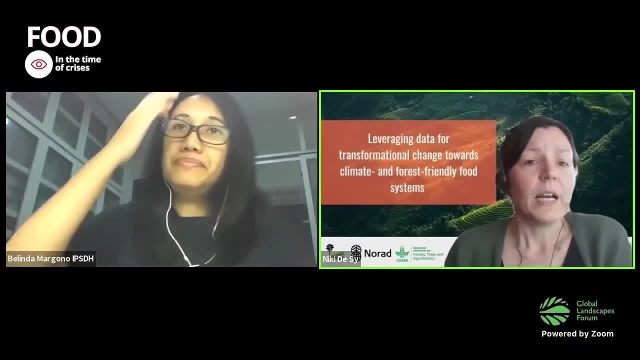 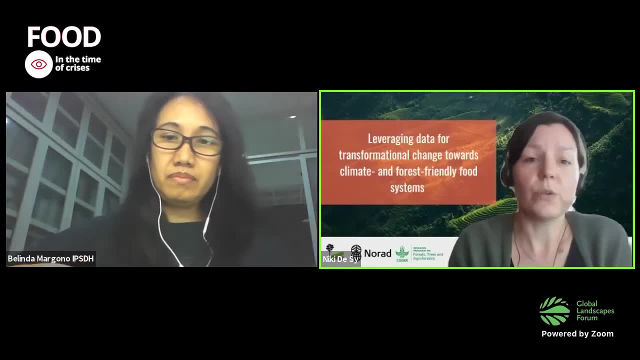 Who is also involved in the improvement of the F-REL. So she has also provided some background information, some additional slides that we will share in the chat right now If you also want to look at that in the meantime or afterwards. So, Belinda, can you briefly introduce yourself and your role in this? 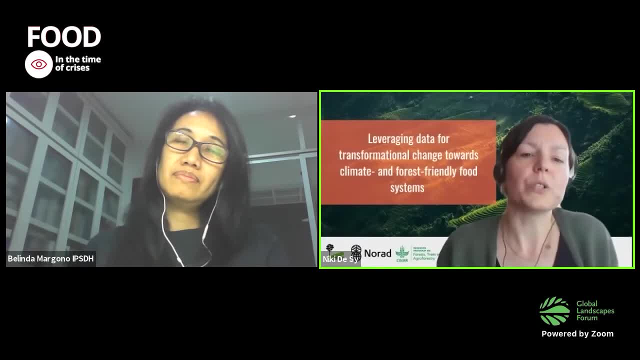 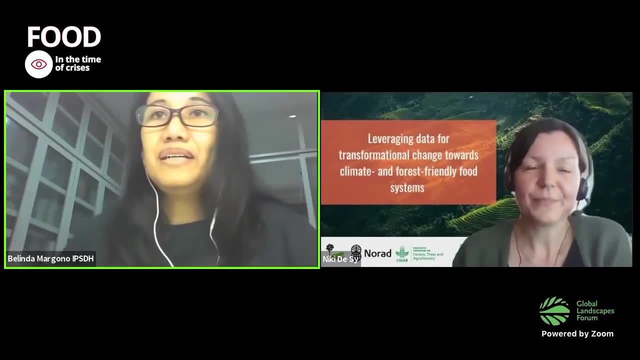 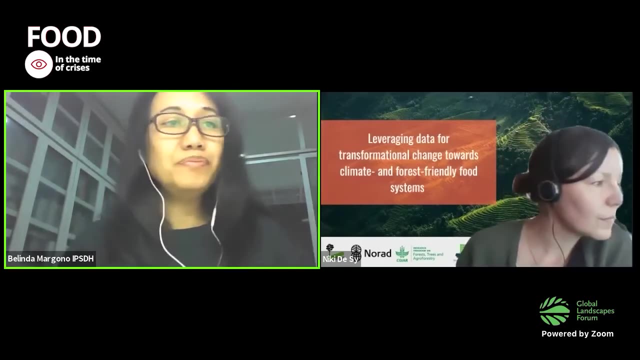 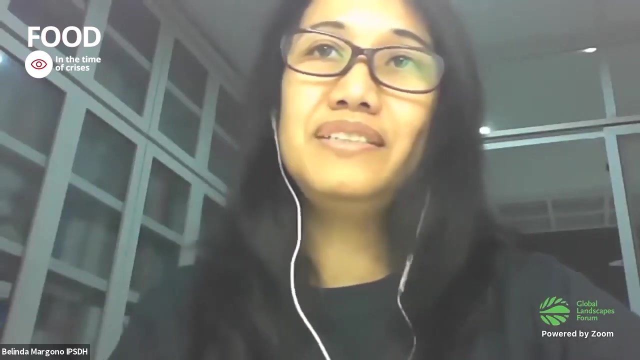 improvement and tell me a little bit about why is it so important to update this forest reference emission level. OK, good evening everyone. My name is Belinda Margono. I'm in charge for providing information for data activity in the Ministry of Environment and Forestry. 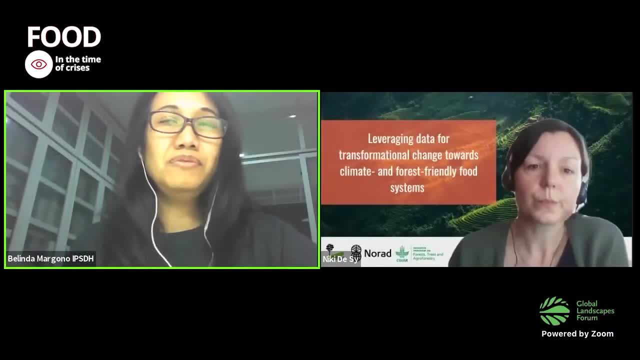 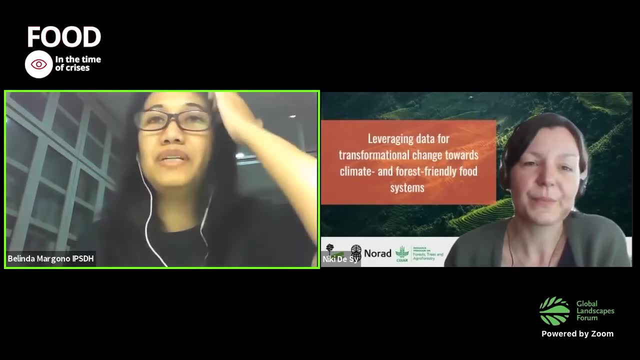 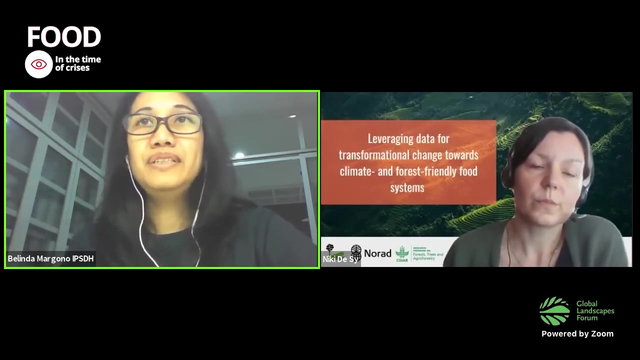 dealing with the remote sensing data set and also the field data measurement. So if the question is like why this is very important, We do have a regulation that actually, the first time we established our first F-REL it was in 2015,- but it takes about a year for just to review the process. 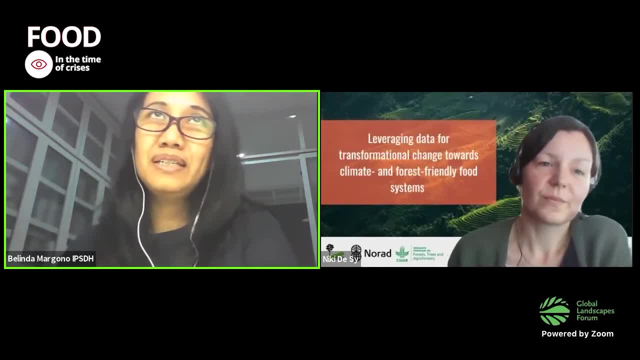 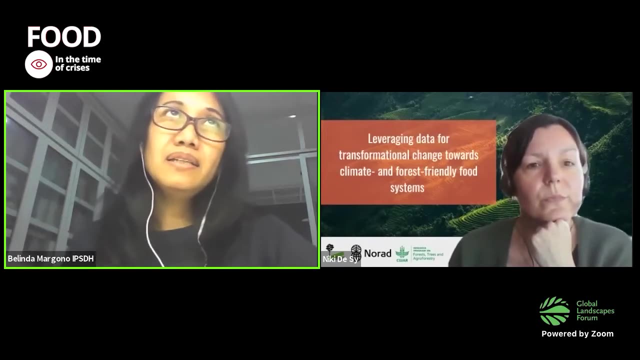 And, finally, we've done the review process at the end of 2016.. So that was the first, our first F-REL. They cover a lot of things. I think Daniel mentioned about some of them, but there are still a lot of. 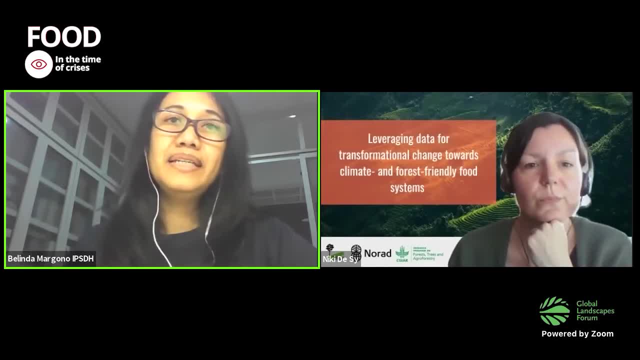 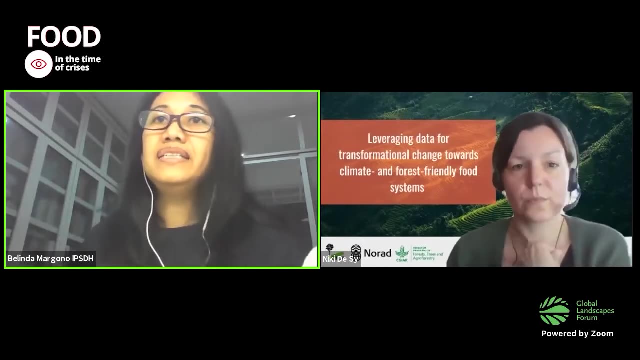 I would say a missing thing, because during that time the data was not available or the data quality was not in a good condition to use. So, based on our regulation, the F-REL have like time limitation, like not a limitation, but we try to make updated every five years. 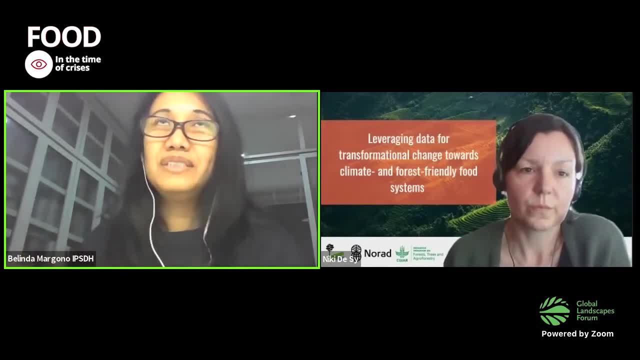 Since it was established in 2000,. I mean in 2016.. So actually by 2021, we should have the new F-REL at least, because that is the F-REL that updated based on the current situation. So that is one of the reasons why we have to update our F-REL. 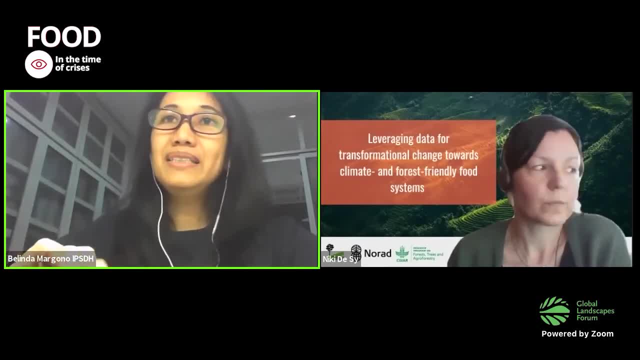 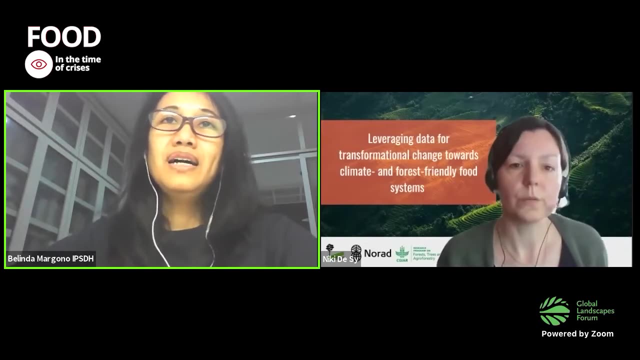 And why we also focus on the wetland. but wetland here is including the peat and also the mangrove, because in our first F-REL we haven't yet really include the mangrove. Not so much information on the mangrove is not in the activity data. 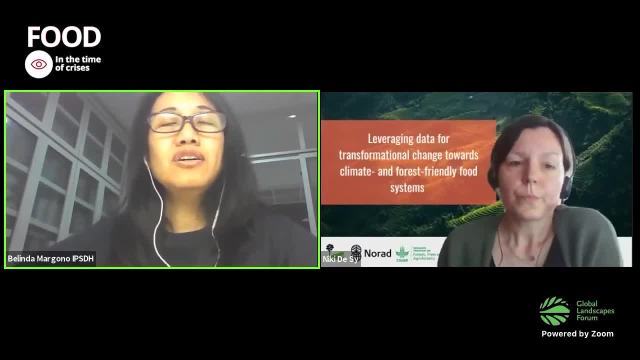 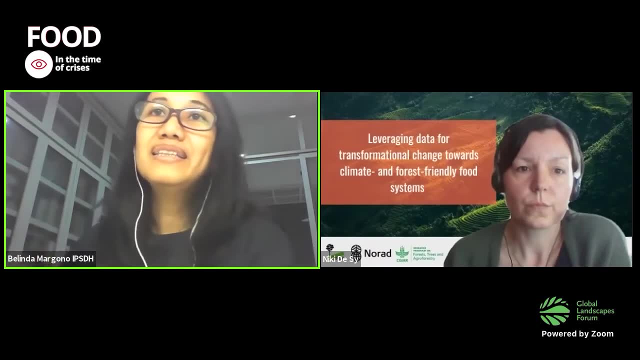 but more about emission factor. So there are a lot of biomass information on the ground, but we cannot make it at the national level to provide the emission factor for strata for the mangrove forest. So that's also the reason why we don't use the national data. 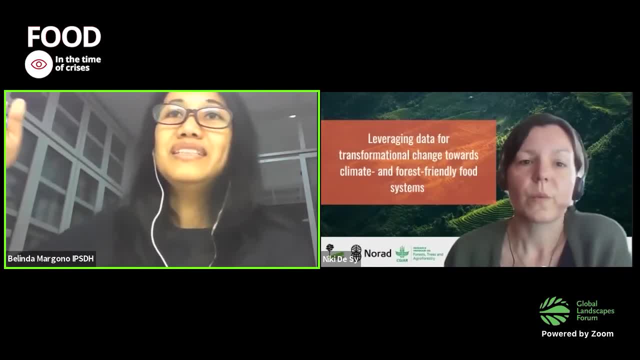 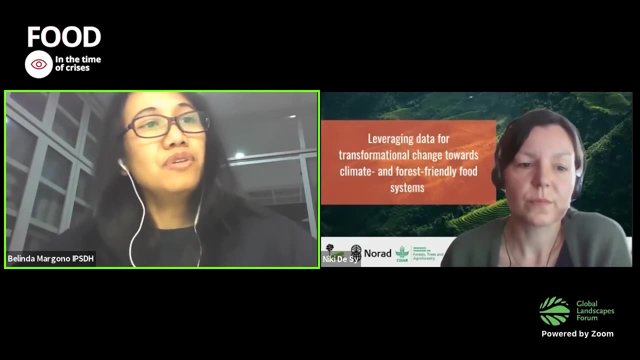 but we refer for some research. So that is the reason why we need to improve that, And also there are some- I mean a lot- of information need to be added on the peatland itself, because so far what we have now is just the peat decomposition. 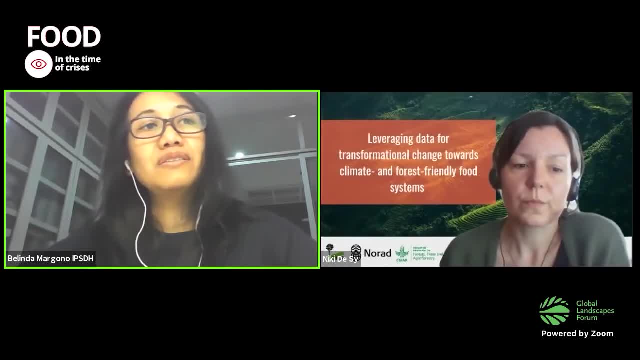 And that is also based only on the research- the emission factor and so on- and need to be updated based on the current research and also based on the current data set. So that is some of the reason why we have to update it, But it's been five years. 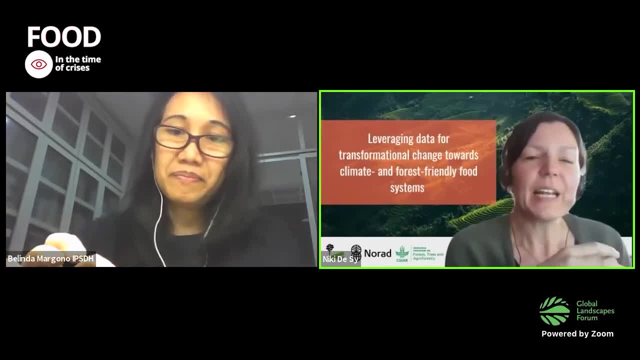 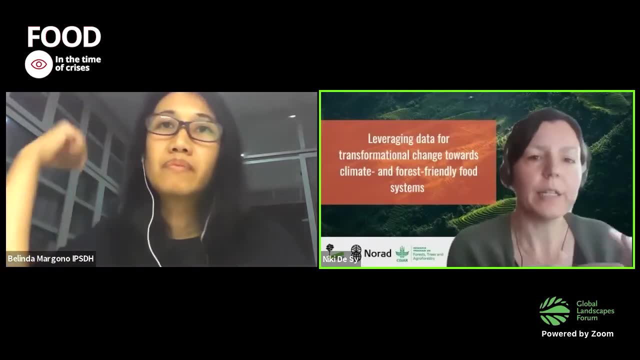 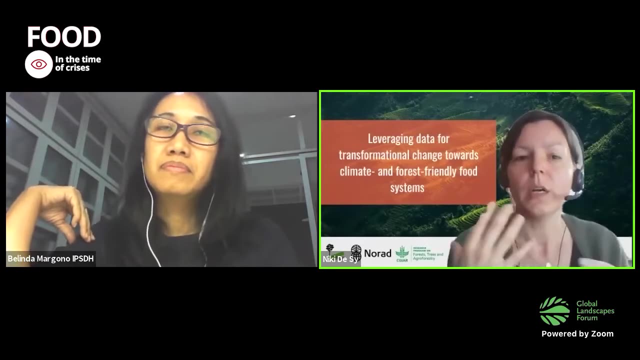 We have to have a new one. Oh, very interesting, And I was wondering: do you also expect that it will have an influence on sort of the policy level, like that, that that this will also help to set certain goals or to take certain certain actions, or you think it will also help in that? 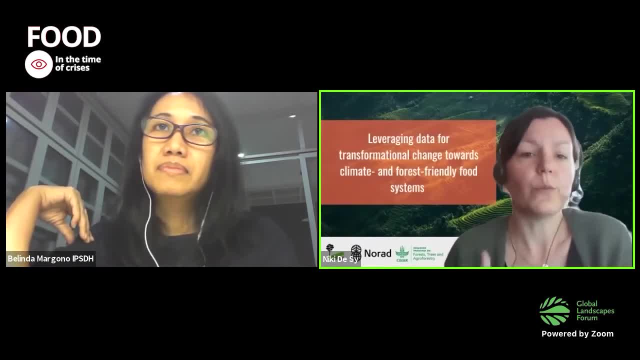 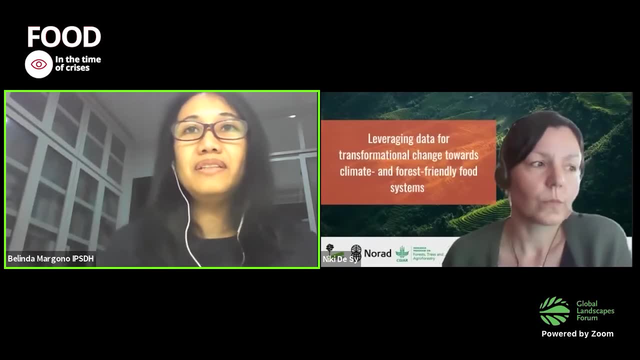 respect to to have more information about that for the wetlands, for example. Yes, it is. It is very true that actually the government itself actually set a lot of regulation and try to get more information on, on the peat, For instance, following our first review on our first row. 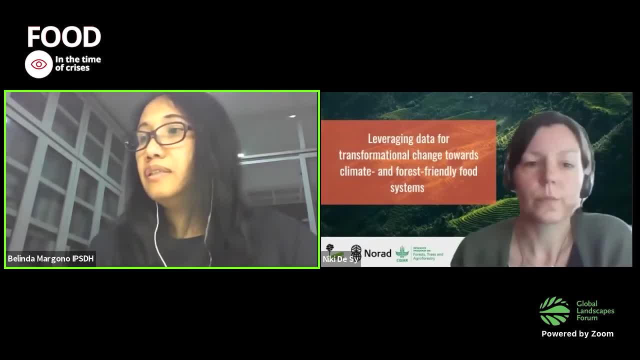 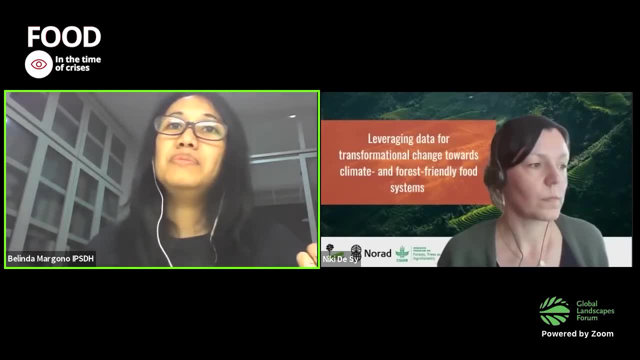 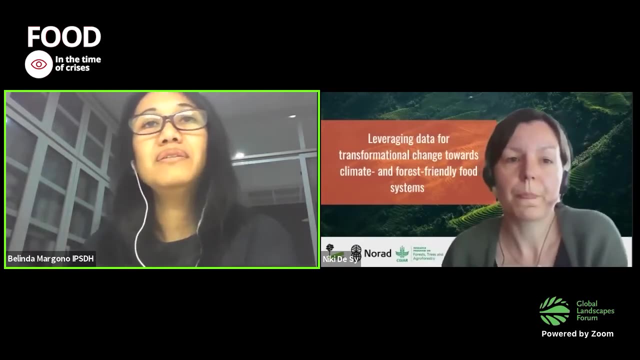 it was also a need that actually we need to have the most: the information regarding the moisture content on the peatland, the information about the groundwater level and so on. We haven't yet have the data during that period, But nowadays I think we improve a lot of ground. 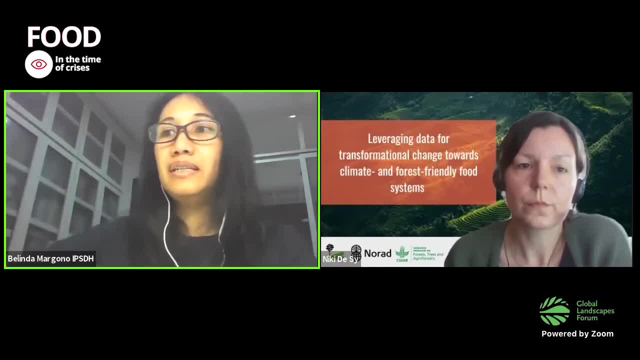 water level. So we have several plots spread out all over the country that actually we hope that at some point we can use that as the improvement on the peatland itself, because you know the peat is actually- it's relatively very huge compared to the size of the country. 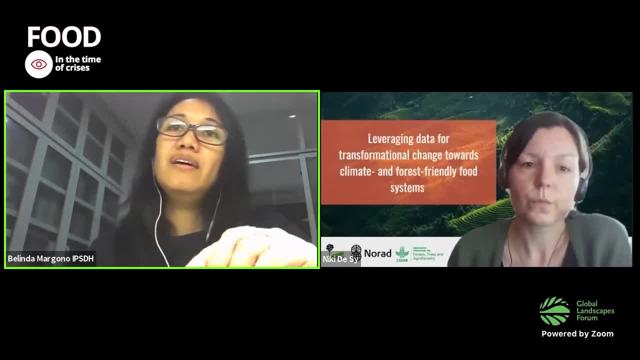 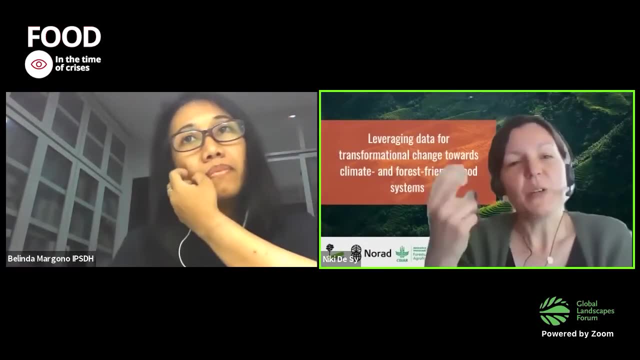 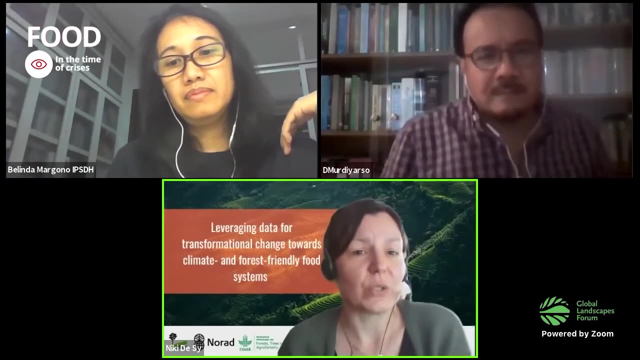 So we really want to pay a lot of attention on on the peatland, Not only the mangrove, but both. OK, thanks. I also want to invite Danielle to join us here, because I have a question that you might both have some reflections on. 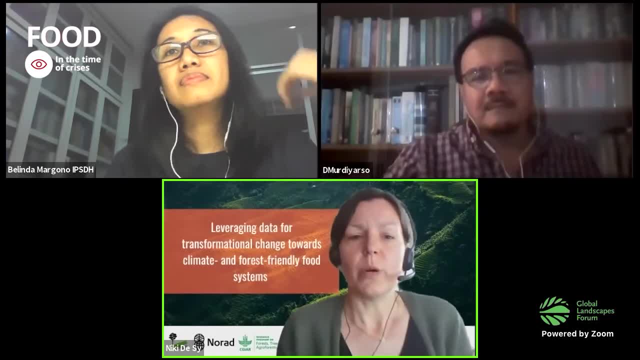 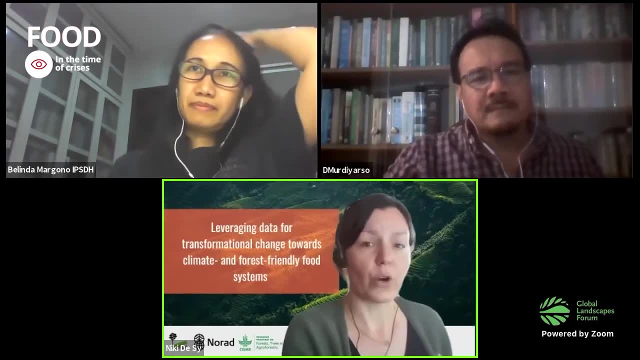 So so what I hear also from you and what I know from Danielle's work: there has been a lot of fieldwork. You have the new IPCC, You have the wetland supplement to to draw from the guidelines. There's a lot of national and global data sets that might be interesting. 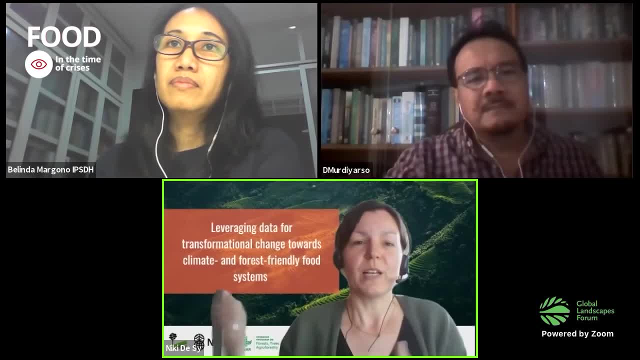 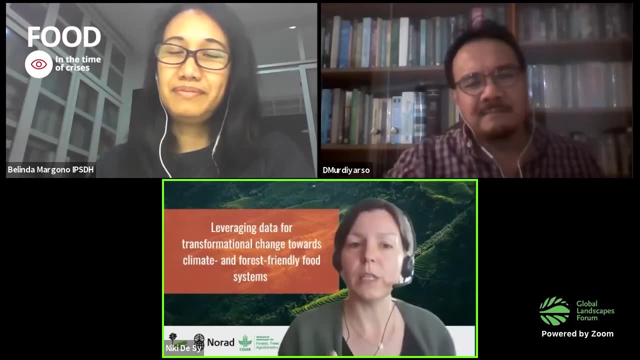 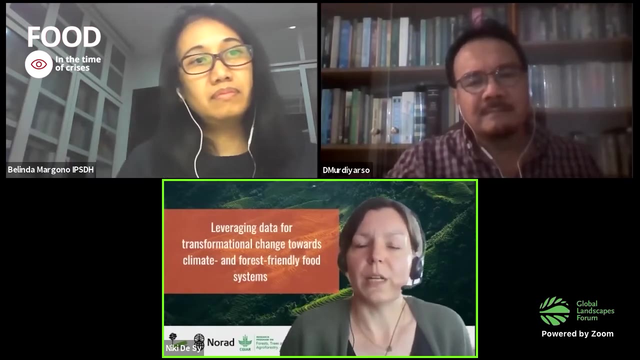 And of course, you're also both scientists and you're working towards also in this policy context. So can you share with me some of the lessons you've learned of making that a success, of really making sure that the scientific data and methods really you know that you can really use them to to improve something? 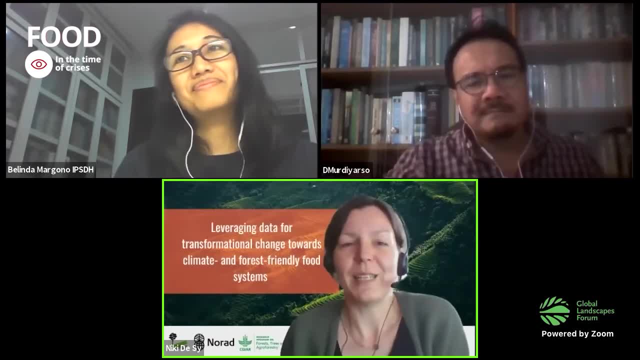 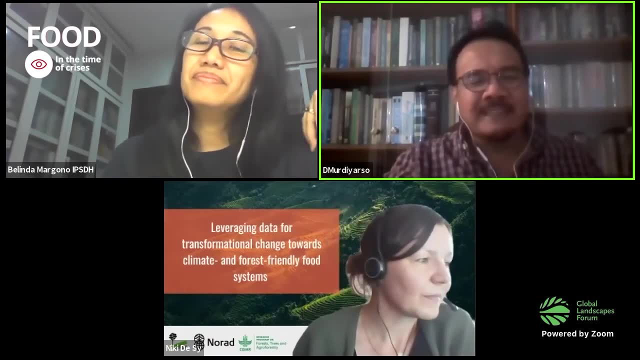 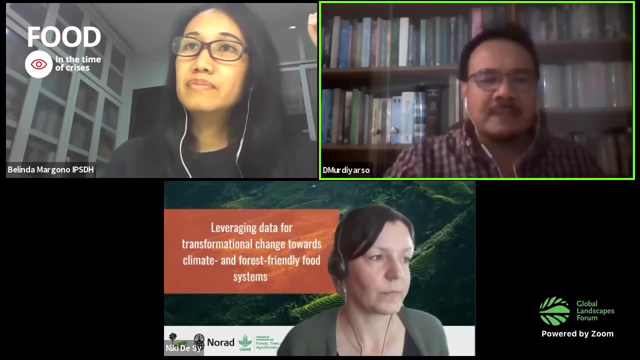 like the FREL. So maybe Danielle can start, And I would also like to hear from Belinda. What are your thoughts afterwards? Yeah, well, welcome everybody. In the context of data, I think we are in a very good position to say about. 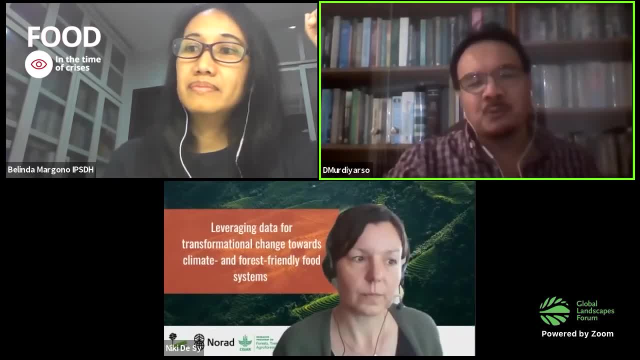 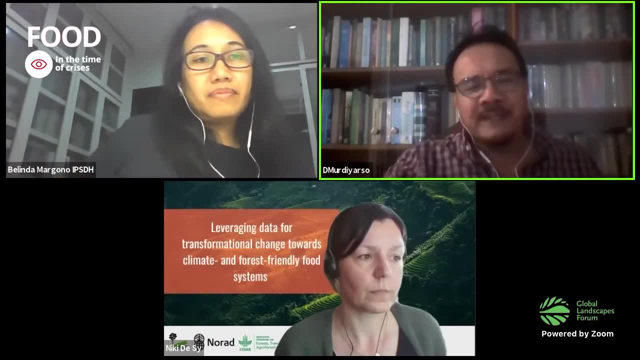 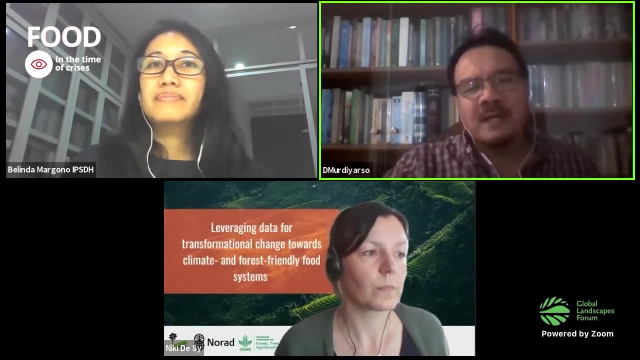 whether or not we are trusting the data or to what extent we trust the data. So the issue of certainty, or uncertainty, is very crucial here. So I did mention very briefly about uncertainty analysis. So if you know how uncertain it was when FREL 2016 was submitted, 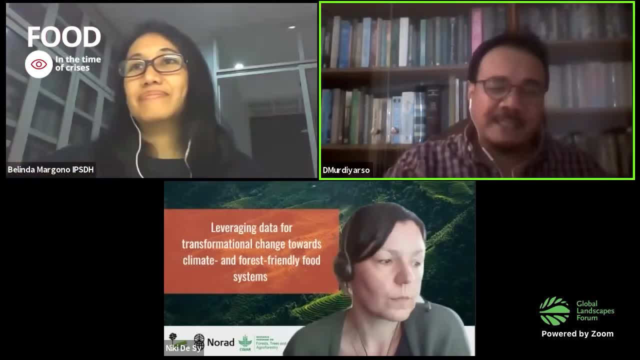 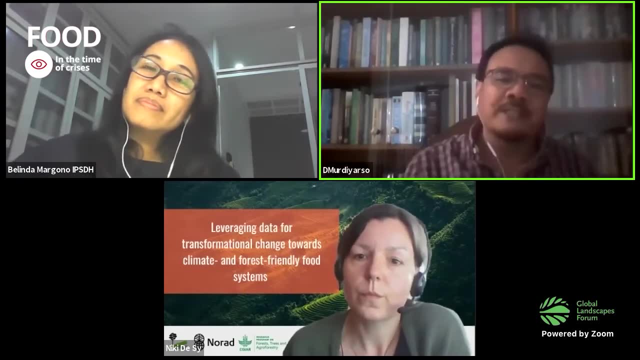 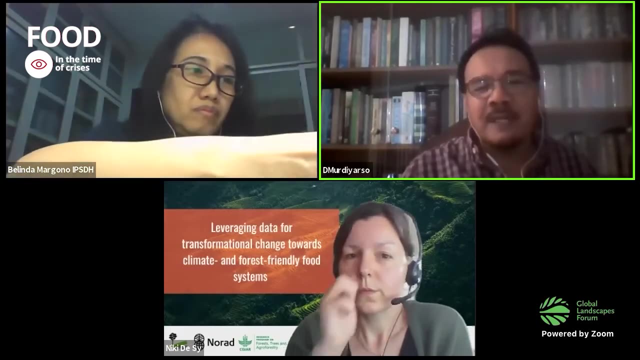 we tried to analyze the uncertainty so that, with this result, we would like to help how to improve the uncertainties in terms of reducing the uncertainties. So, with the help of Norway, we tried to reduce this. So, at the end of the day, the FREL will have. 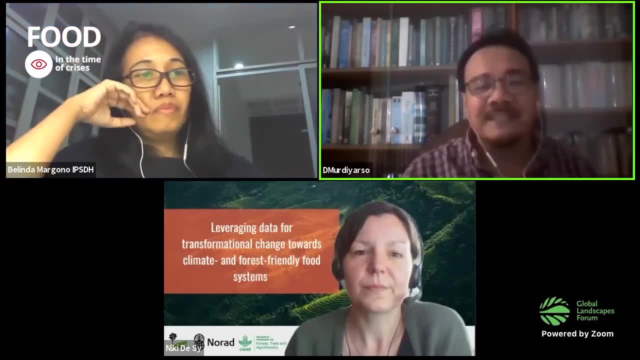 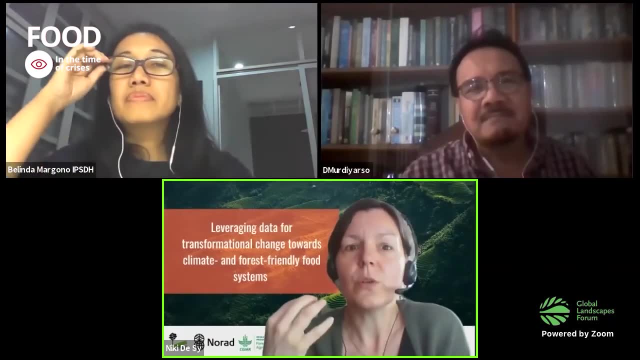 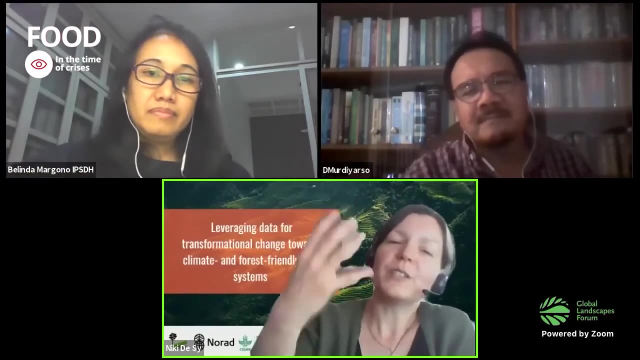 a lower uncertainty in both emission factor as well as activity data. And can you elaborate a little bit why it's so important to reduce uncertainty? Because also uncertainty means something very specific to scientists or statisticians, But so can you also for the non-scientists or the practitioners, explain a little bit? 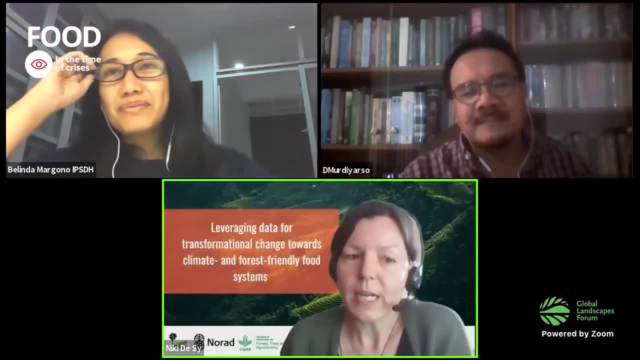 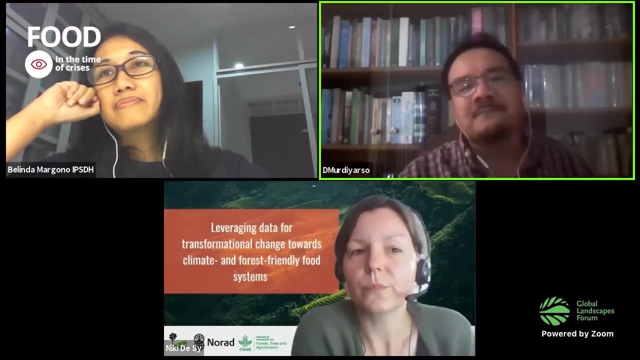 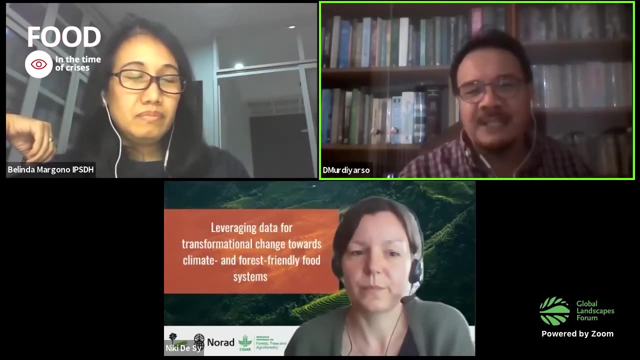 sort of. so what is this uncertainty and why is it so important to tackle this? Well, it's related to the quality of your product, the quality of your commodity. in this case is carbon currency, So the buyer will have to see how uncertain it is. 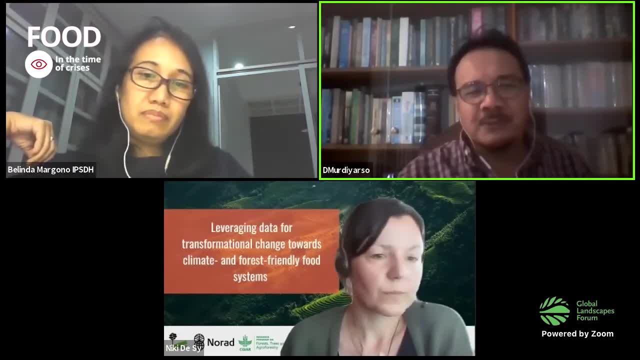 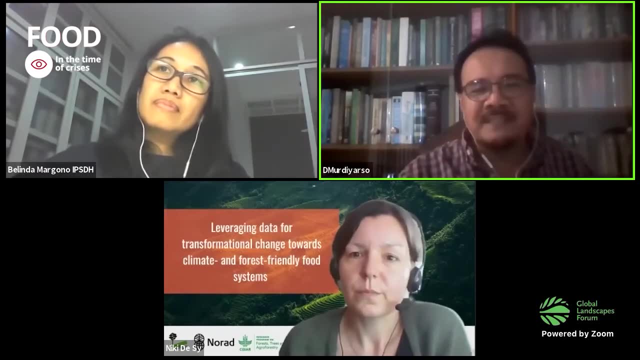 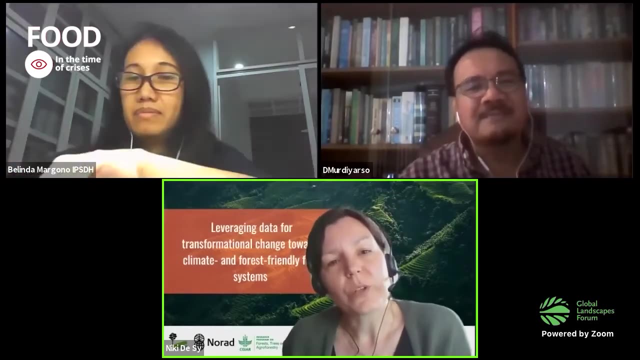 So how can you rely on this? So it will be related to the price of the commodity And, I believe, the buyer on the result of this payment. this uncertainty is very crucial. Okay, Thank you. So, Belinda, from your side, what are some of the lessons you've? 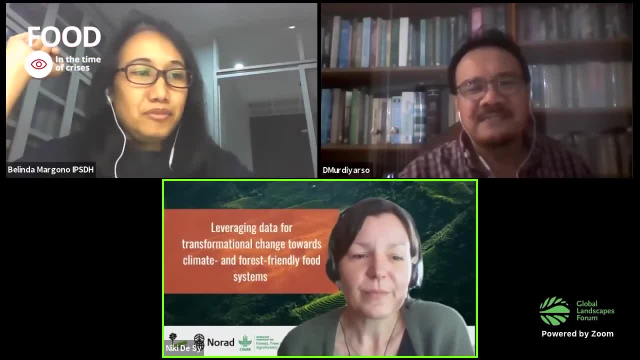 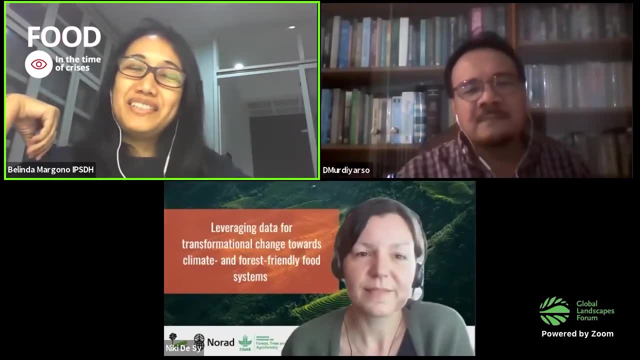 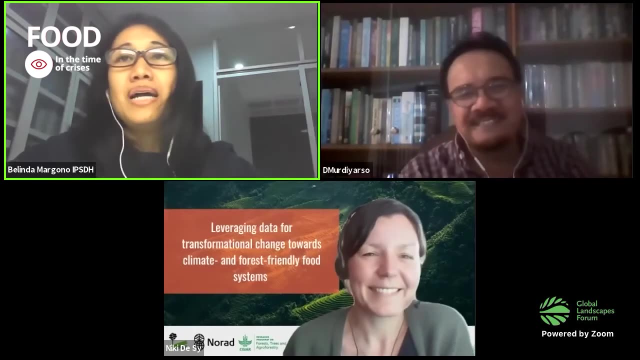 learned from being in the middle of that process? First of all, I would like to start that the process is actually very interesting. I think I feel so lucky that I did follow all the process from beginning till now. But I think the first important thing we have learned 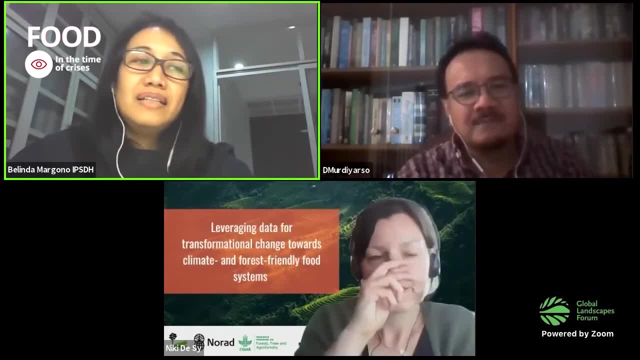 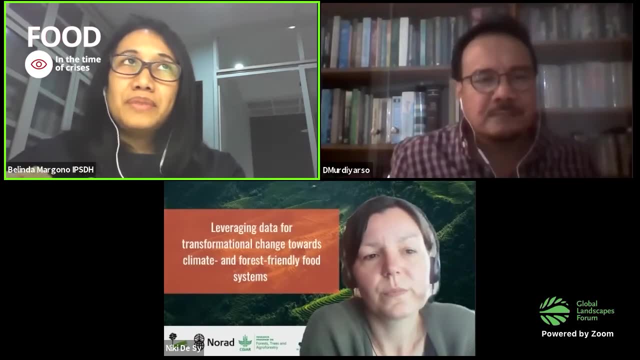 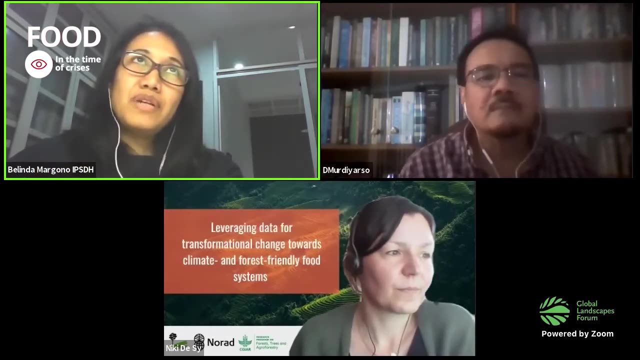 is that the process of establishing the FREL is a stepwise approach. I know, we all know that, based on the UNFCCC information and so on, it seems like the establishment of the FREL or any other information related to that, it's a stepwise approach. 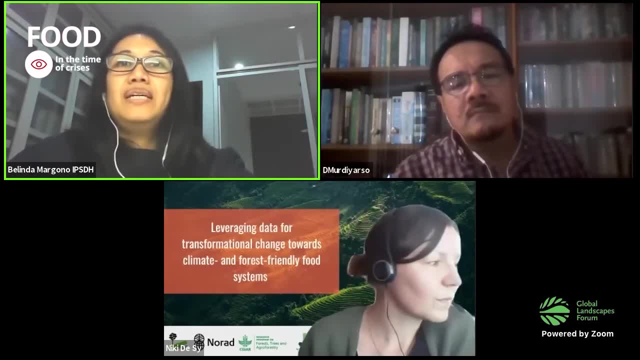 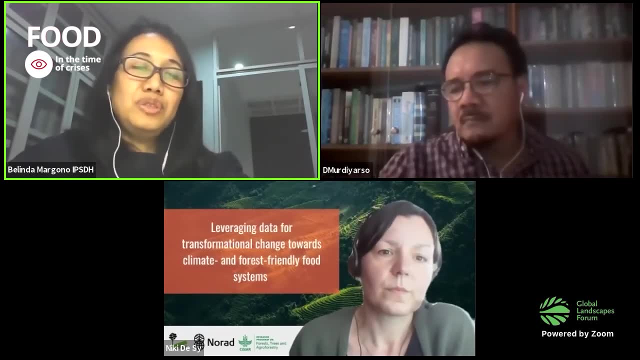 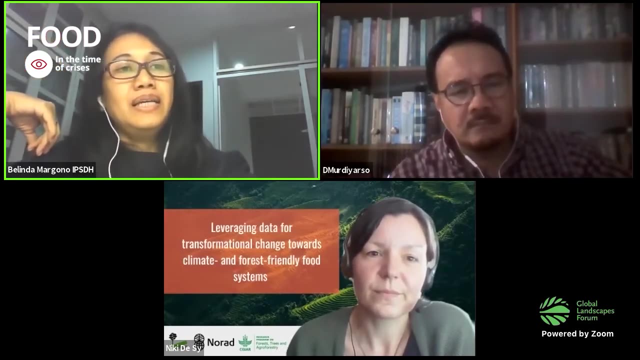 So we don't have the perfect one at the first time. We can learn and try to improve all the missing things or we try to improve, I think in the case of Daniel. he mentioned about the quality of the data And in my views I think on the first. 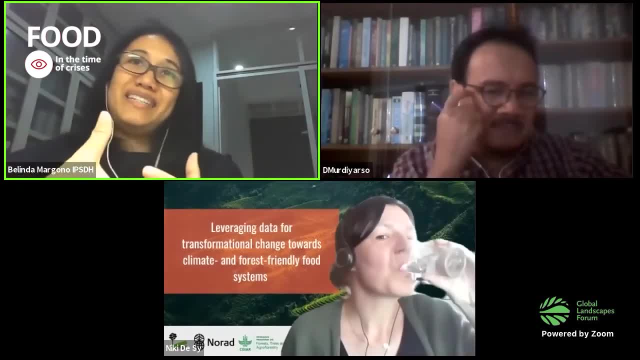 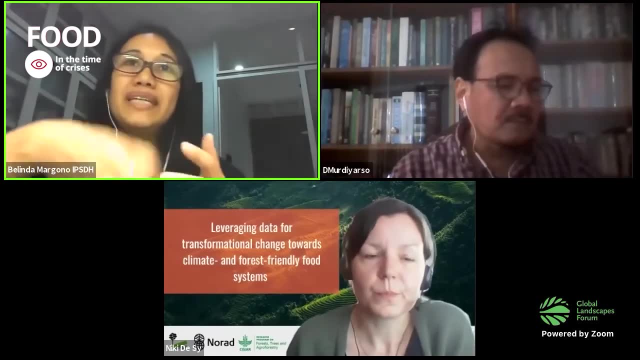 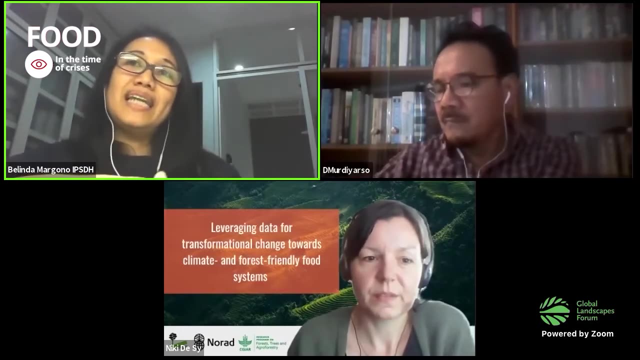 the step is more into to get the data ready. So we need to know about where the data, where the data is and everything. So everything is about getting the data. But the lesson learned- because this is a stepwise approach- is not only getting the data now, but how we can ensure that the quality. 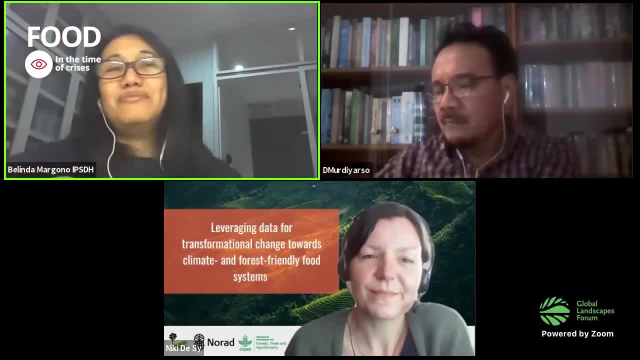 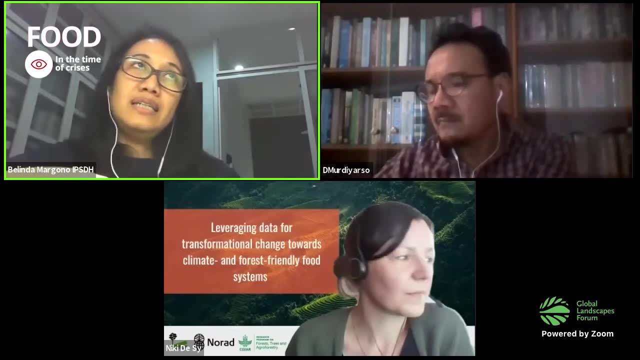 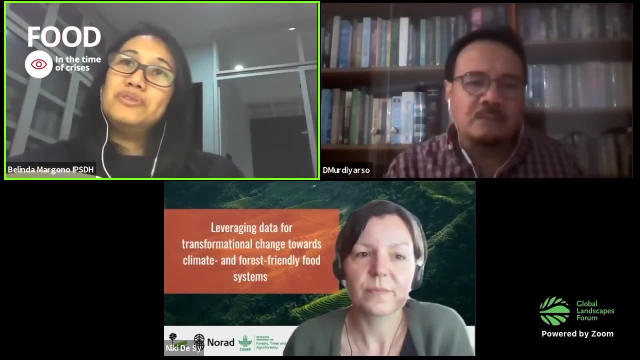 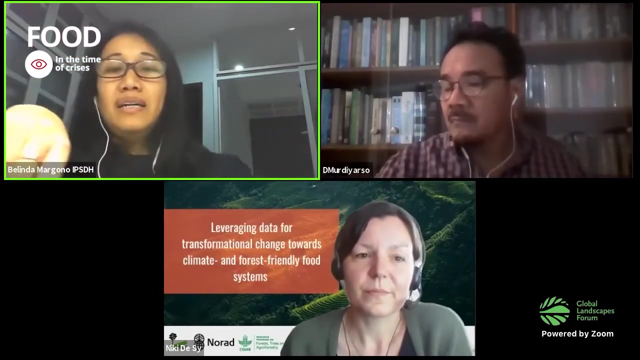 of the data is improving, So that is the the thing that we learned so far. So it's not just providing, but have the information easily accepted and can be provided in the uncertainty or having the accuracy threshold required, especially since Indonesia is one of the red countries. 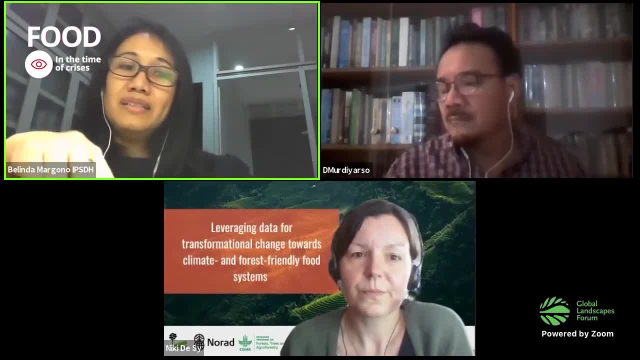 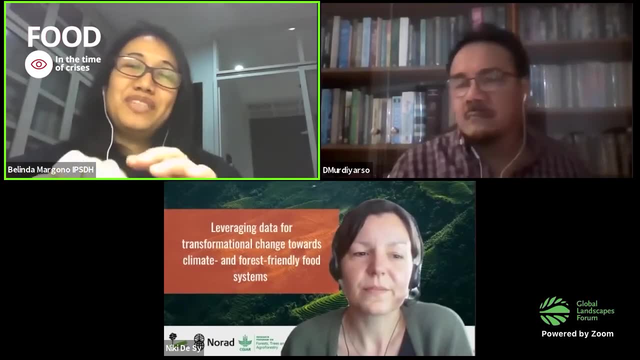 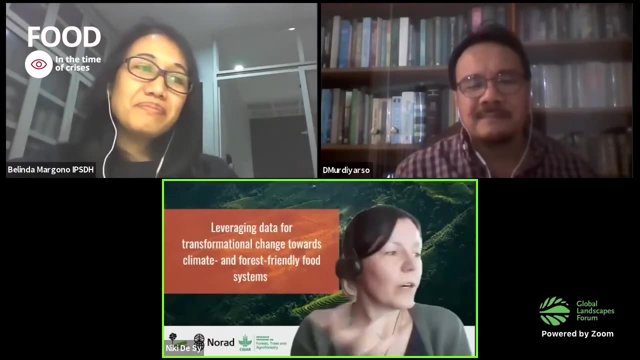 and we almost done with our report, everything on the result based payment. So uncertainty is really our focus on this step. That is the thing we learned from the process. Oh, great. Well, thank you for these insights And there are some interesting questions. 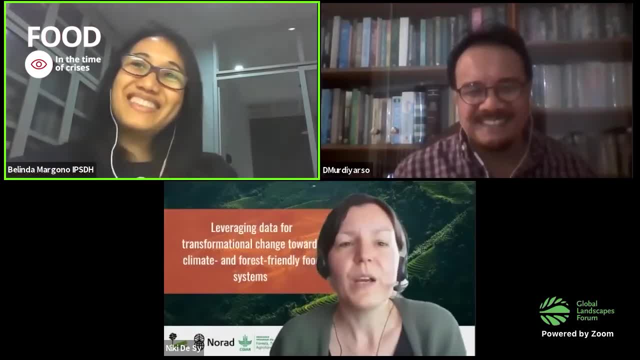 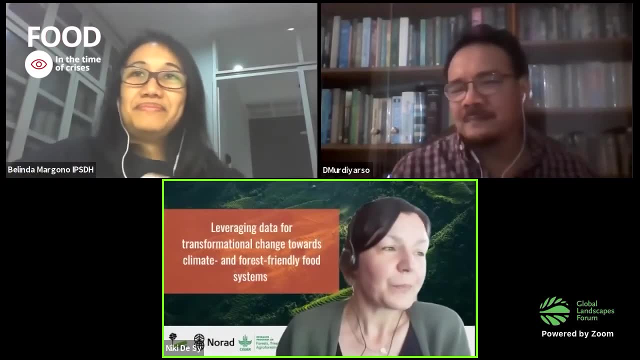 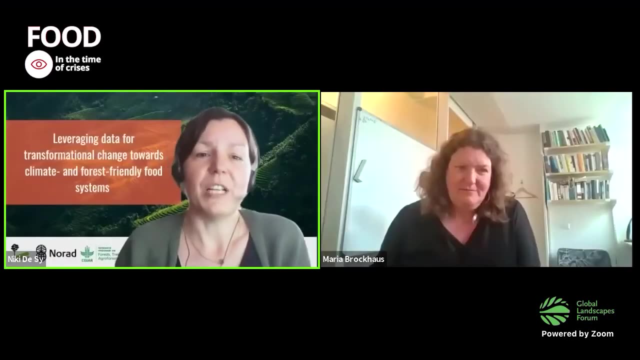 popping up, but I want to keep them for the panel discussion because I think they're relevant for more people. So I want to move on to the next topic. So we're already at our last topic, which is the politics of numbers and information sharing. 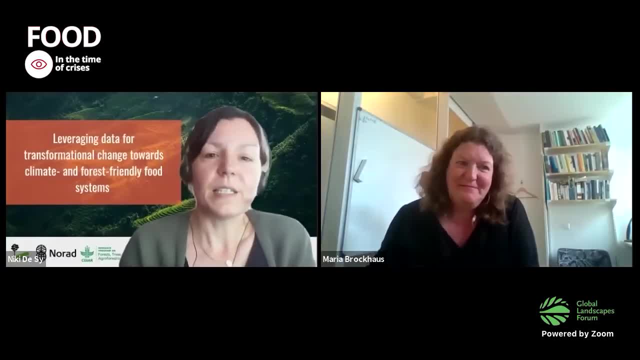 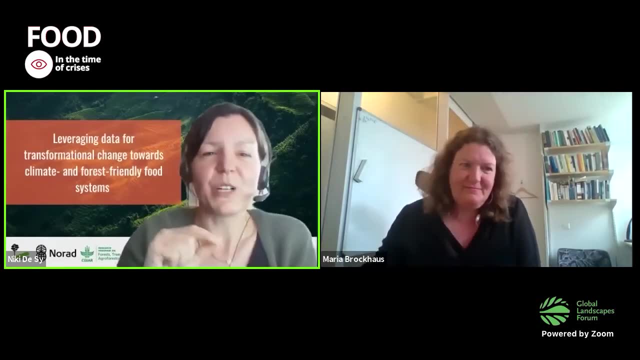 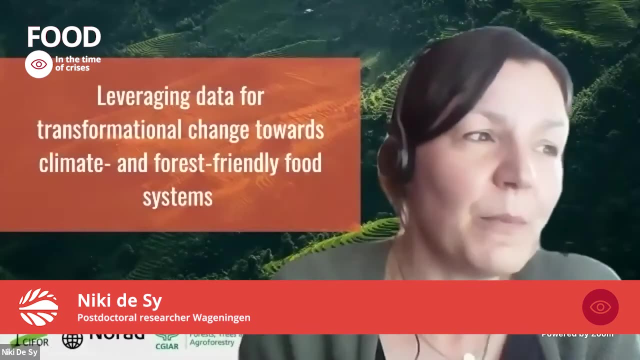 A little bit of a different topic And in this last topic, maybe, Maria, you can close the video now, because we'll watch the video first. I don't know if that matters for the streaming, But so Maria will talk about the politics of numbers. 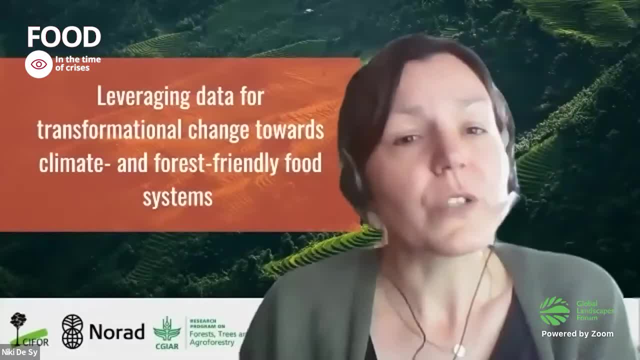 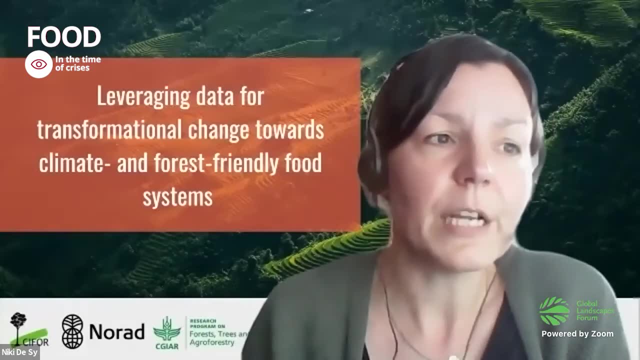 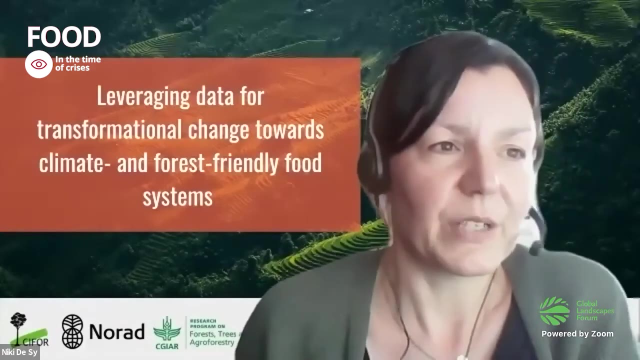 And in her talk she mainly talks in the context of forest governance and REDD+, which is this UNFCCC mechanism for reducing emissions from deforestation and forest degradation, But the key messages she's making are applicable in a much broader context, of course. 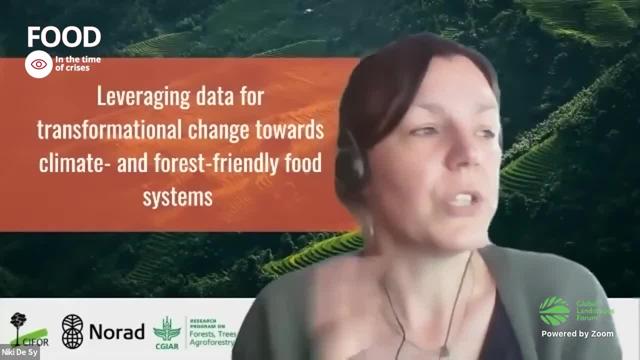 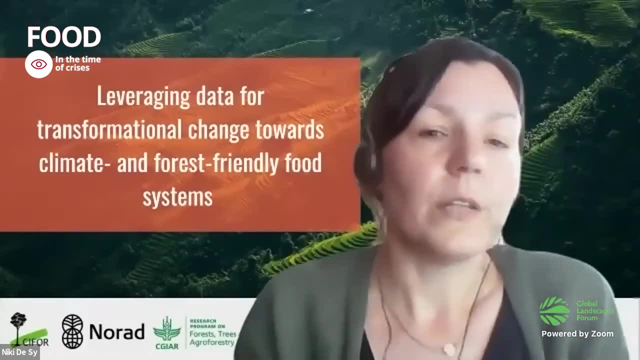 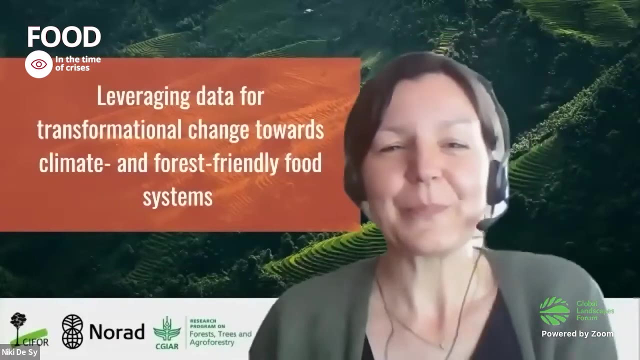 Also, she is not showing any slides during her video, but she also provided us with some background slides that might make it easier to follow or to look at later, And we'll also share those in the chat. So let's look at what she has to say in her video. 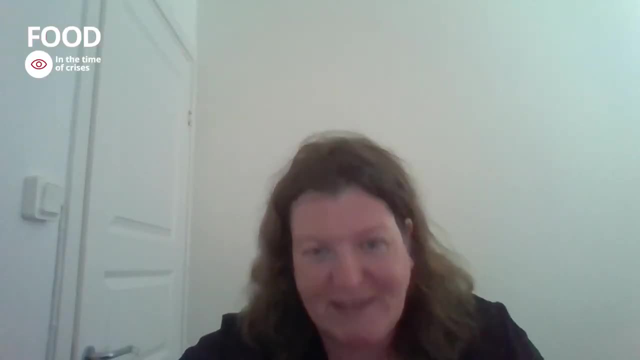 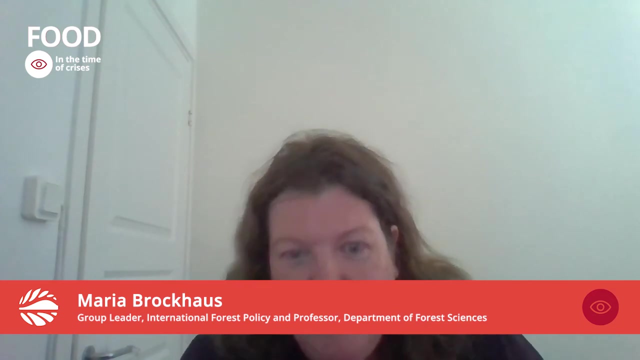 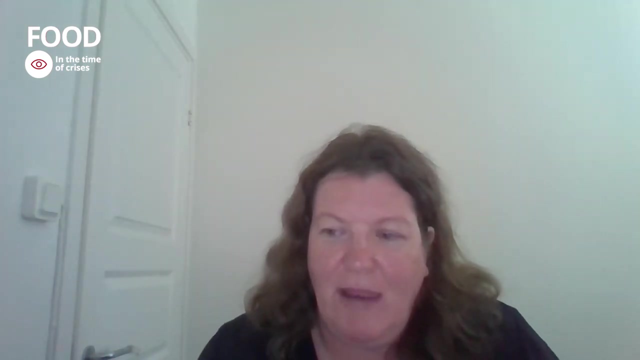 Good afternoon everybody. Hello, My name is Maria Brockhaus, And before I even start with my talk, let me quickly say thank you to the organizers for having me here. The talk that I will present today at this time is maybe for some of you a little bit quite of a journey. 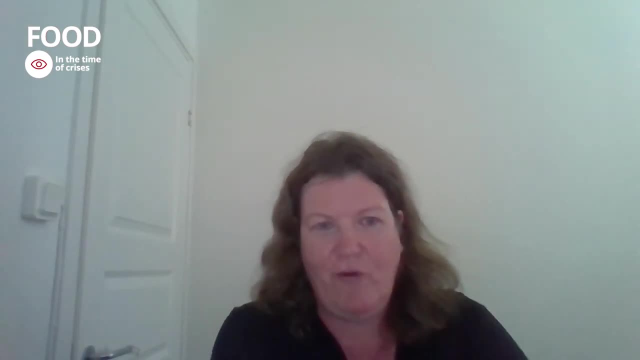 If we look back at the sessions that we had already, the talks that we have heard already, this talk here is about the politics of numbers and information sharing, And what I try to talk in my few minutes that I have here about is actually why it is so important. I want to talk about why it is so important and what. 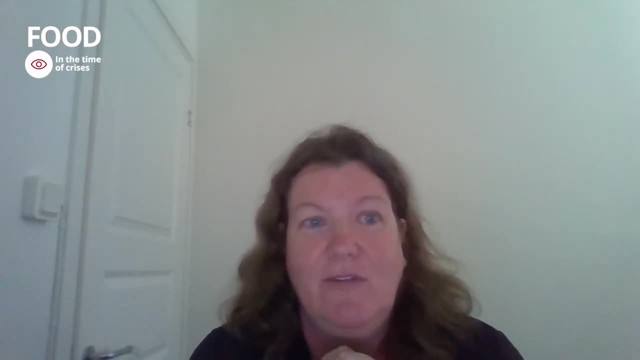 makes numbers so important and why do we have to actually talk about the politics of numbers and information sharing? And one reason for that is, of course, that information is actually a currency in today's world. So facts, rather than speaking for themselves, are selected. 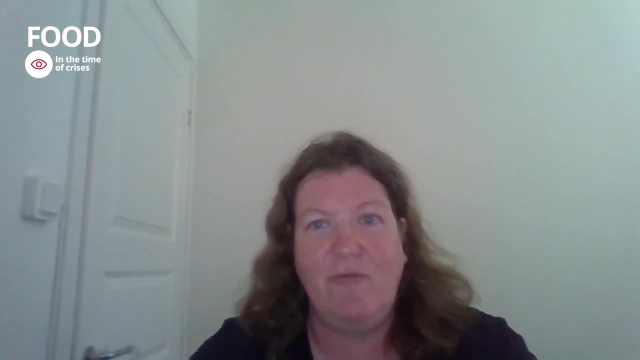 They are interpreted, They are put into context in ways that often reflect the interests or beliefs of the information provider. And information is very much linked and finds its expressions in the ideas and the discourses and narratives that are promoted in the institutions that shape our being. 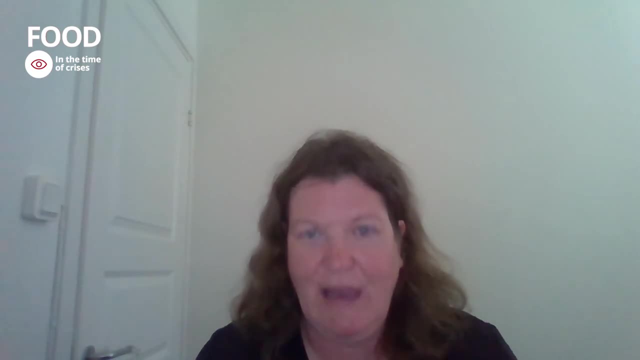 And, of course, driven very much also by the interests, as I mentioned earlier, And there are two quotes that I would like to show here that I feel are very good examples for why it is so important to consider politics when talking about numbers and facts. 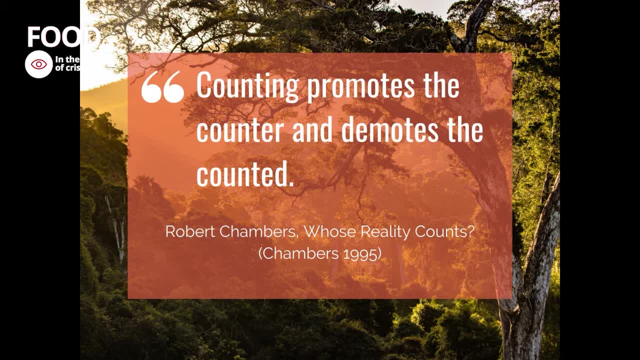 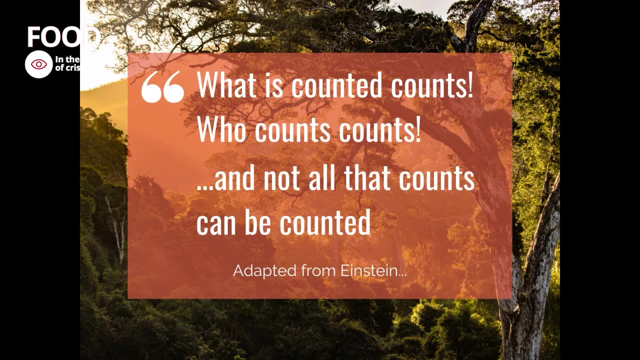 And one is from Robert Chambers, who pointed out that counting promotes actually the counter and demotes the counted. And the other quote I would like to highlight, a little bit adapted I have to say, is that only what is counted counts and who counts counts. 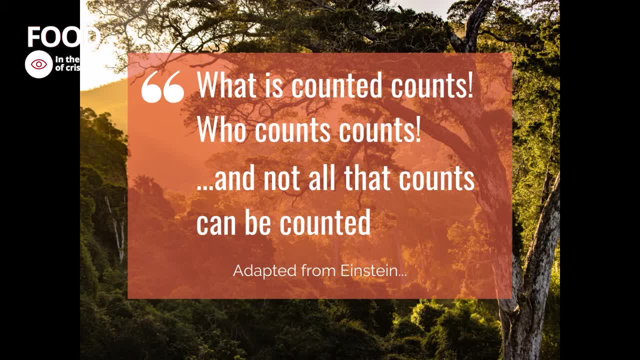 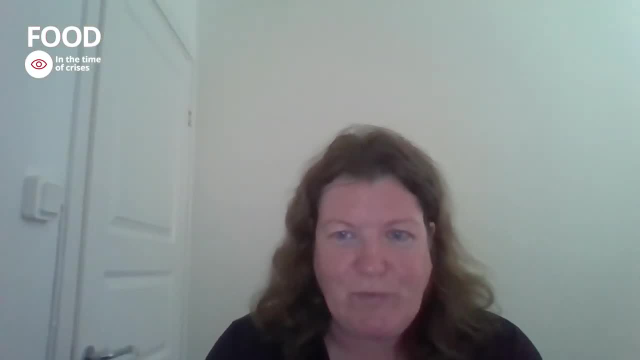 And, as Einstein pointed out, not all that counts can be actually counted, And maybe this sounds a bit like a wordplay, but these are very relevant questions. So what is counted? Who counts? counts is a question, an expression of power, And in the Red Plus world we can see: 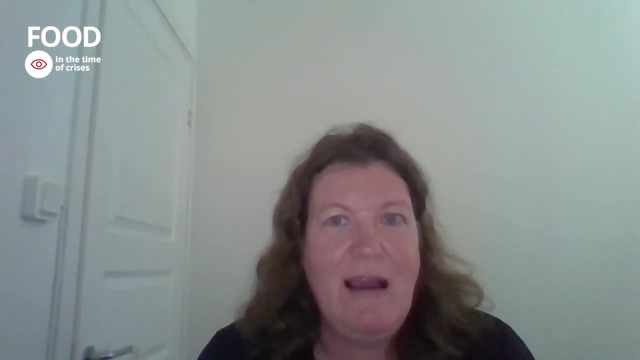 that very clearly, I think, because numbers shape our world, quantify our world and with that also enabling markets, economic transactions, And I think one example where these how important numbers are in Red Plus and how political they are- I think the Stern report is a very good example. 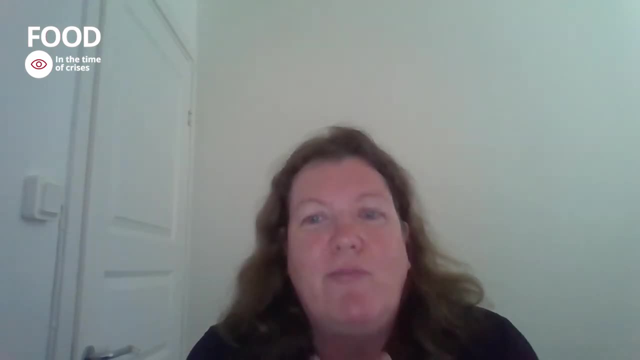 As we all remember, at that time, as this report came out, it provided actual numbers on which policymakers then could actually act on and acknowledge the importance communicated through numbers of forests within the climate change mitigation agenda, And an other key area, of course, is negotiating reference levels. 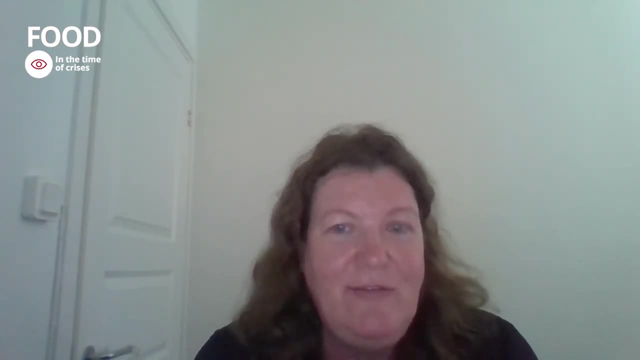 I should have said here setting reference levels, But the reality was that this was a very political negotiated process. Last but not least, what I would like to highlight is holding accountable. So who has access to information? if you think of the Indonesia's Freedom Act of Information? 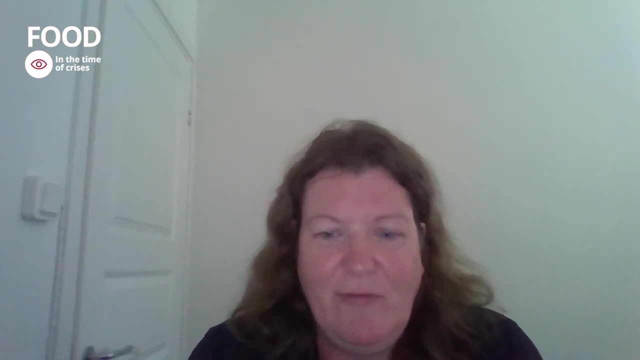 who can, or many other countries with their rights and lack of rights to actually hold those that make promises- states and private sector actors, companies- for zero deforestation, for avoided deforestation? who can hold them accountable? who has access to information that enables accountability and holding accountable? 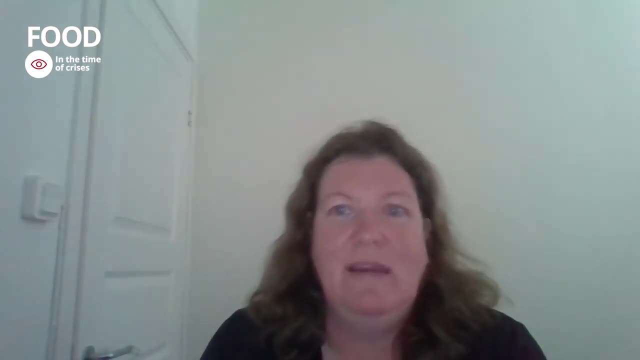 So when Red Plus is rendered technical, when the forest is depoliticized, then the big questions are related and these affect them. That is why we have to talk about politics, Of course, effectiveness, efficiency and equity of Red Plus. What is measured when the focus is on smallholders while ignoring large drivers? 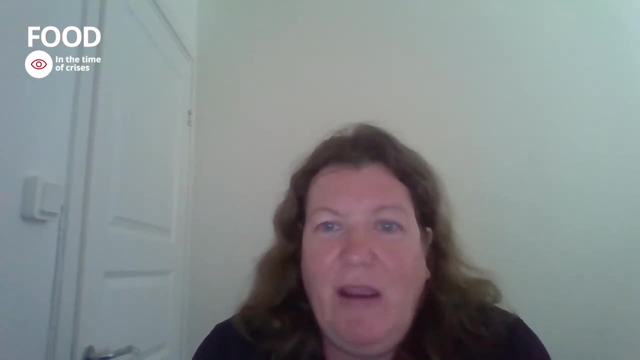 Who measures when we have shallow implementation because there are clashes with belief systems or habits? When it comes to equity, very important is the question of who actually then snoops, as one conference member recently said: snoops in whose backyard? who decides what is measured? 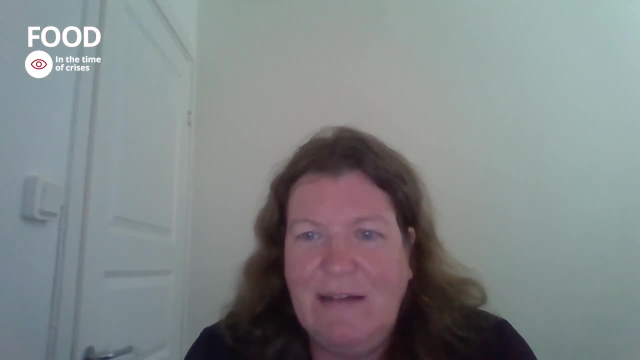 Who owns this technology. Then other political dimensions of numbers are related to who is actually blamed. This goes back to Chamba's, I think quite nicely back to Chamba's quote: who is blamed by what is actually measured? who carries out? 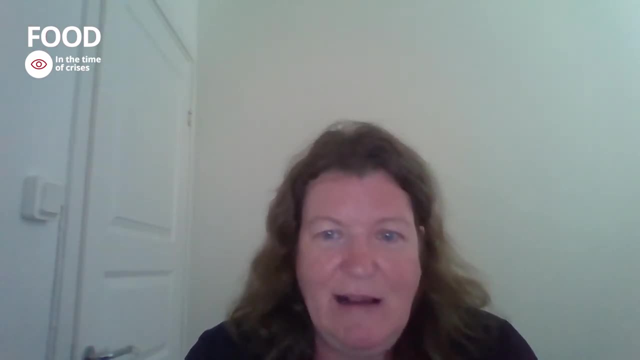 Then the burden, And there are very interesting papers with Parmet Eil, as Kutsch and Turnhout published something along these lines. Who benefits from current measurements is also a big question And, along these lines, whose interests are actually served? 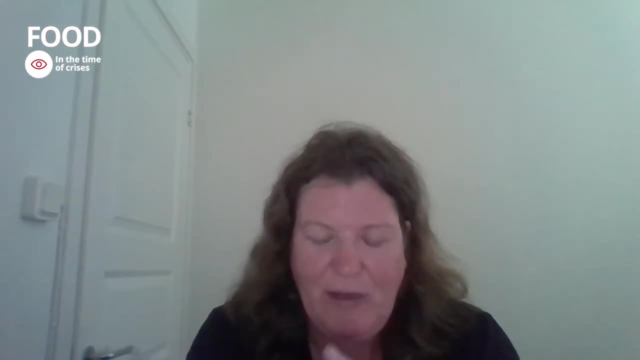 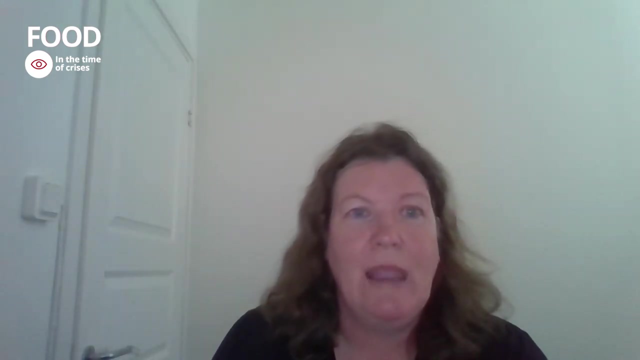 But basically, as Peluso and Vanages call it, political forest is co-produced with forest science experts and the politics of the state. And the political forest is co-produced with forest science experts and the politics of the state. And the political forest is co-produced with forest science experts and the politics of the state. 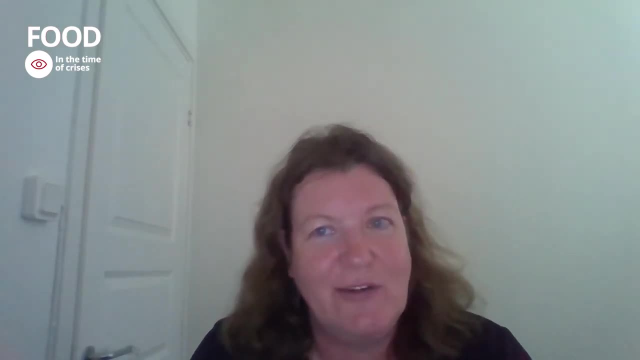 So to come to an end, since my time is running out, so I do hope that with these few minutes at least I could spark some interest and some debate here for the next, for the coming question and answer session, of why I really would very strongly argue that we have to acknowledge the politics of numbers. 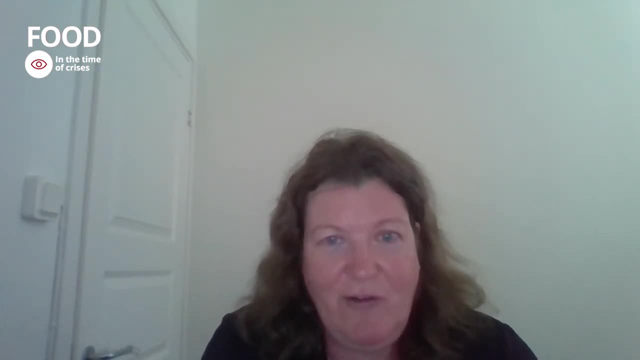 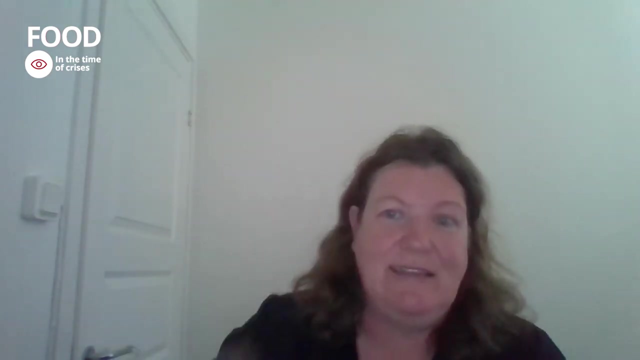 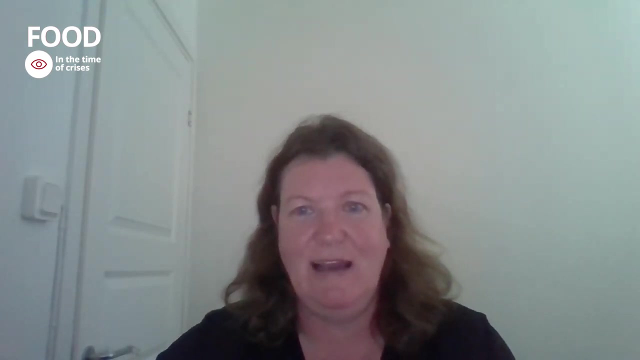 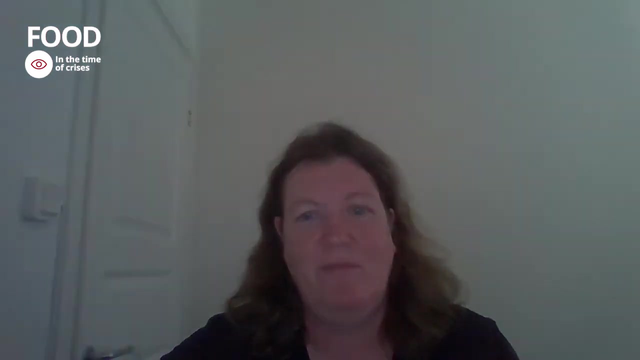 Not understanding power and power imbalances will have trade-offs. It will bring risks throughout the Red Plus policy process, from political agenda setting to implementation, but also to evaluation of it, And ideally this understanding power, power imbalances within the numbers and information in Red Plus policy should happen with science as an honest broker. 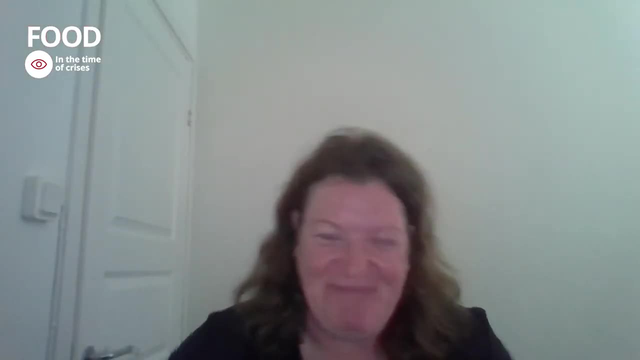 And with that I could just go on, but my time is up, but I really do hope this will spark some debate in the next minutes of this session. Thank you very, very much for listening and talk to you all soon. Thank you, Maria. A very different topic indeed all of a sudden. 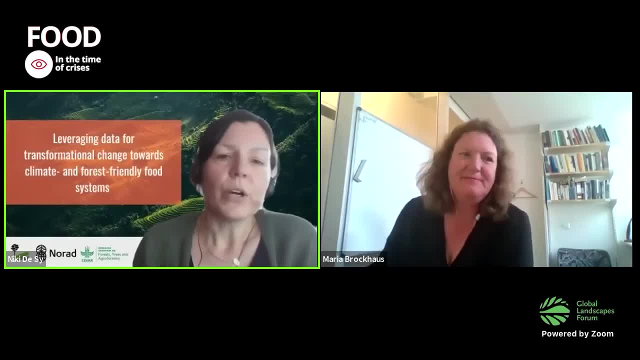 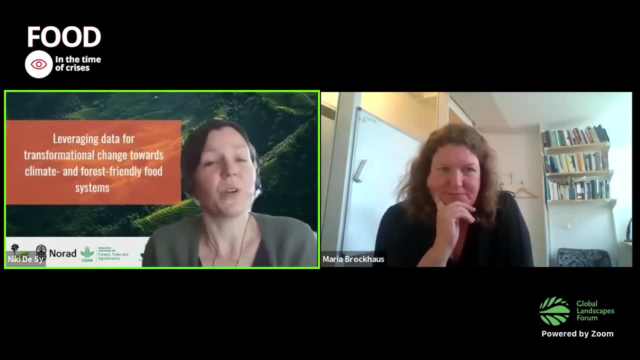 but I think a very valid one. And you know you pose a lot of questions in your video and sort of you know, and of course we have to be aware of these things, but I would almost argue being aware of them is not enough. 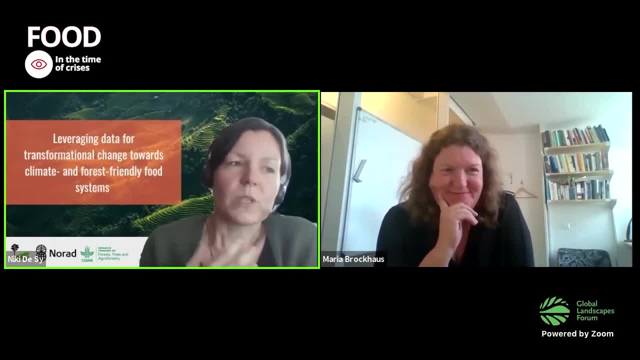 So could you also give us some handholds or some, almost I would say, solution how to how to deal with this when we- you know you already mentioned scientists being honest brokers, but how can a different range of stakeholders actually deal with some? 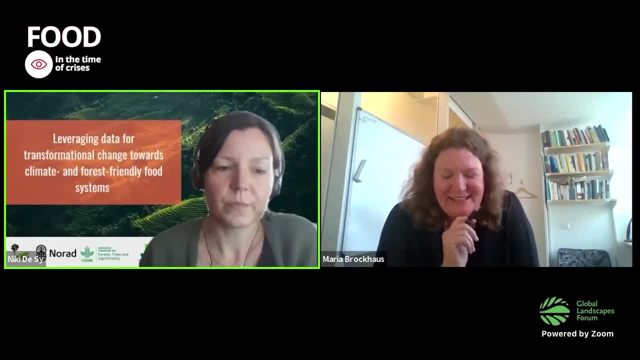 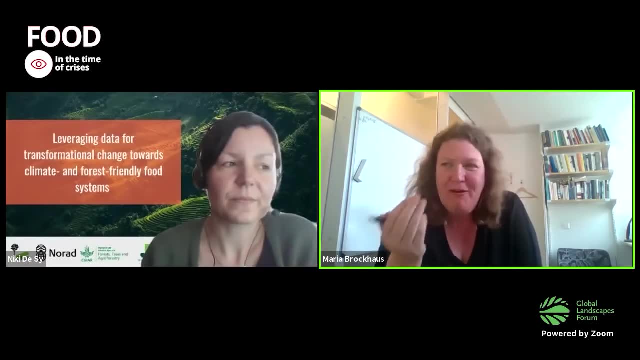 of these issues you mentioned. Thank you very much, Nikki. Maybe, before I even say more, let me say this is not a different topic. The whole point I would try to make is that politics is not different from numbers. Politics are inherent. 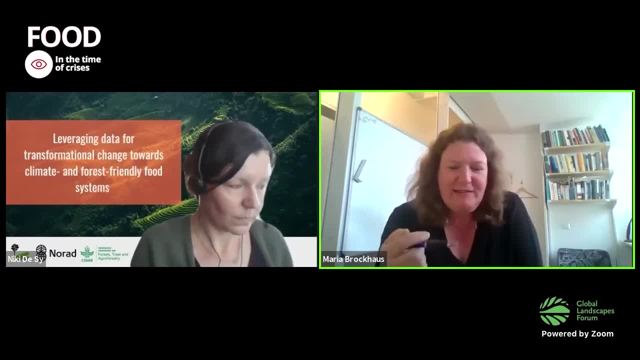 And I think if we just go back through the scene one, scene two, scene three, from the Indonesian reference levels to to the earlier presentation on the ERR system, somebody has selected this data or there was, for example, I think, in- or Christine highlighted that- that that there was very much knowledge or very much. 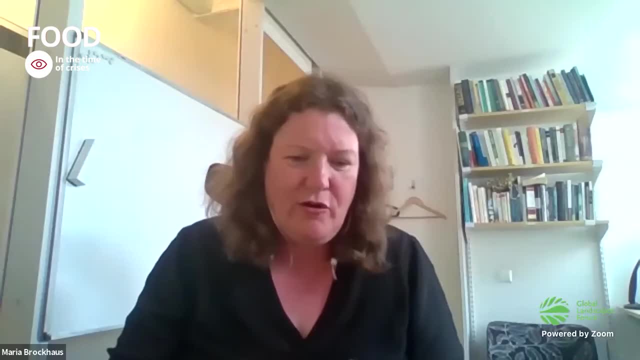 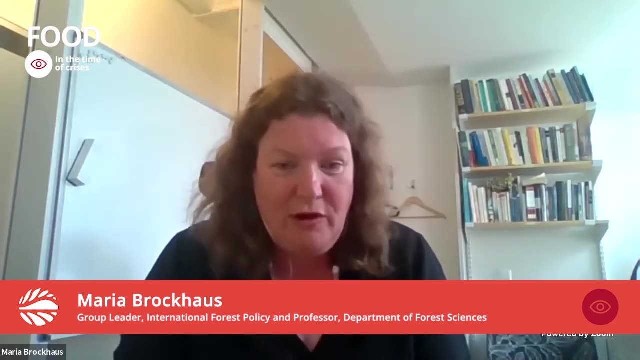 information available on fertilizers, non-organic fertilizer, Those kind of things are super fascinating because there's a reason for that, And the reason for that might be related to politics and to power. So the whole point is this is not, if you talk about numbers, 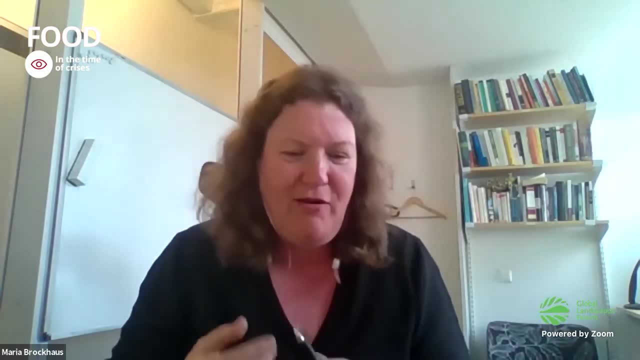 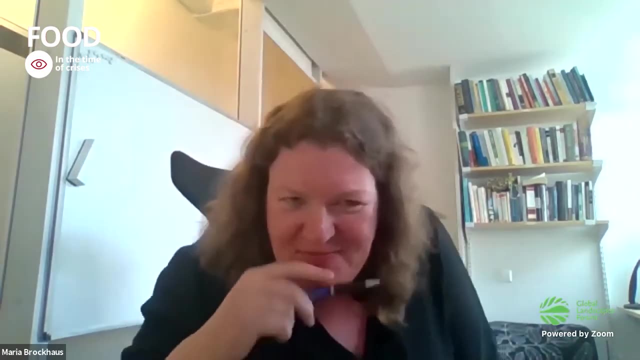 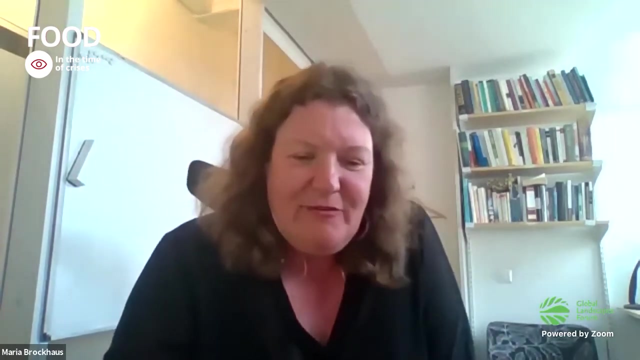 then we also have to talk about politics and the power of making choices or deciding over numbers, And I understand that you asked me for a solution or a response here to what can be done now. I think really seriously, the very first important part is that we get 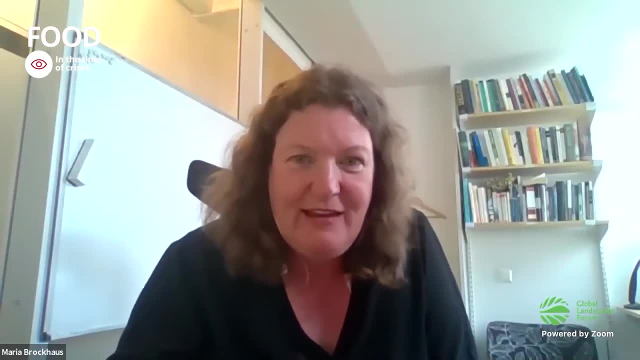 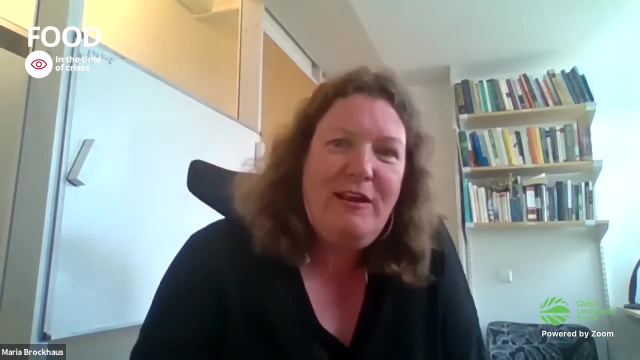 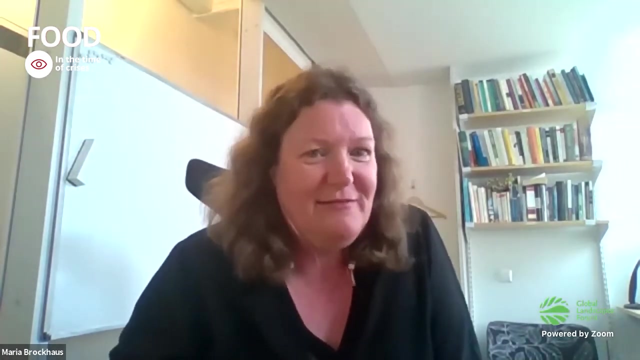 aware that we understand, that, we acknowledge that numbers are nothing neutral, And this whole rendering technical power politics did not come up in any of the earlier talks today. So I would really challenge all of us, including myself in my own work, to not forget about politics and power. 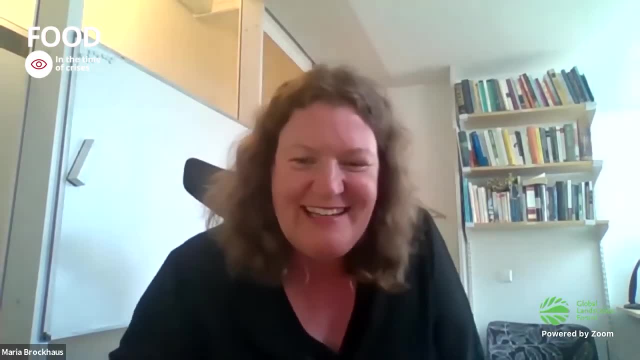 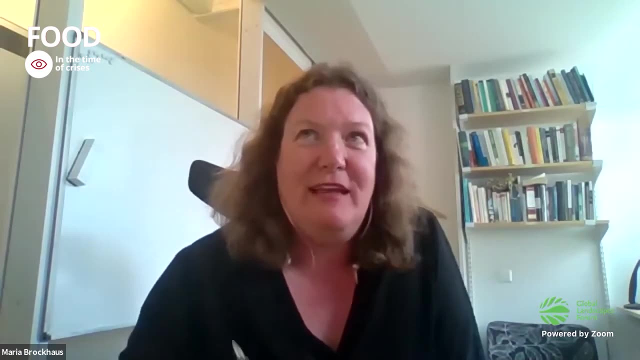 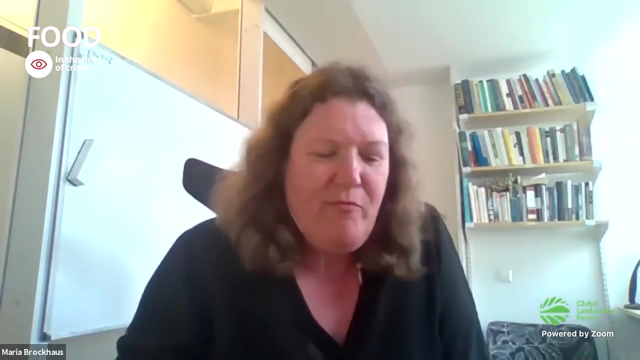 Let me talk about that. That's maybe not the solution or the technical answer you would like to have, But I think the very most important step is that we are aware of that And maybe more nuanced as a more nuanced answer- Trying to be a bit short here- is: it starts with models. 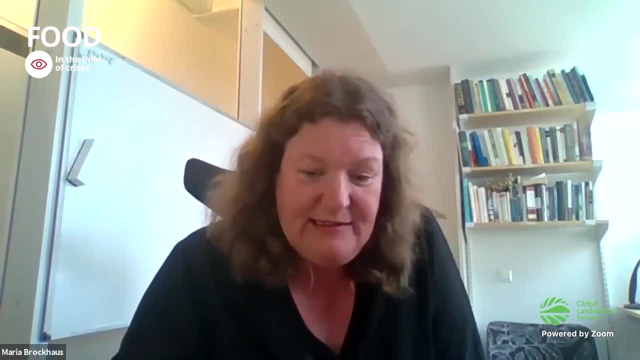 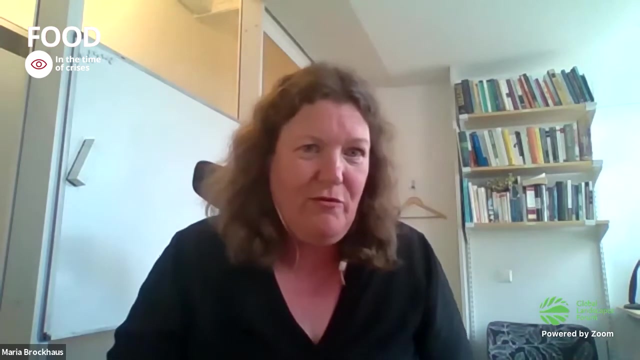 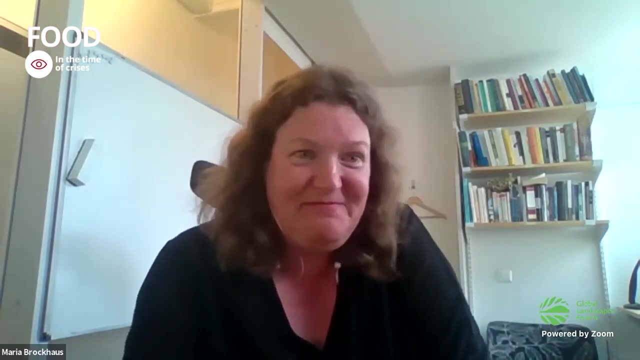 So maybe being a scientist as an expert community much more accurate about what we are talking. What are our underlying assumptions here? But- and I think that's these are the steps where we as a community, expert community, can also contribute to acknowledge and be aware of politics and power when talking about data. 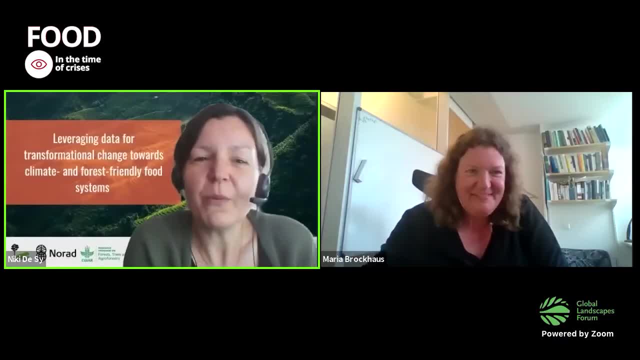 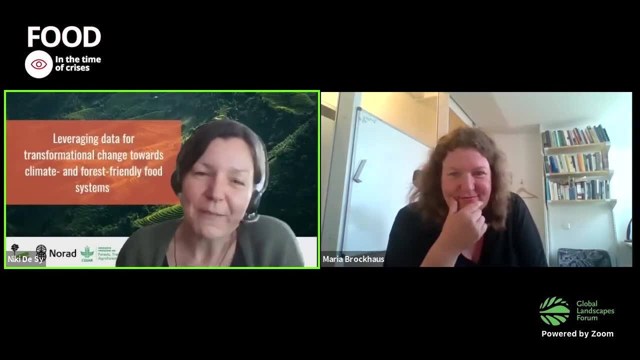 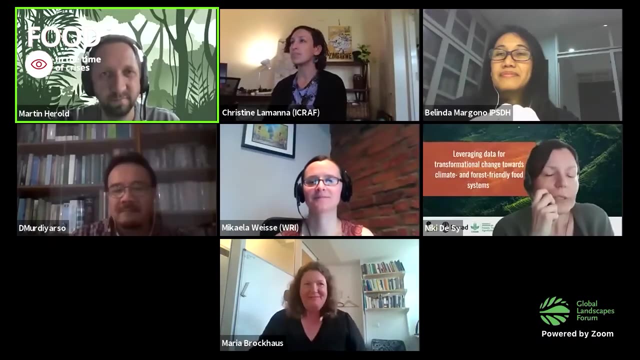 Well, it's nice that you challenged also the other speakers, maybe. So I want to take the opportunity to just start the panel discussion now. So I invite everyone to turn on their cameras and I want to see if people want to react to this thing, like because I mean I 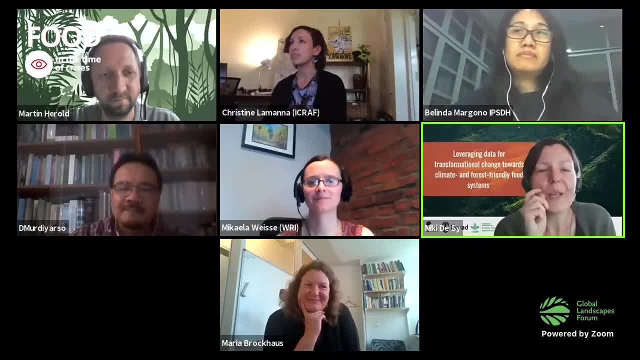 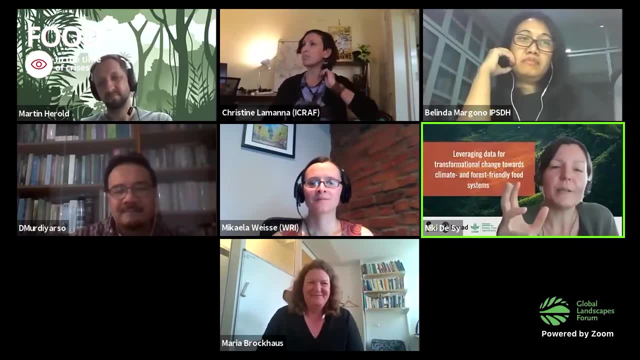 I'm not asking for technical solutions because I think exactly the point is: not everything is technical, But I do sometimes think, yes, I follow your ideas, but I find it also very difficult to deal with them as a more technical person- And I can imagine I'm not the only one. 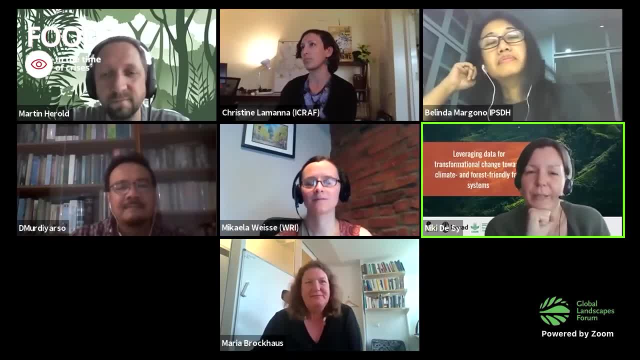 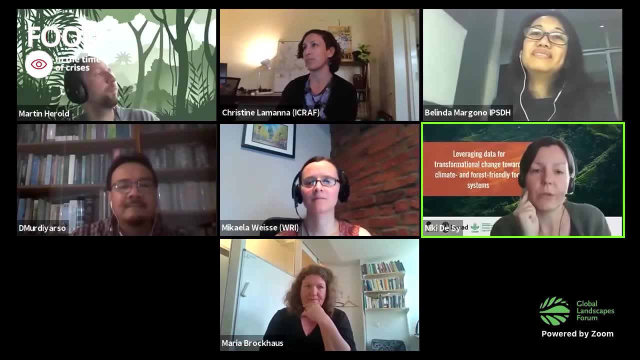 And so I want to know from the from the other people speakers here, whether they, whether it was something that they considered in the processes they just now described, or dealt with it in a certain way, Or is it also very difficult to do that? 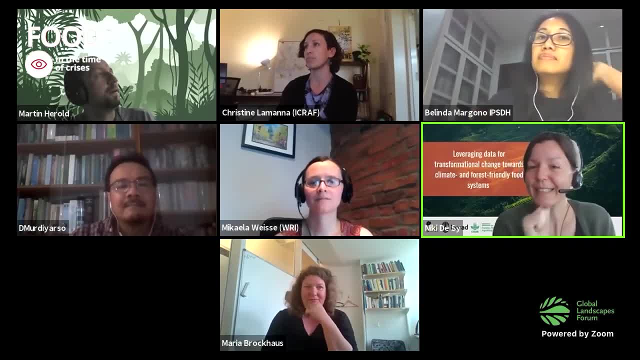 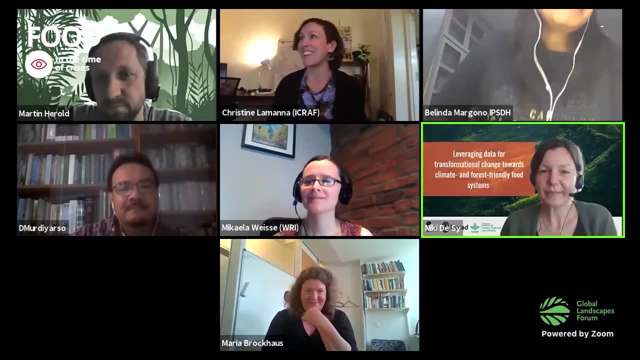 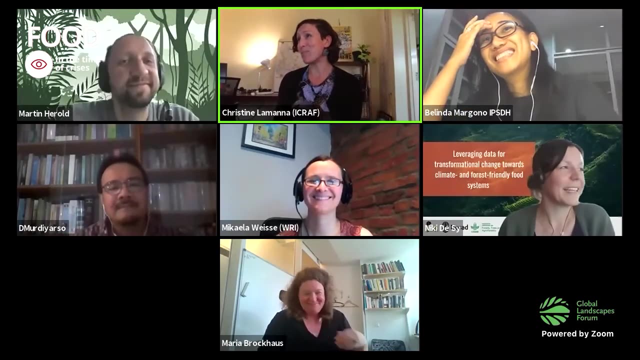 So I don't know if there's somebody who likes to react on that. Yeah, Christine, go ahead. OK, thanks so much, Maria, for a really inspiring and important talk. I really you have a big fan now. One one thing I wanted to say, and we're in a session. 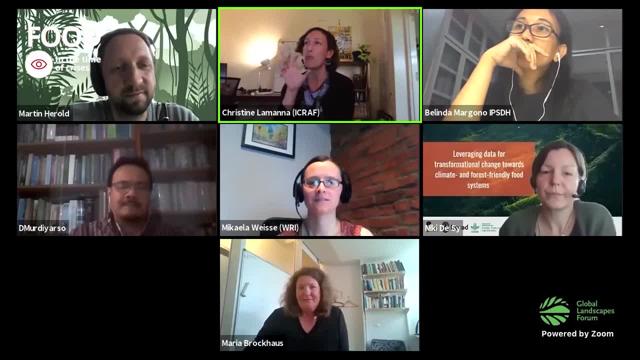 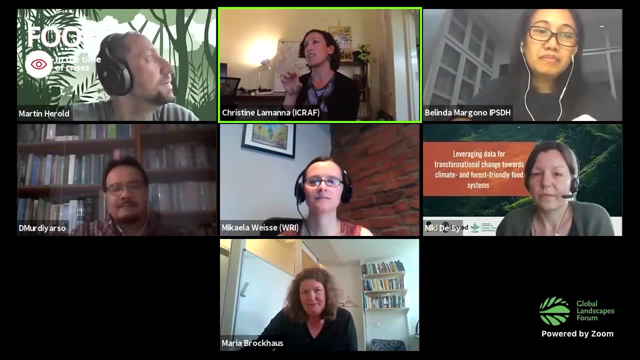 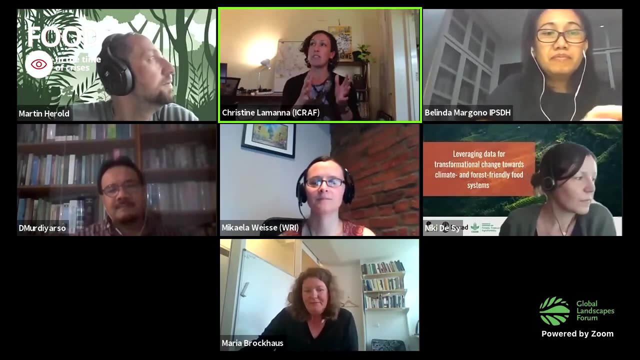 on data, but was also that data is only kind of one piece of evidence And there are so many other types of evidence that are really important for decision making and policy making, And so one of the things that we've tried to do- a lot of it has been around- 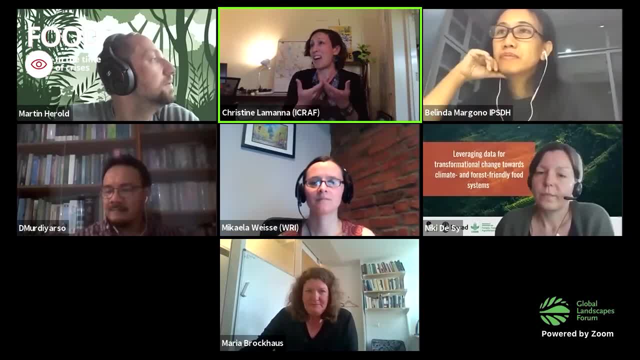 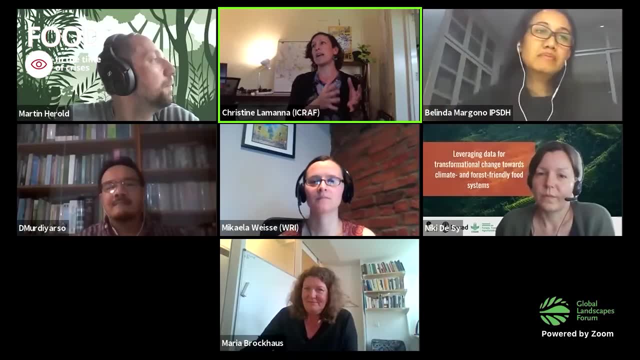 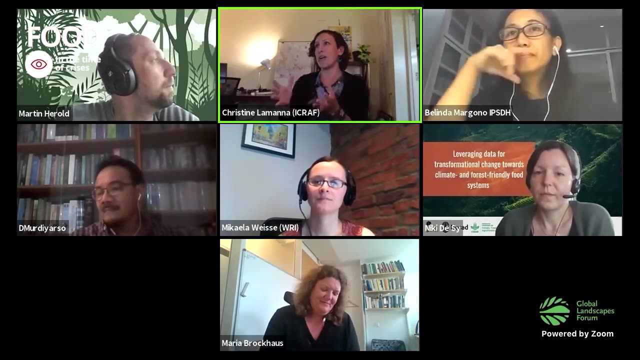 developing this database and trying to make it responsive and answer questions that people have, But then how do people actually go about using that data? So how can you combine Hardness- hard evidence that's coming from one epistemology- with other ways of knowing and other sources of information, including farmers experiences? 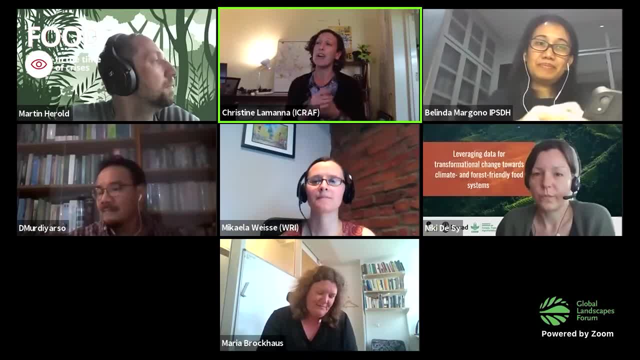 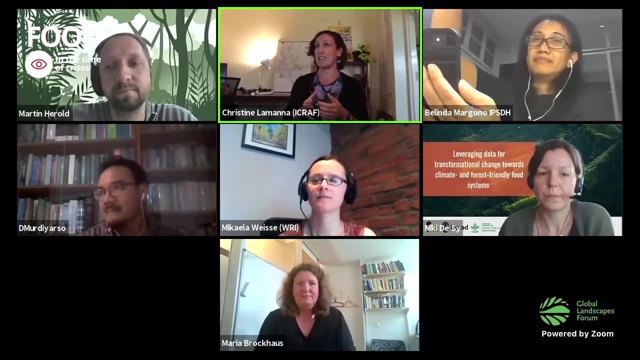 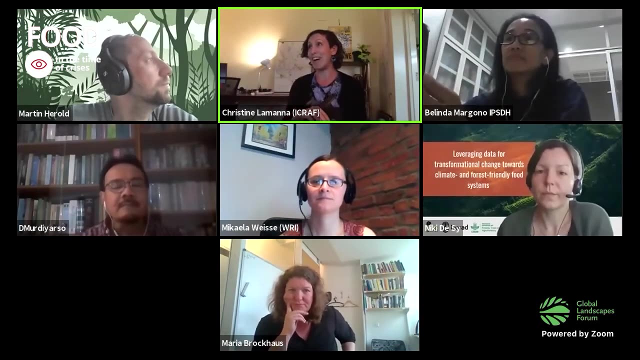 including all the other values and factors that are going on when you have to make a national policy or a community action plan. So so, even though I think the data is important and enables a lot of decision making, like the example from Peru is mind blowing to me. 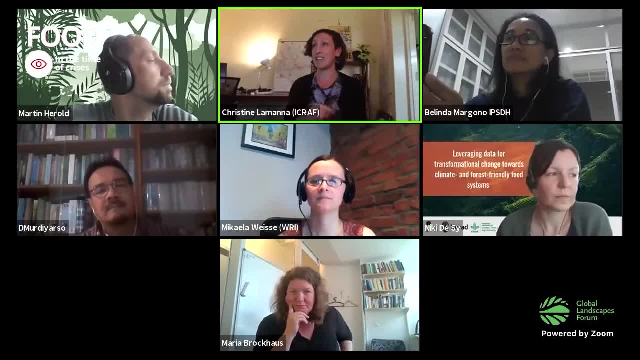 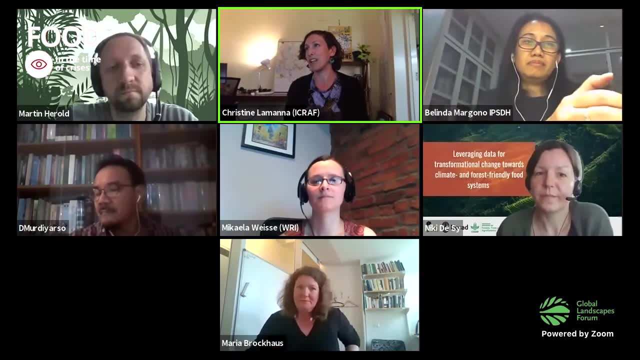 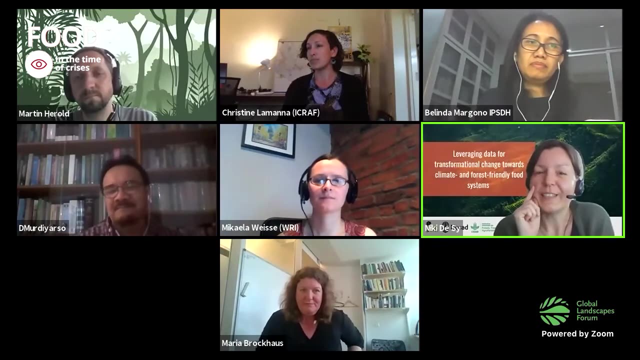 that people can instantly get an alert and go out to the field and have more agency over their area. but it's only one part of the puzzle, And so thanks for really highlighting that. It is also very interesting perspective as well indeed, and we are also getting 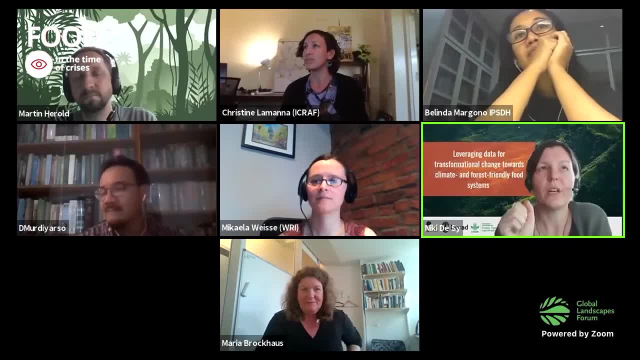 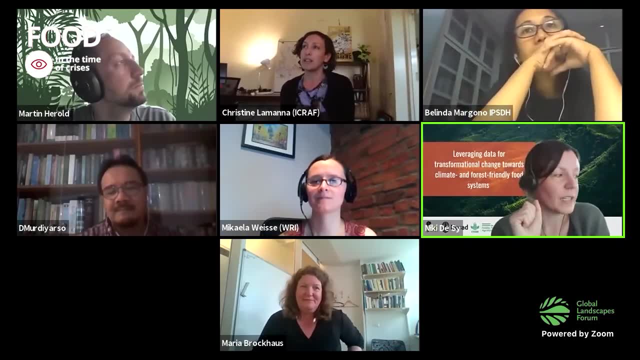 other questions on this. so how can we ensure that we also have, let's say, non biased data, or at least a little bit less biased than we have sometimes? that really represents all interest And and also be critical, as, I guess, as researchers. 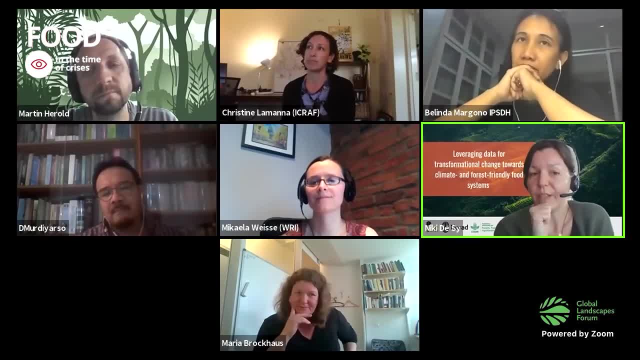 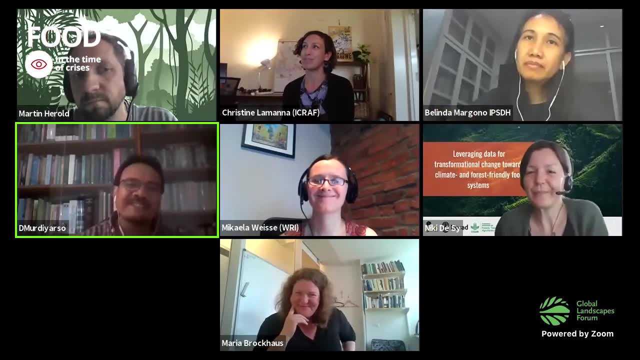 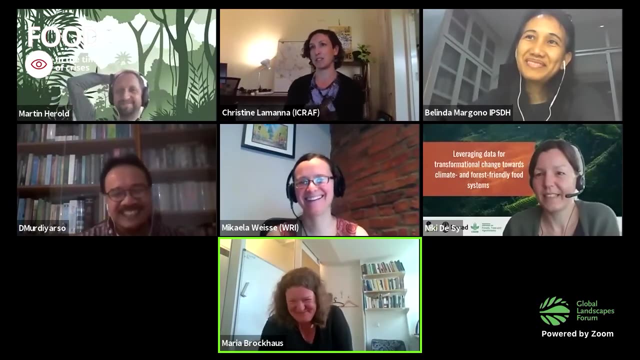 How can we be self-critical on that? And so I don't know if anyone wants to react on that. I think, Danielle, I see, Yes, Maria is always challenging Who counts. I take that as a compliment. Thank you, Danielle. 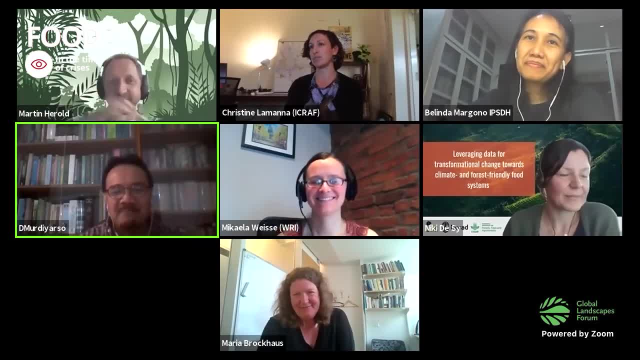 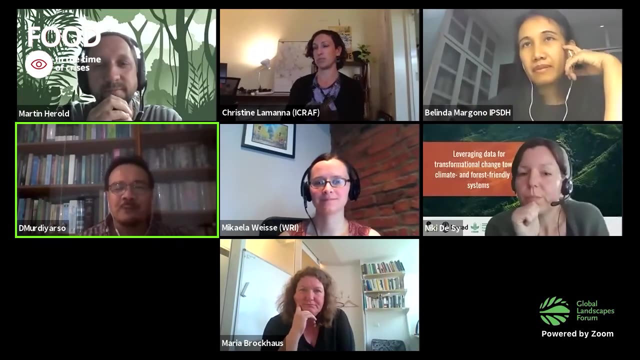 Who can count? Yes, I agree with that, But I'm not entirely agree with the fact, the fact that you, you always absorb in your numbers so that you can be biased with that. Well, we, we know what we call expert system and in this, in this system, 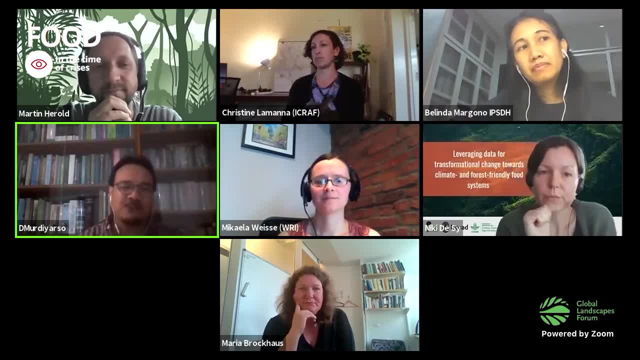 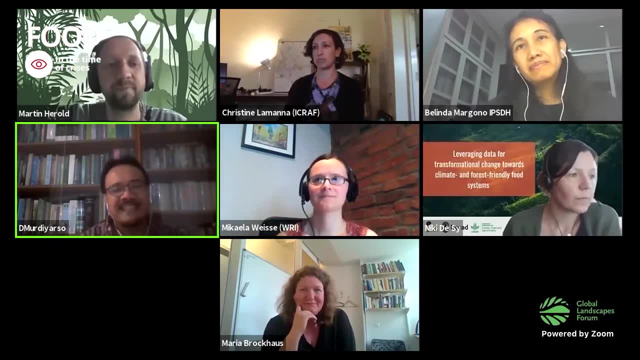 we try to be not biased towards us, or towards me or towards the scientists, But let's the number tell themself about what it is And, statistically speaking, we are talking about. you know range. There's a lower case, upper case. 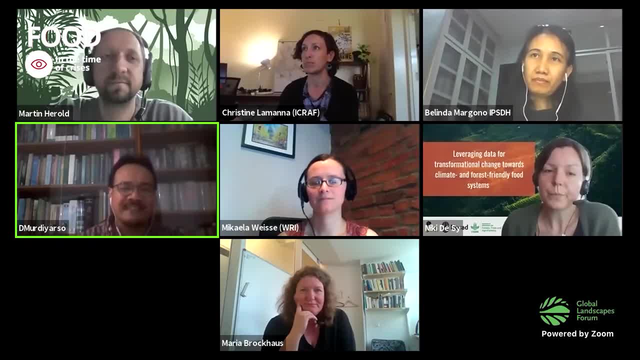 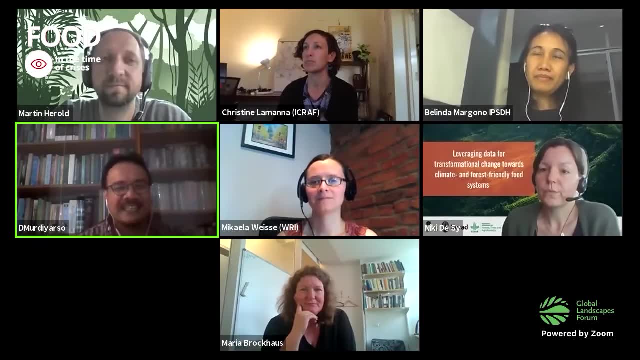 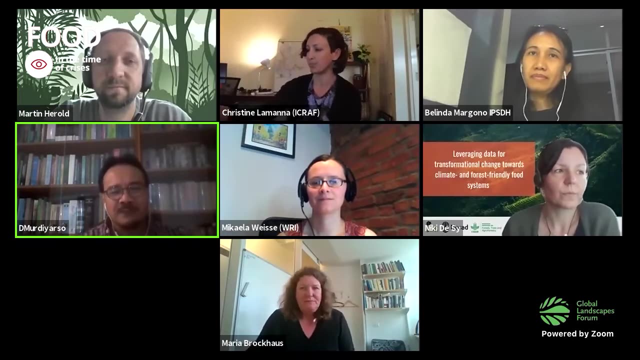 And then you come up with the proxy of this thing. So You, you are normalized in that case that this is not only the idea or the intention of who counts, but also the counted one, which is the number itself. So in the IPCC process people collect lots of data. 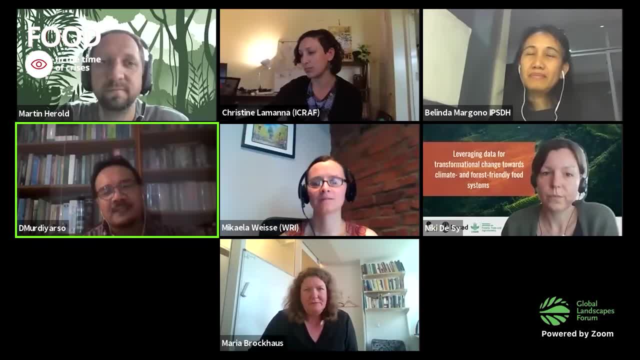 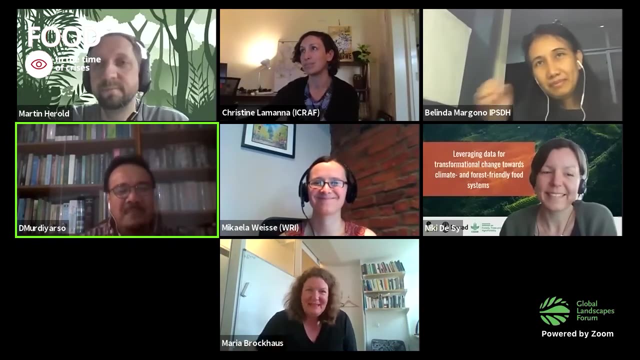 That's why they're database, And from here it is the country who can choose and decide which one is the most appropriate. Then the issue of politics of number really counts. I'm not, I'm not defending myself, but that's. that's the way I understand it. 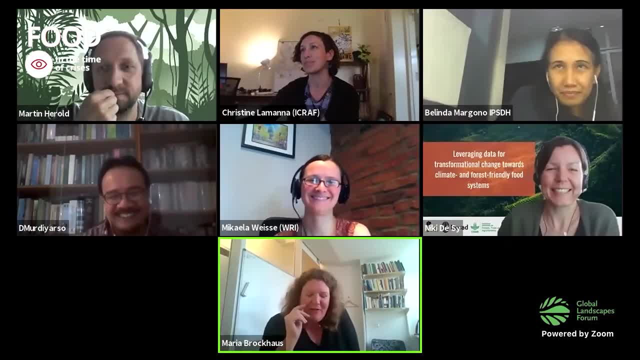 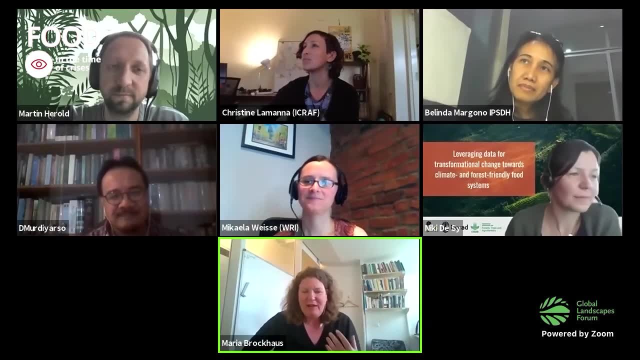 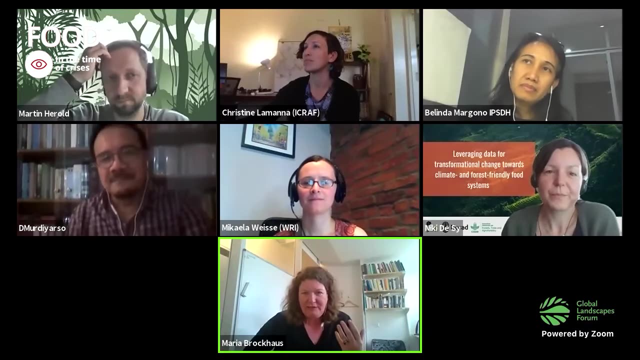 I think Maria wants to react to that Right. Go ahead Very, very quickly, because actually both of you make very interesting points, because of course there are mechanisms in place And I'm really to enhance quality. I think also earlier Belinda mentioned improving quality as 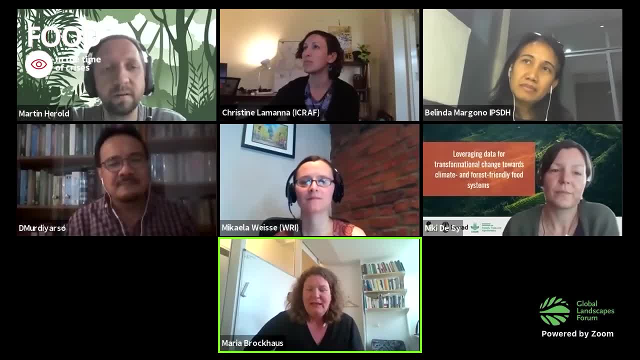 an ambition that drives Indonesian government also, But quality is more than getting the process right. I think it's also asking the question: who has provided the initial data? And that's a little bit what I would love to have a discussion with Christine about. 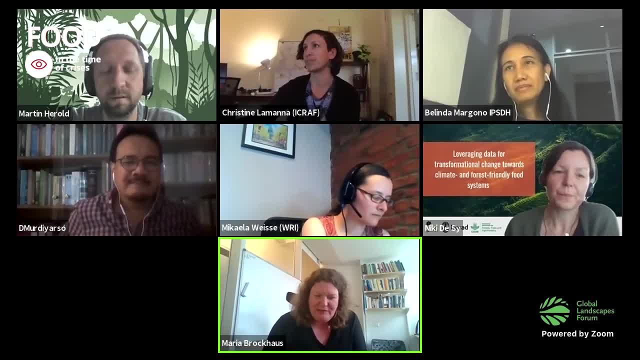 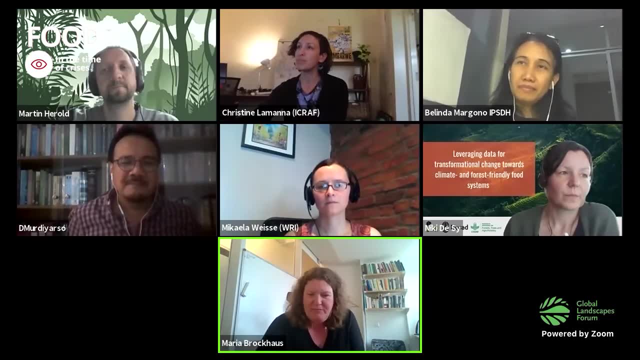 So we talked about bias. You mentioned the IPCC, Daniel, But my question is: for example, there's some literature out there that looks at the authorship in the IPCC and looks at who actually puts this IPCC together. Who are the authors? 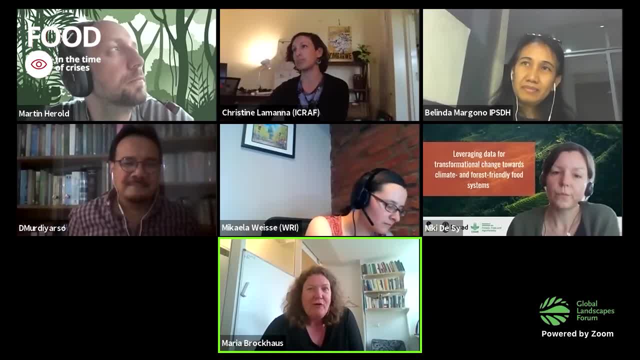 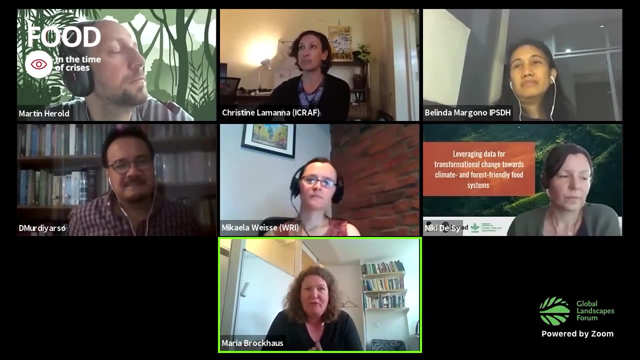 Who are the lead authors of the different chapters And, of course, what you then have is a very North American European bias. very quickly And again, IPCC, I think, make a lot of efforts to kind of correct these issues, because that means you don't have all perspectives. 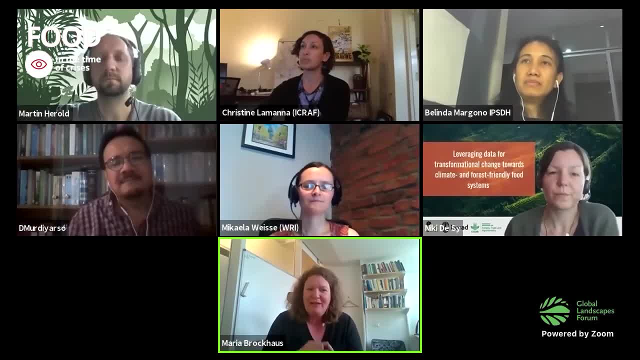 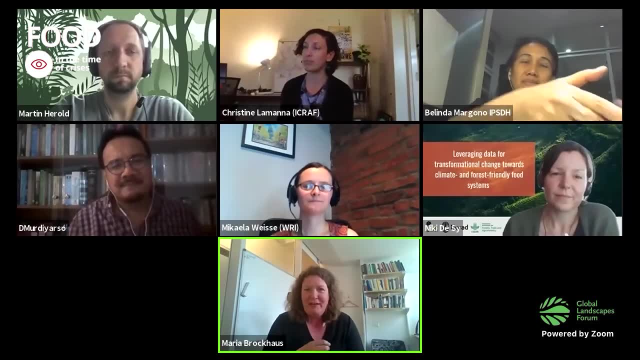 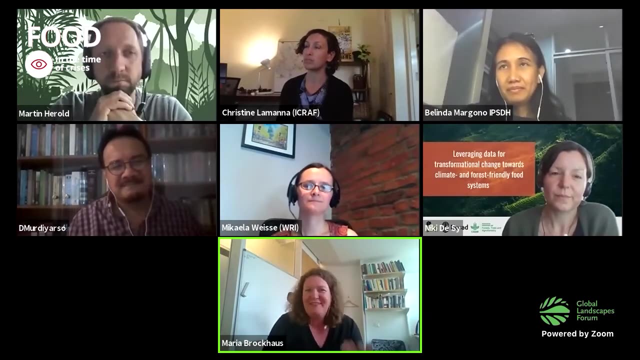 And that is simply what I'm calling for. It's this: being aware that politics are everywhere. This idea of a neutral number is flawed. There is no neutral number because somebody made the decision to count this number, So that means there is already politics involved. 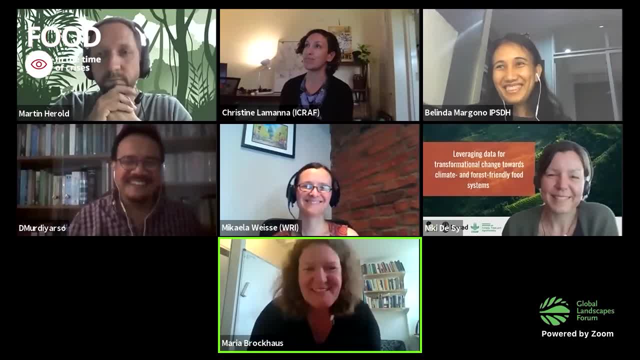 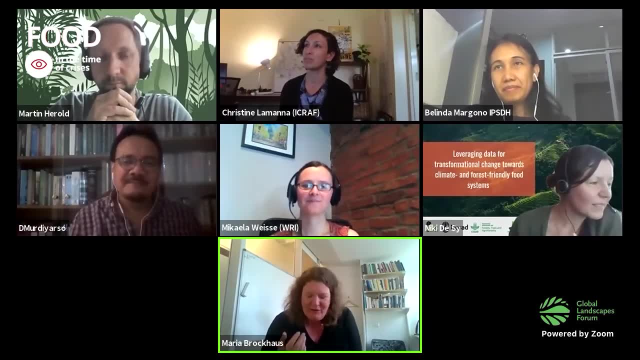 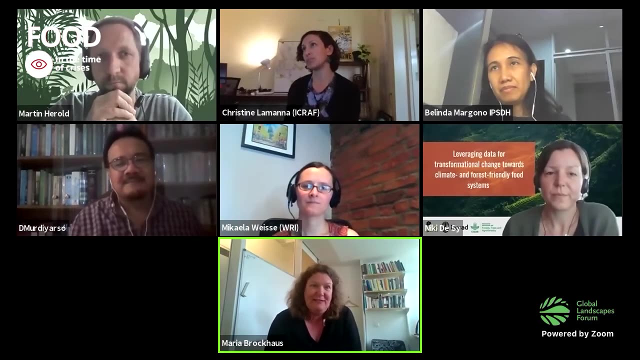 That's my point, And sorry for jumping in and talking so much here, But I think it's important to avoid this technicalization, This idea of neutrality. if you want to deal with politics and power, step one is to be aware of it and to look for it also. 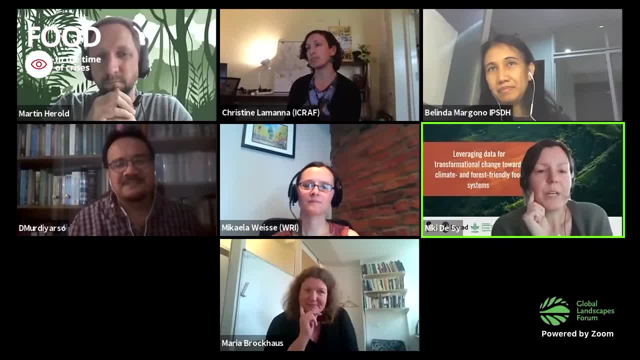 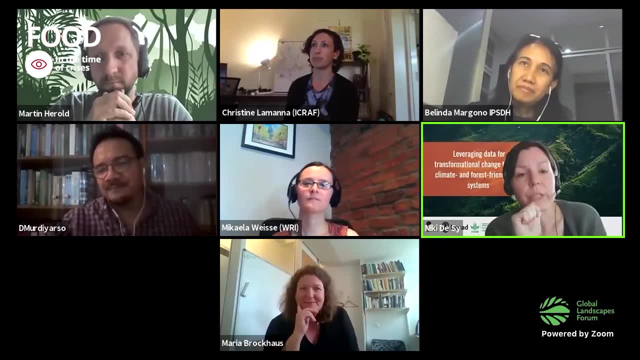 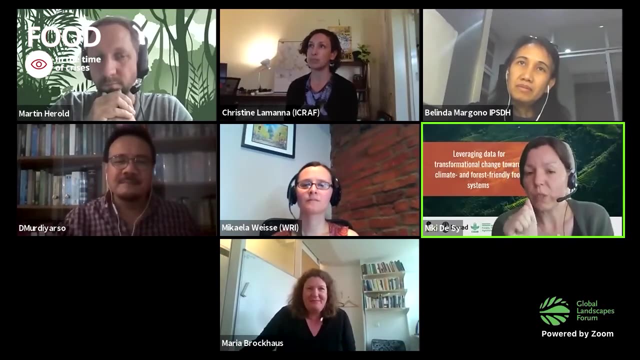 Now I think one of the questions that are also raised by the audience is whether community generated or co-produced data can be part of the solution here, And sort of: is that possible to to, to incorporate that or do that more? And I don't know if anyone wants to react on that, because if done, 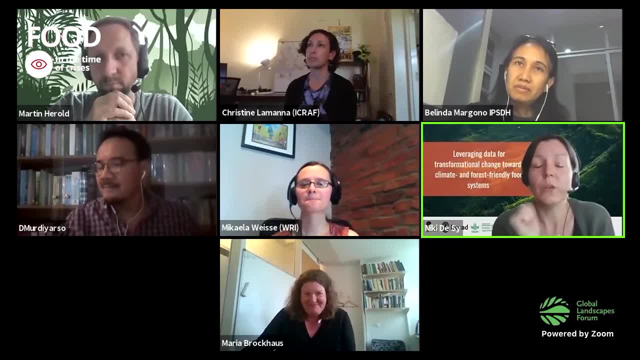 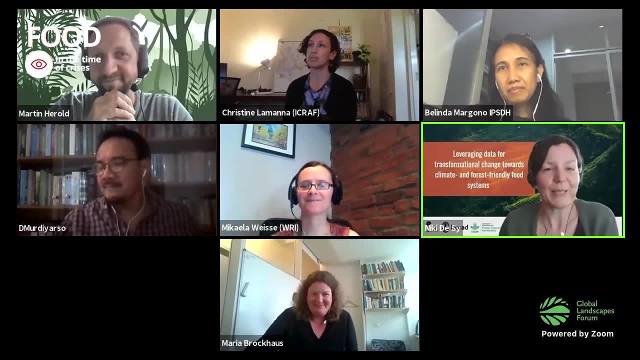 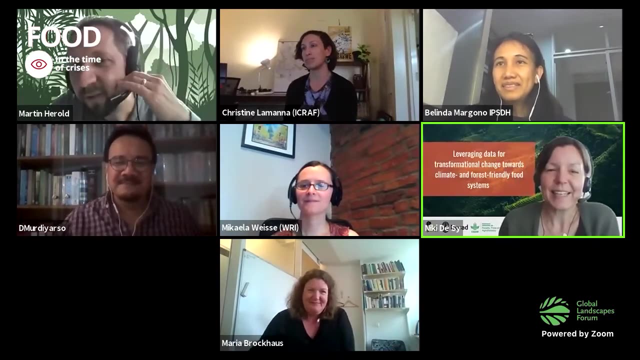 it, or because they see new ways of doing that, for example, with new technologies. So I'm also looking a little bit at the people that maybe haven't spoken yet, if they want to react, or someone else. No, takers, Martin, you wanted to. 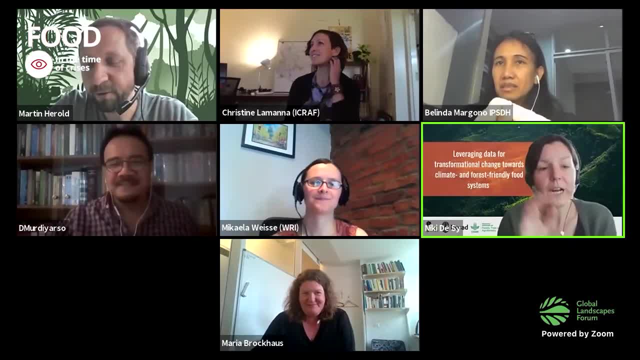 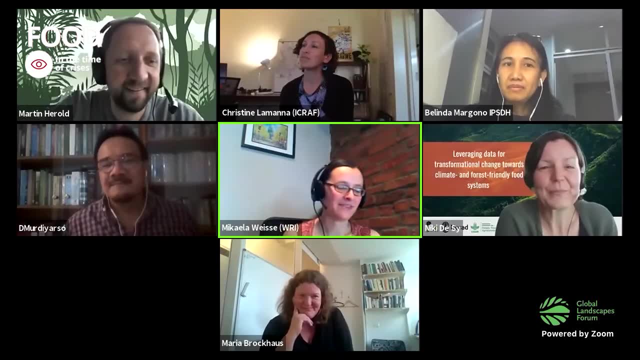 And I know Michaela had her hand up for a while. Oh sorry, Oh, I'm sorry, I don't see your hand, Michaela. I'm sorry, Just go ahead. Oh, no, worries, No, I was just going to comment and maybe 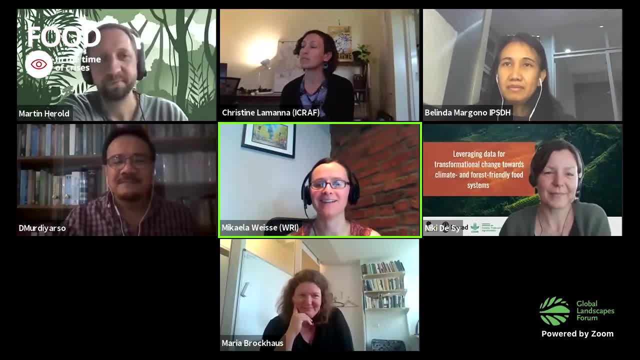 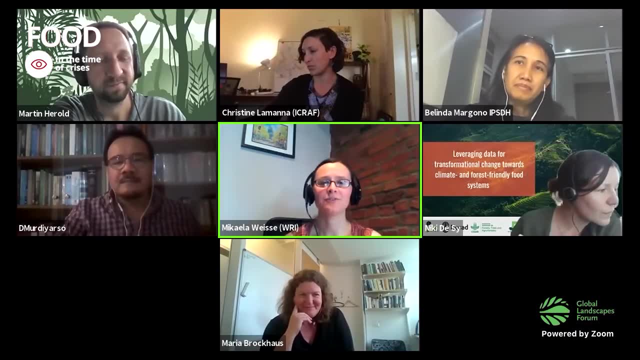 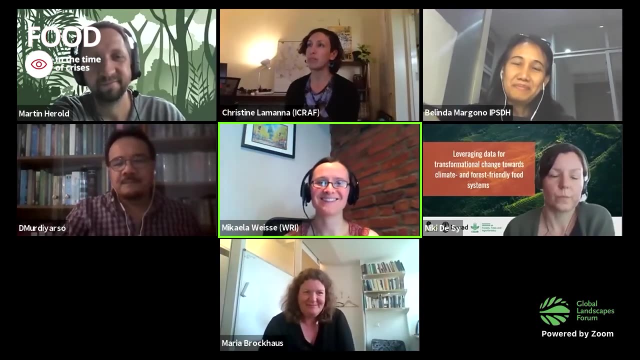 then I can just transition into the co-produced information. I really see Global Forest Watch as an interesting place, because we're generally not actually producing the information ourselves. We're. we're taking information from academic providers And certainly there's a choice about which data sets we think merits adding to the platform that we spend our time on. 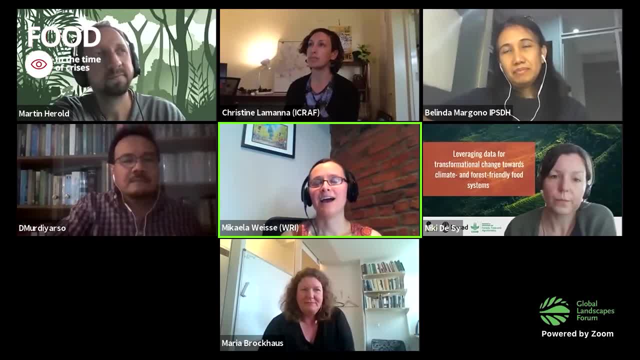 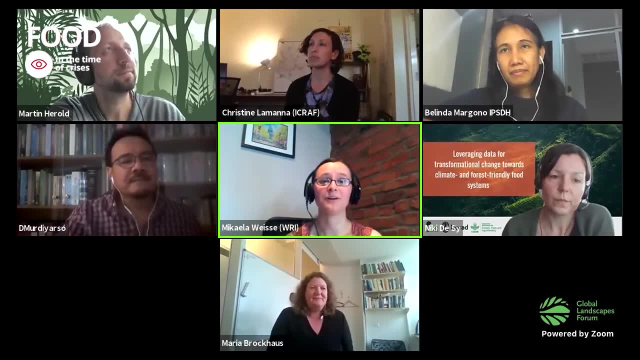 But I think a big part of our role also is in just advising users and trying to be as transparent as we can about what are the limitations of the data, where it works well and where it doesn't work as well, And also on what are appropriate uses and 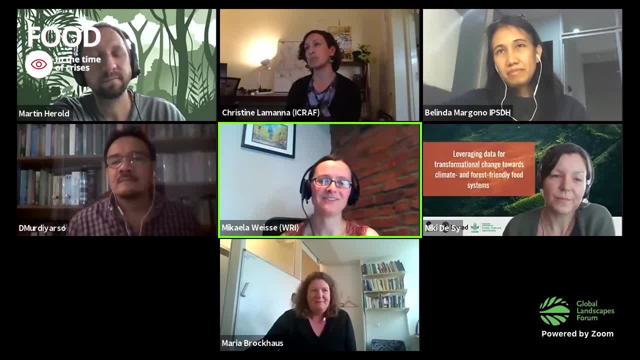 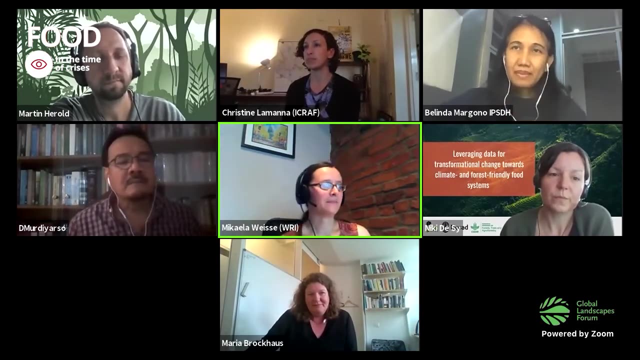 what are also not appropriate uses of that information, And so I think we are trying to think about that constantly and trying to be responsible and aware that certainly this people are using this information and that has consequences in the real world as far as the co-produced data. 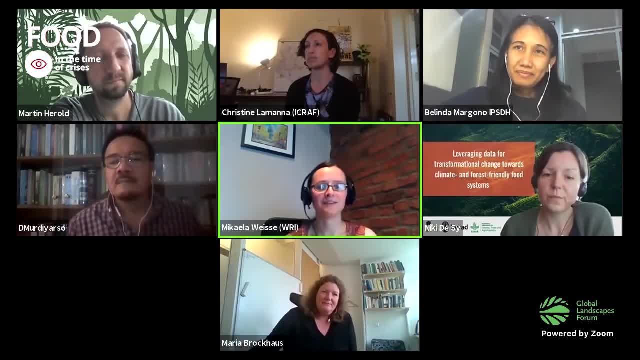 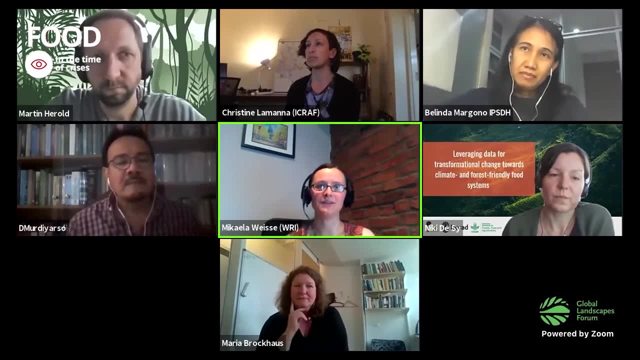 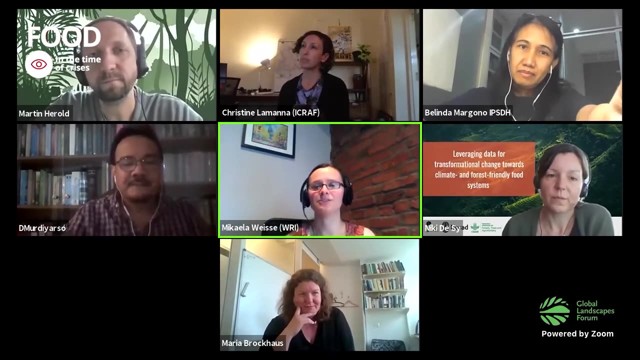 And I'm interested to hear from from Martin and others that have maybe done this more, more directly. because we are a global platform, We constantly have this tension between how do we kind of take these broad global data sets but then also make them applicable at the local level and make 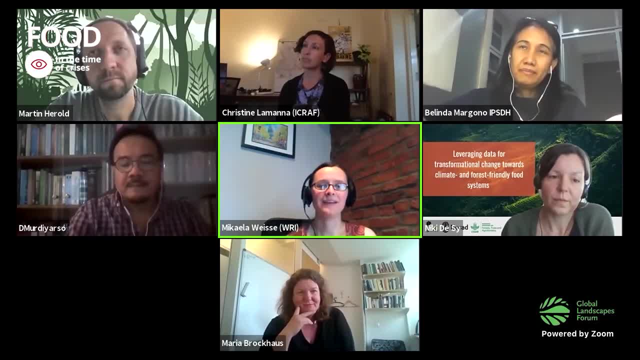 sure that we're taking local perspectives into account. So I would say it's something we struggle with. We don't have an answer. What we try and do more and more now, I think, is really providing this information in a way that it is more possible to integrate. 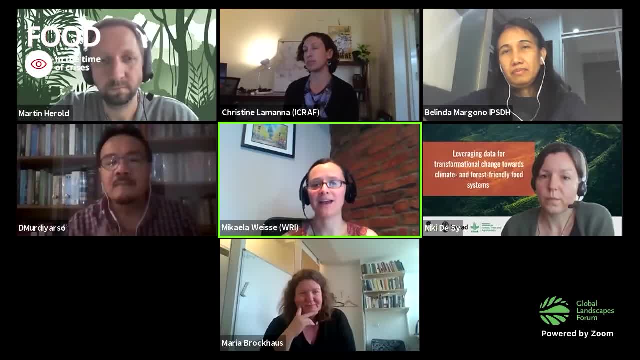 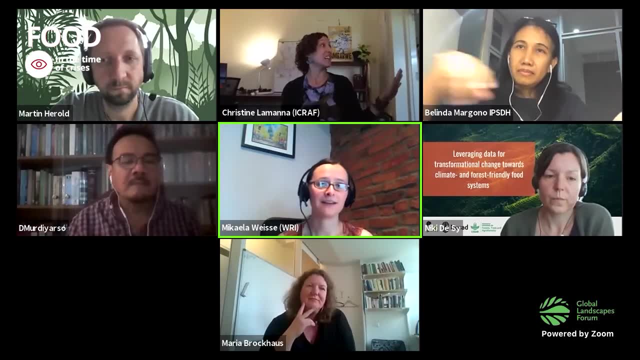 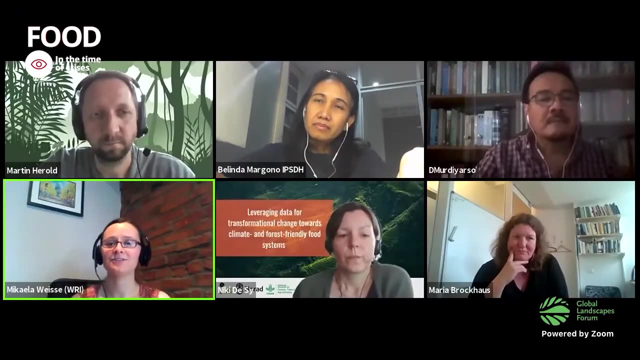 with systems and data collection mechanisms that are already happening at more local levels. So I think in the video from Marco with Cernanp, we are providing new real time alerts from the University of Maryland to them, but also making it very possible and easy to integrate into tools like smart. 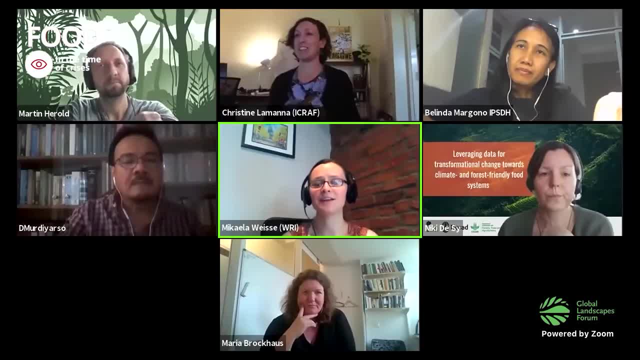 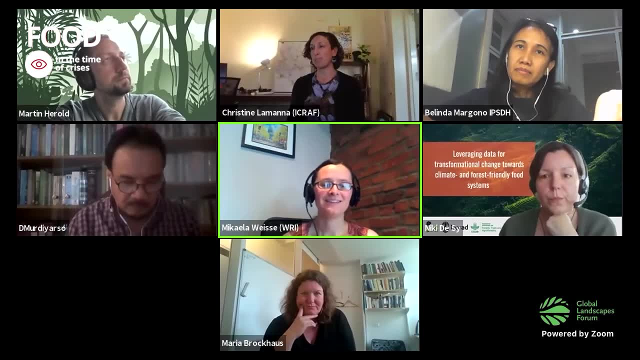 which they are already using for data collection, so that this can just be another input and also be used along the side all of the other information that they collect, Because we definitely know that this kind of satellite based information is not going to solve all the problems. 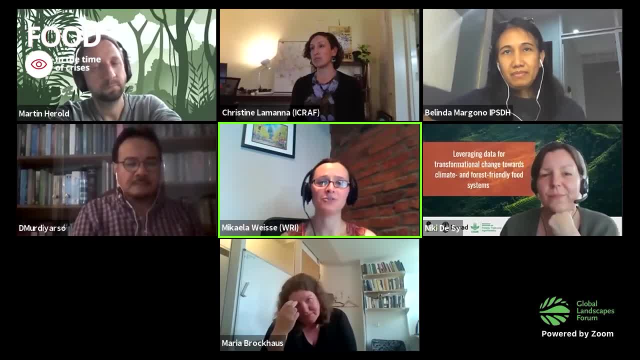 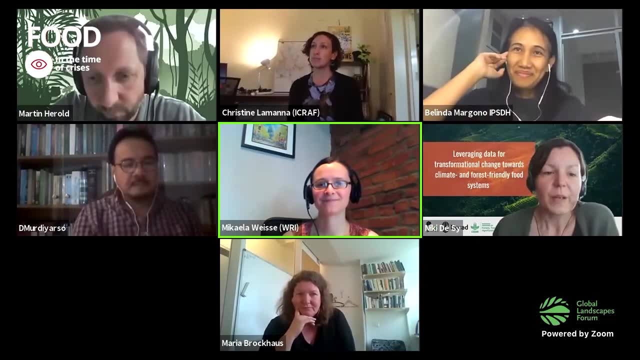 Right there. There needs to be a lot of other inputs of information and local knowledge and expertize if you're actually going to have effective use of that data. So you want to do, you want to direct on that as well, Martin, or? 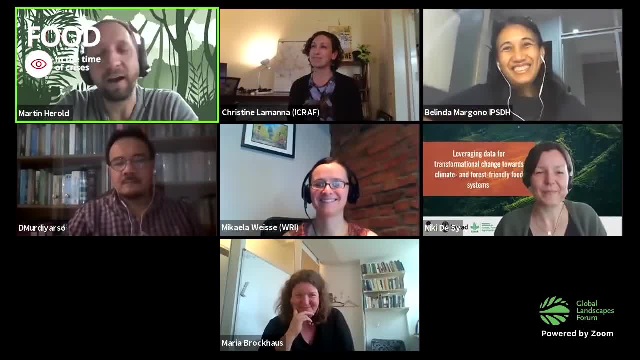 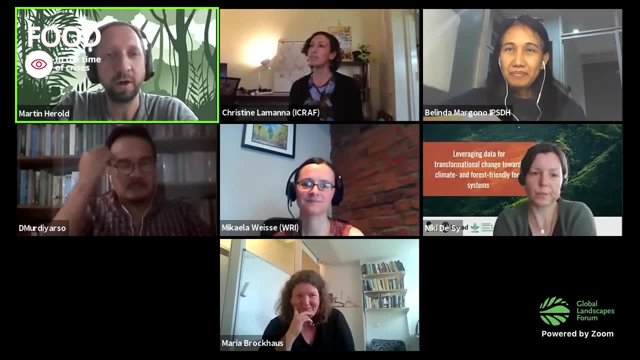 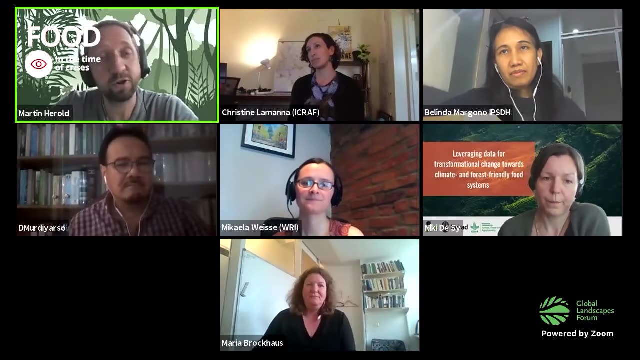 I was just about to raise my hand and on this I mean, I think this, these, these take an advantage of both. this kind of what you call community or locally acquired data doesn't have to be communities, can also be local experts or citizens, but also, you know, extension workers and stuff like that. 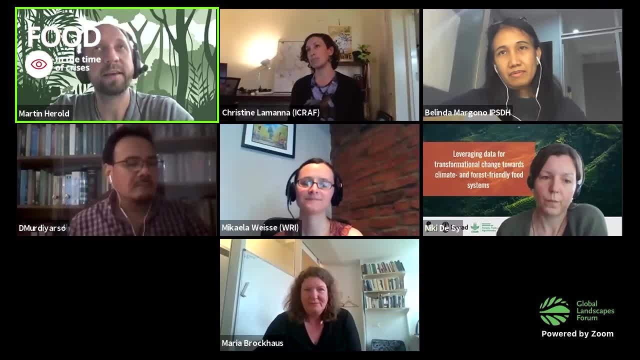 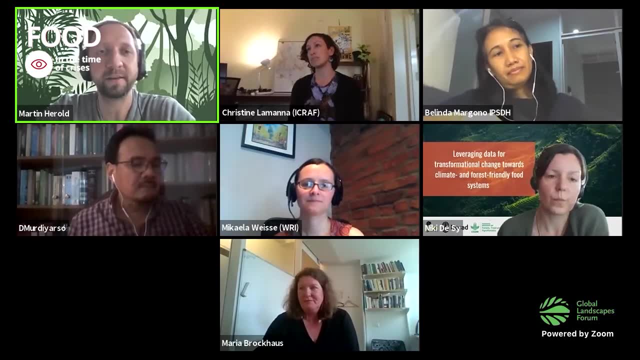 I mean these locally generated data and and linking that with the global and try to do it in a more interactive way. from a technology side, That's quite possible now And that's not really the limiting factor. I think it's finding the ways how this can work in practice. 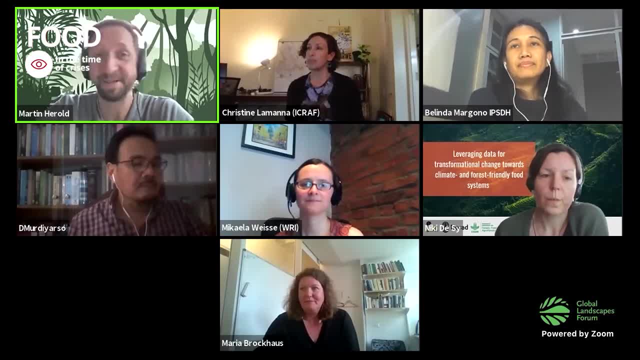 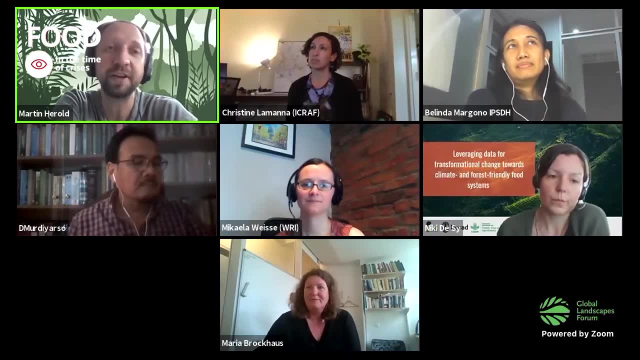 It's linked to a governance system, maybe a decision system, maybe an incentive system and stuff like that. I think that is where part of this challenge lies. So there's there's a lot of good research on that. I think there's not a lot of very. 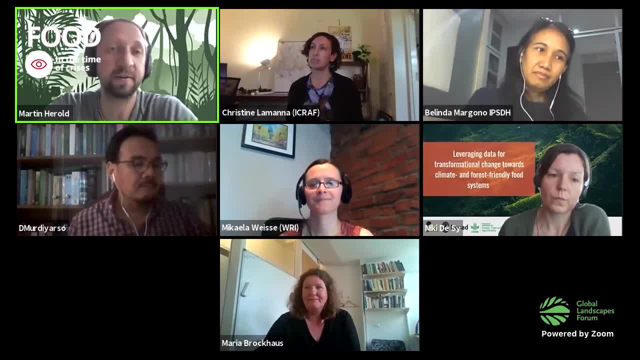 very operational examples in these country contexts, in the context we have been talking about now. so that is, that is part of the challenge, And as long as we don't, we're not able to bridge basically Data streams or information and stuff across these. 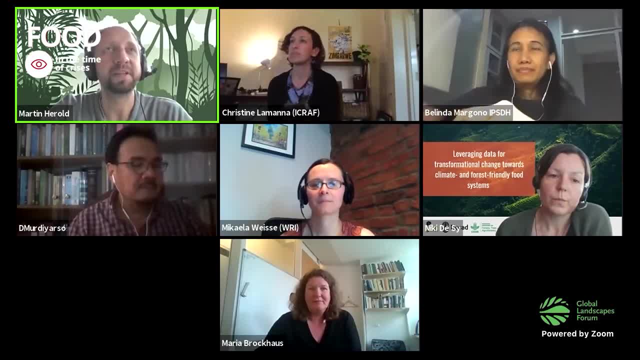 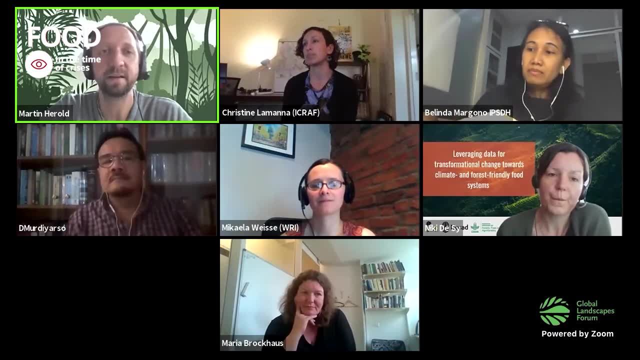 Some of these boundaries, we see we still are a bit stuck and we still run even more into the problems that Maria was talking about. that the data is, limiting It is. it can be biased by generated by a few people, not being a public open. 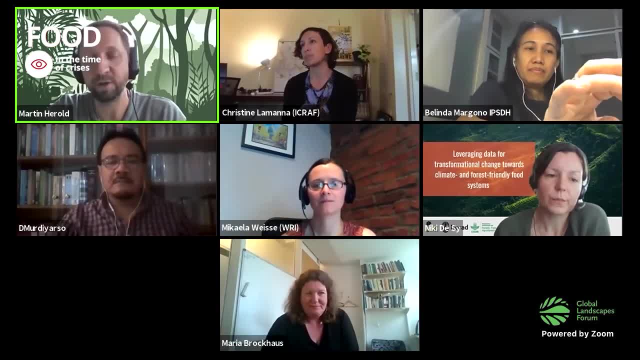 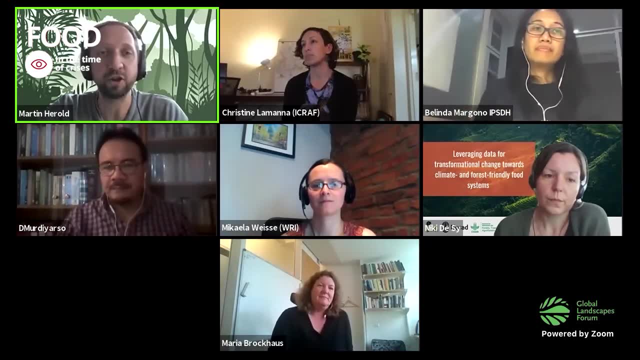 easily understood and accessible, good, as we would like it to have, as we actually need it to deal with these, let's say, sustainable land use challenges, which involve a lot of people, a lot of stakeholders, And ideally, we want everybody to have the same level of information. 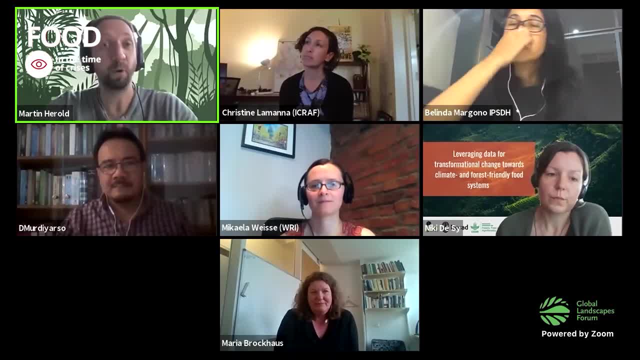 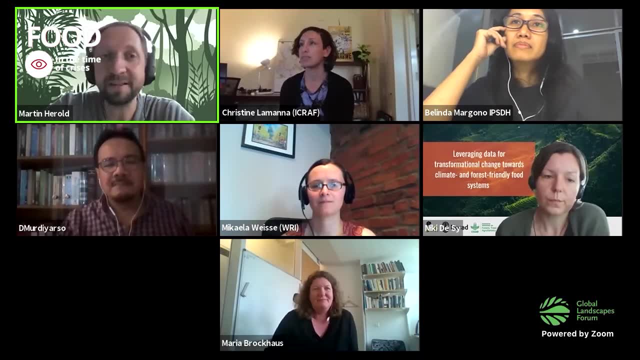 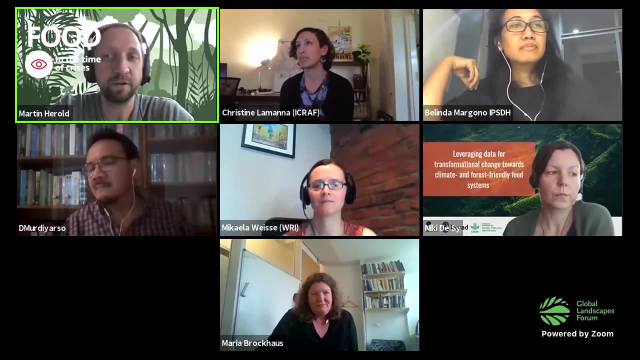 and the same understanding to tackle a problem that we all agree is a problem together. I think we've came a long way in general with transparency and transparency frameworks and more open sharing and stuff like that. I think that is a very important development. I think there is a lot of political push now in the direction which is: 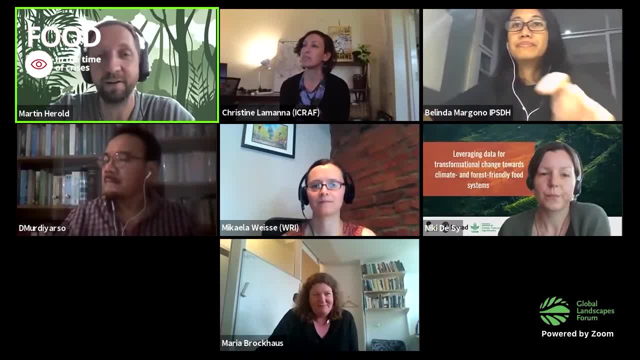 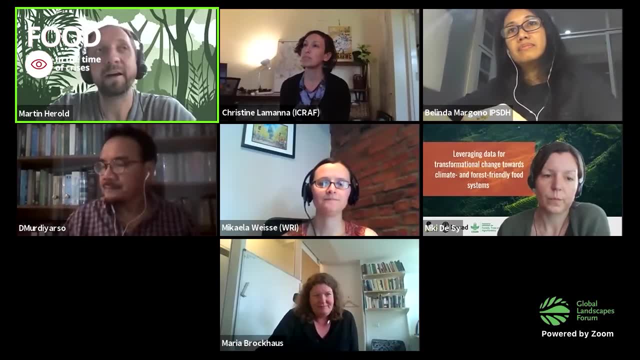 I would say almost unique to that climate change kind of sector. I think not a lot of other sector. I think it's also really, really in this transparency world active at the moment. But still, I think this question on asking where the data come from who's 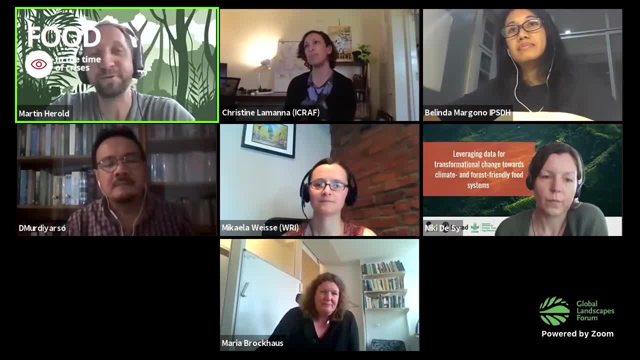 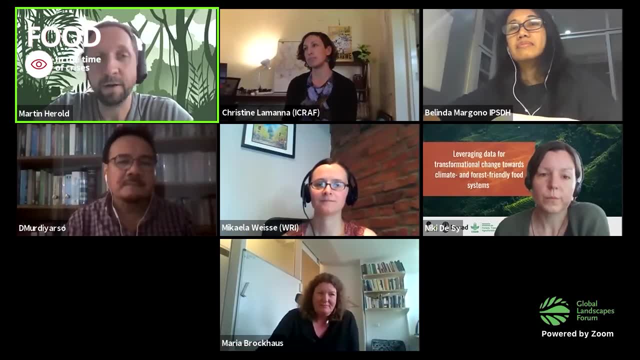 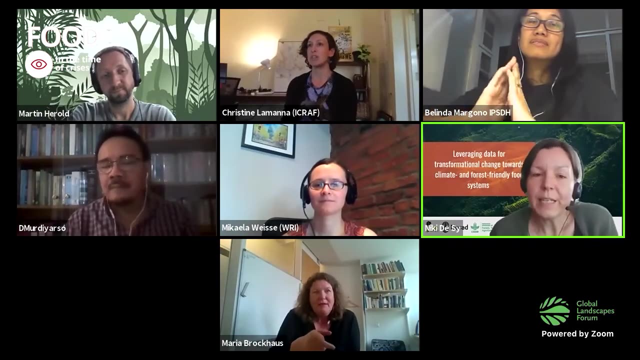 generated them for what purpose, and who's using that information, for what interest, and so on. that that is a good question that we should always ask ourselves. So that's why also the input from Maria was very appreciated. Yes, indeed. So I want to move also. I think Belinda wants to react as well. 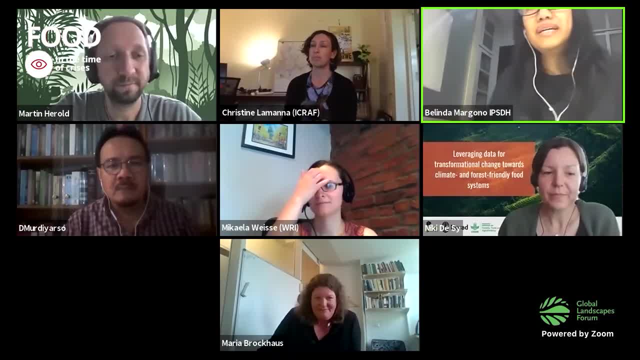 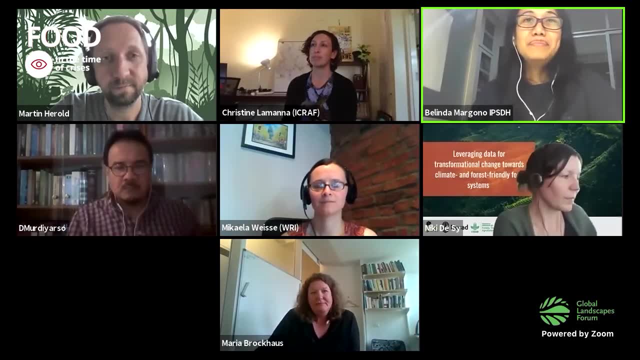 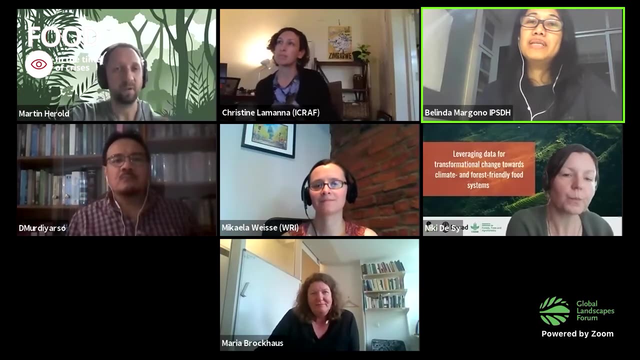 So go ahead. I probably just would like to add something. I think the data can come from everywhere And I'm happy that Kyla mentioned that sometimes remote sensing is not answering all the questions. That's just really true, because sometimes people think that. 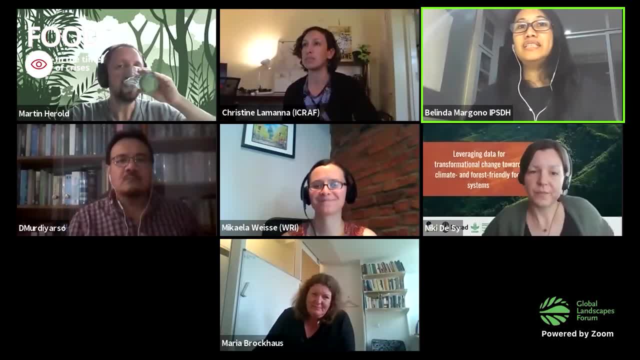 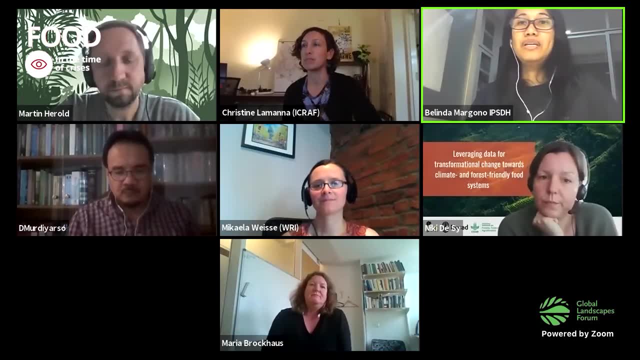 the remote sensing data is a magic that can give all the information we need. It's not like that. There are still a lot of lack of information generated from the remote sensing, So we have to give understanding to people, specifically people for operational 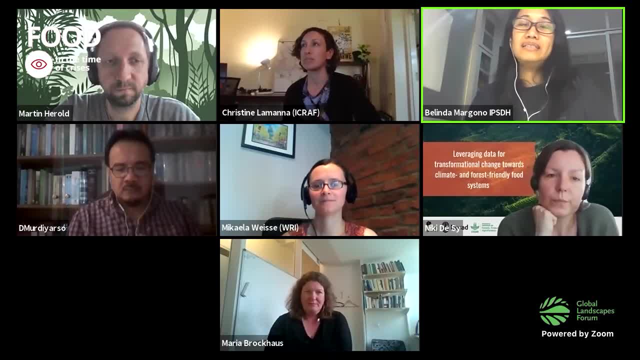 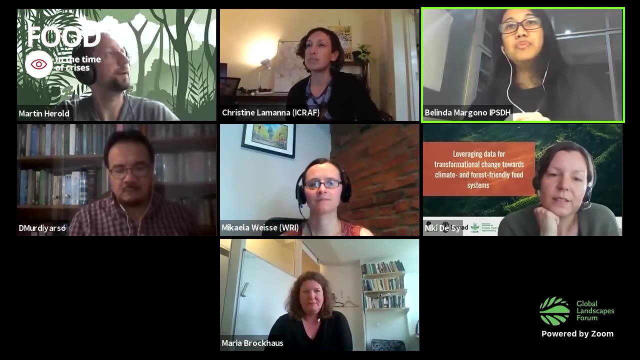 that we need to combine all the data generated from remote sensing with other data source, that actually it's better collected from the ground and it's better It was produced by the people. I probably will not use the word of a community, but could be. 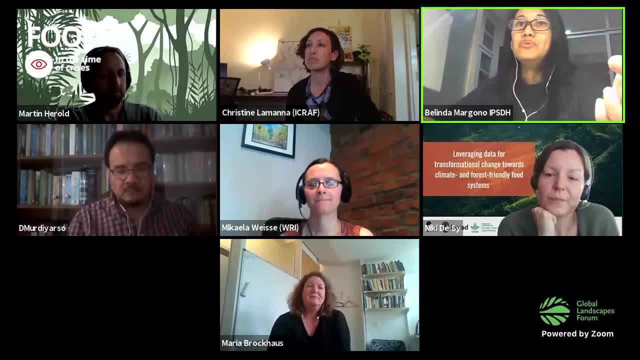 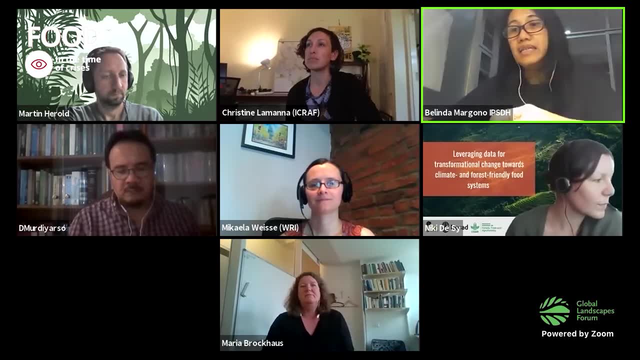 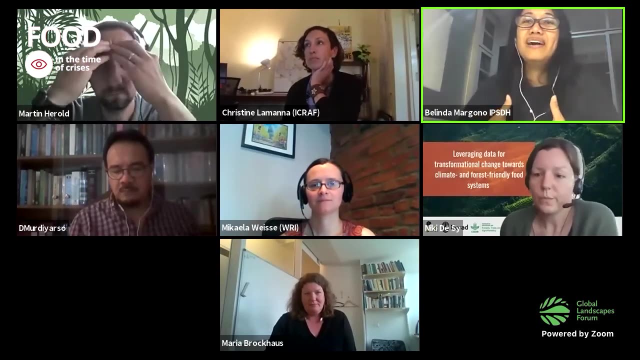 local people could be the country or could be whoever who actually live and know the area very well. Why I mentioned about this one? because I think, regarding the data, the ownership of, or I mean I mean the feeling of have the ownership of the data, of the problem of using the data, that is also very important. 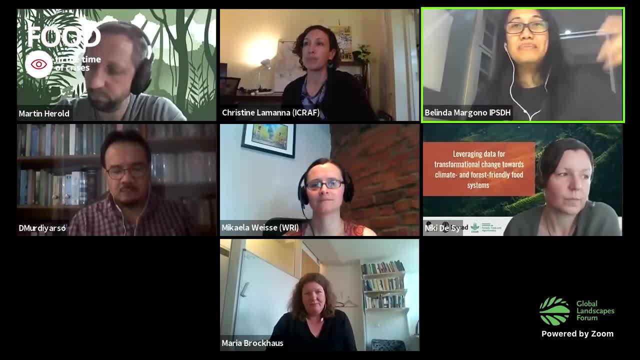 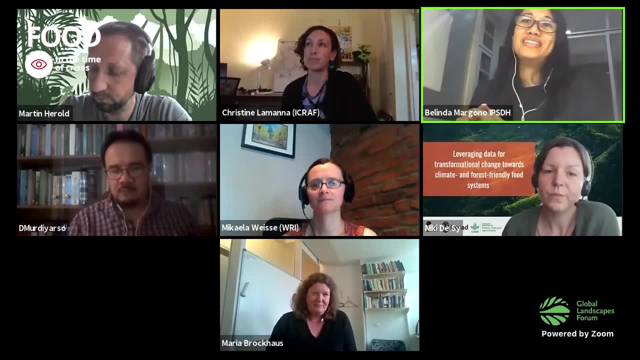 I mean if you use the data and the data is ready from somebody else and you just learn it's different If compared, If you have your own data and you produce the data by yourself. So this is something that actually we need to. 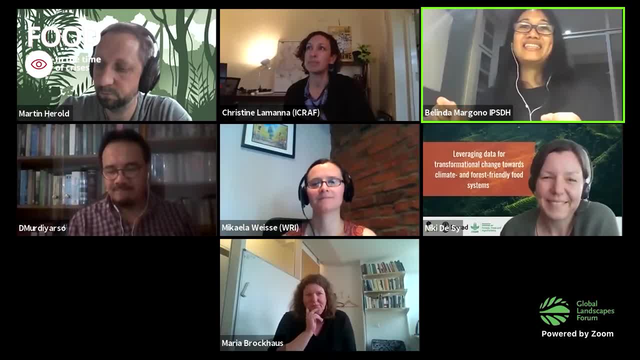 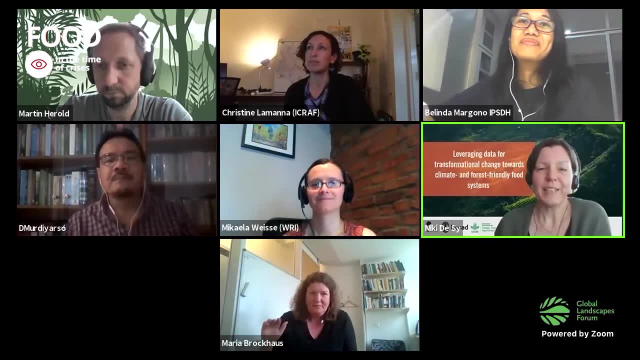 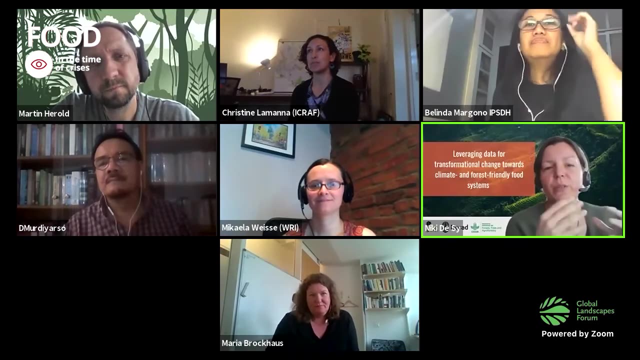 count also regarding this at the position of the data. So that is the point that I need to add. Great, I think that was also exactly the direction I wanted to go in, in the sense that also, indeed, we can do a lot with remote sensing, with field work. 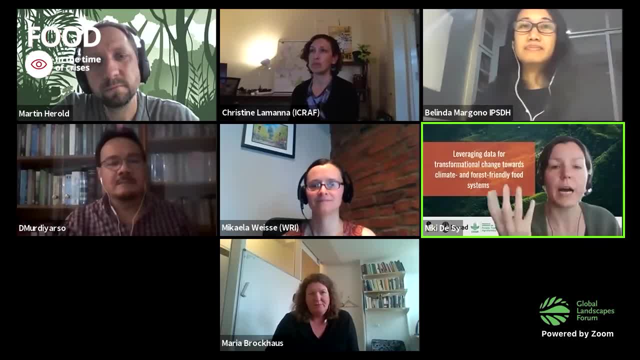 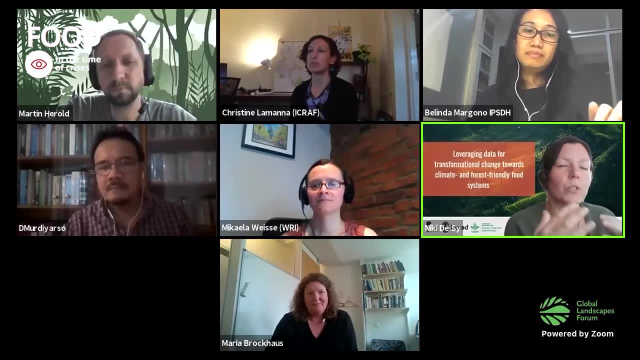 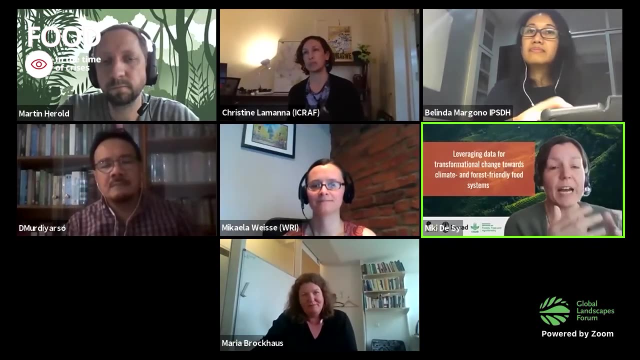 But you know, I feel sometimes that there's a certain type of data is often still missing, more related to socioeconomic biodiversity and maybe going a bit more towards not. OK, the forest is changing, But why is it changing? And I would almost argue that the more information you get also coming. 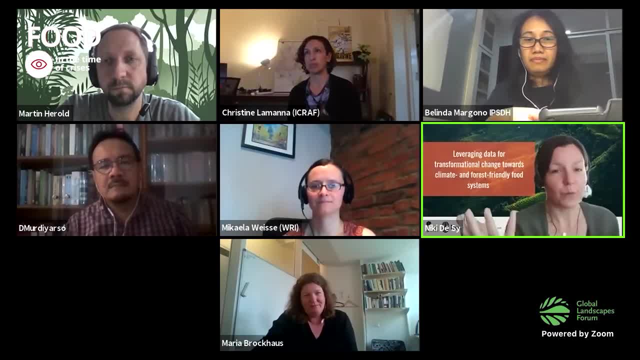 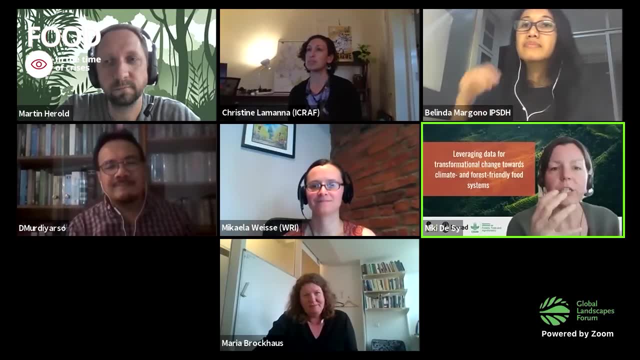 from different sources that feel ownership over the data, I guess the more friction we're going to get as well, Right, I mean so. so I want to ask people as well what their opinion is about essential data that we're still missing. I also got a question from the audience and that said: you know if you have? 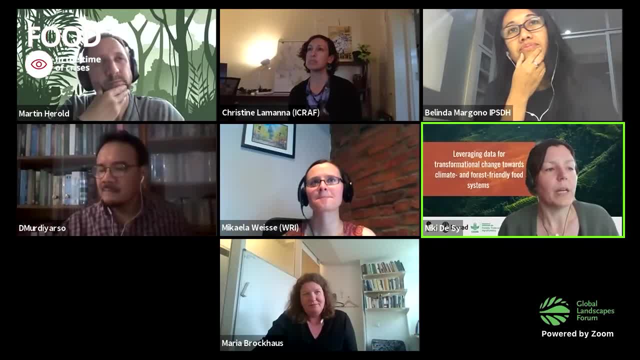 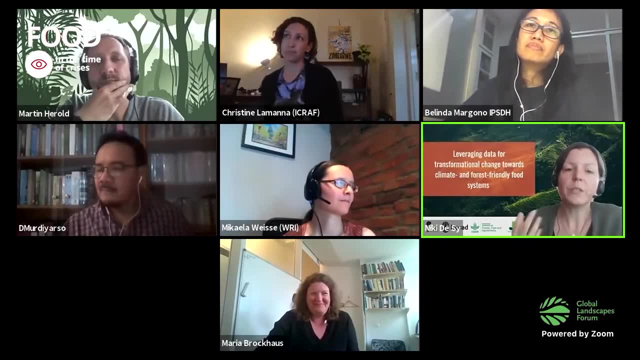 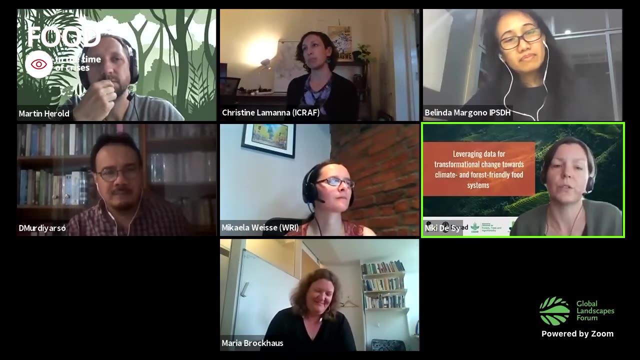 you know which essential data should be presented by every serious reforestation or agroforestry project, or I would even keep it a bit broader, sort of sort of what is essential data? and especially, which, which components are we still missing? What are we not focusing on at the moment that we should focus on? 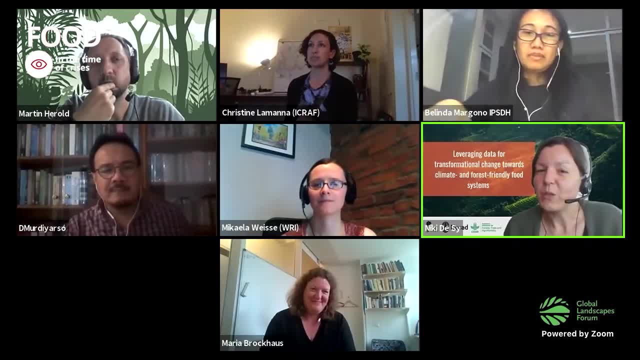 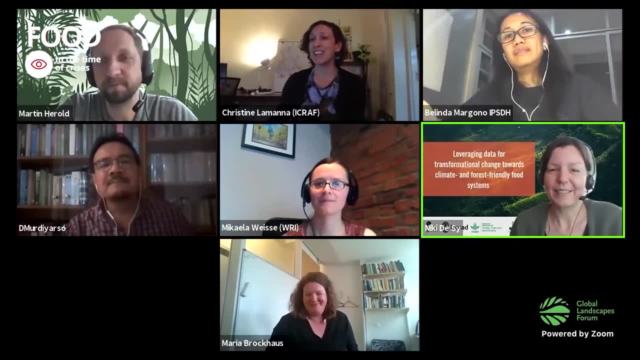 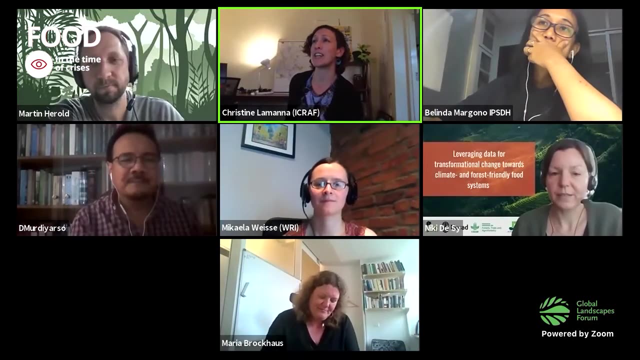 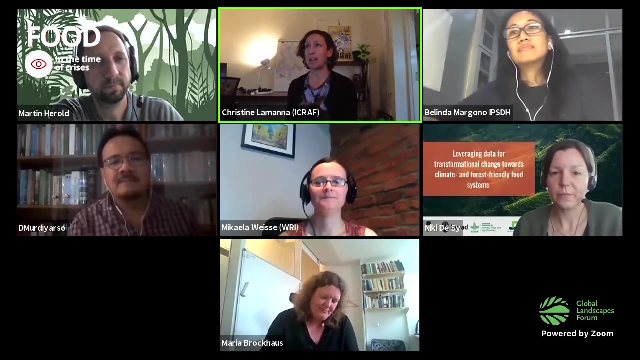 So I'm not sure if who wants to start with that. Christine, go ahead, Sure. So I can kind of reiterate a bit of what Veronica was saying before she got cut off. her connection is bad and she sends her apologies, But she was saying that for climate change planning here in Kenya. 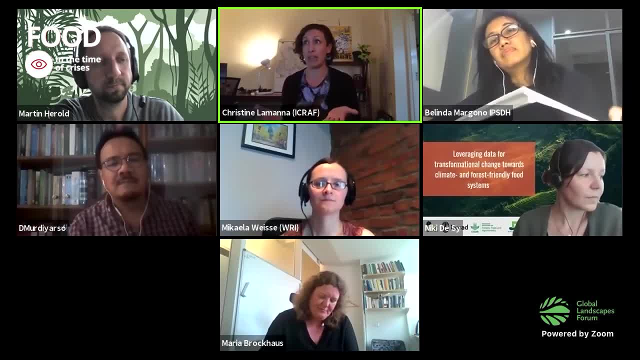 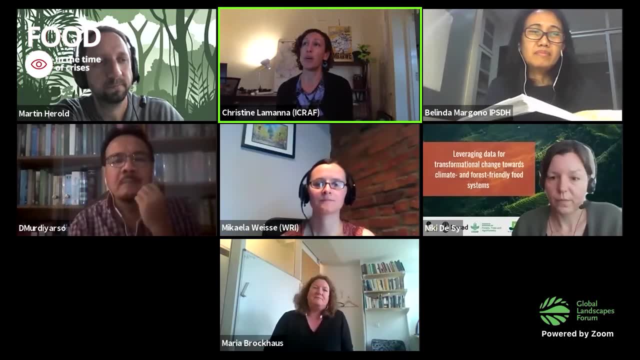 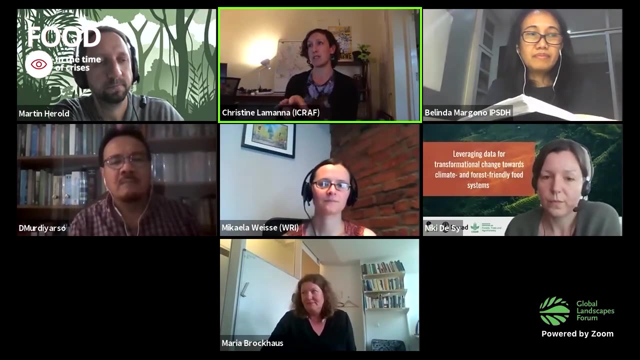 one of the key things that we need is information about what's going to happen in the future, which which here is actually really challenging, And so one of the- you know, I think there's really two key data needs, And one is sort of that, that kind of downscale climate information and even 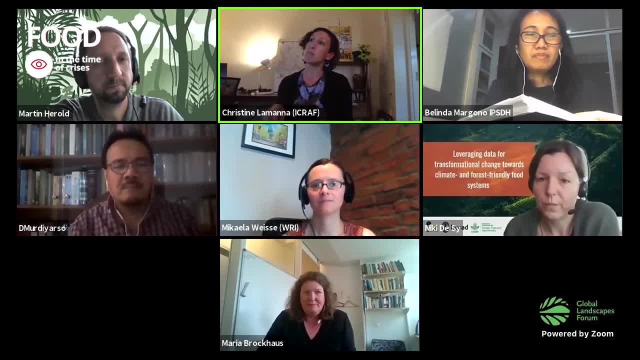 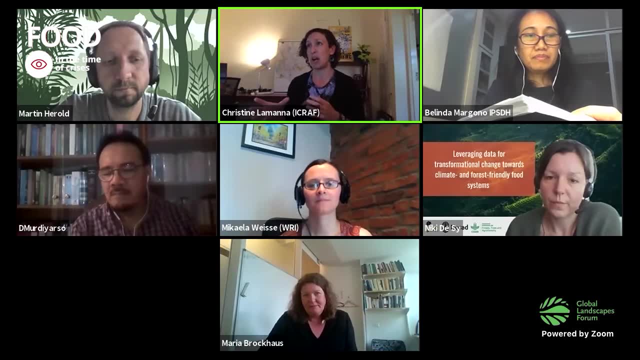 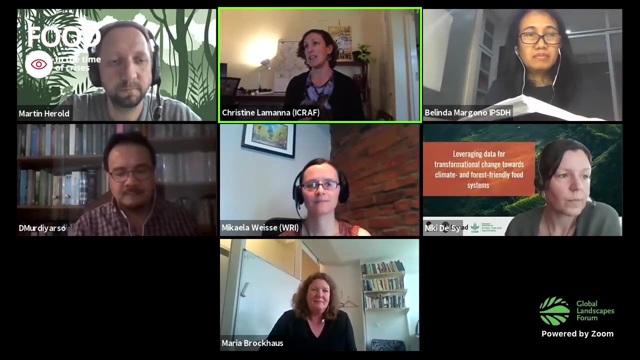 weather information here, where often sort of the publicly available weather information is very, very sparse, whereas a lot of information is sitting in sort of private enterprise hands, And so making that data accessible and open is a really key, key thing that we need to do. 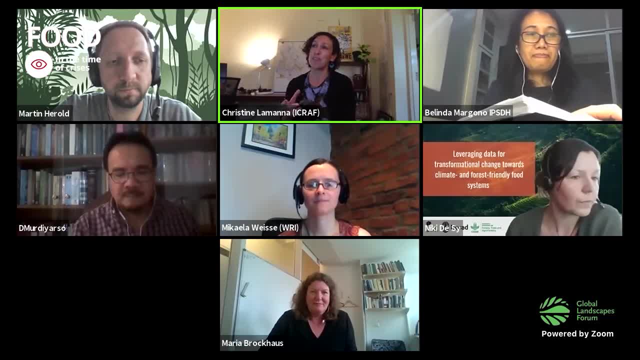 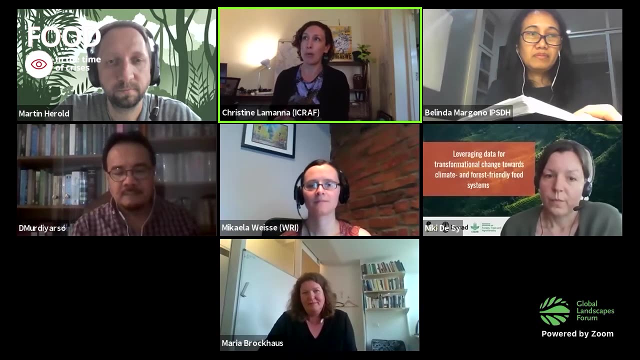 And the other is is is finding these adaptation options, which gets a bit to what Maria was saying about. the politics of this is also: you know, how do we prioritize and amplify sort of the research or the innovations that are done by local people? 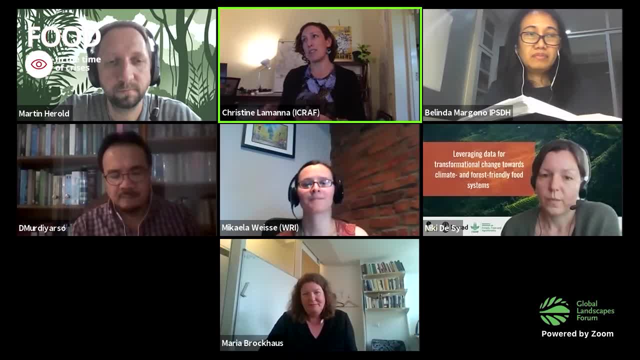 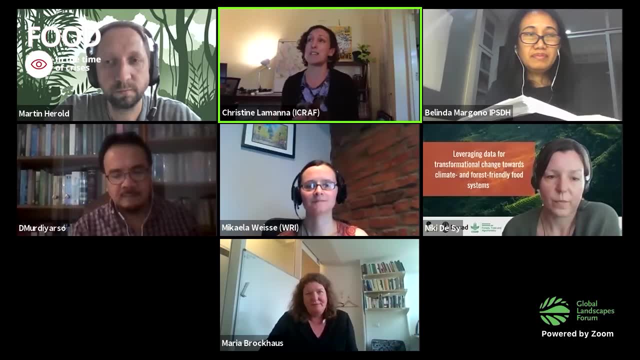 get that information into these decision making processes. So so, both sort of the. so what's going to happen? The climate information is key, especially in our context here in East Africa, But then also, you know, making sure that that in indigenous voices and locally relevant technologies get a spotlight on them as 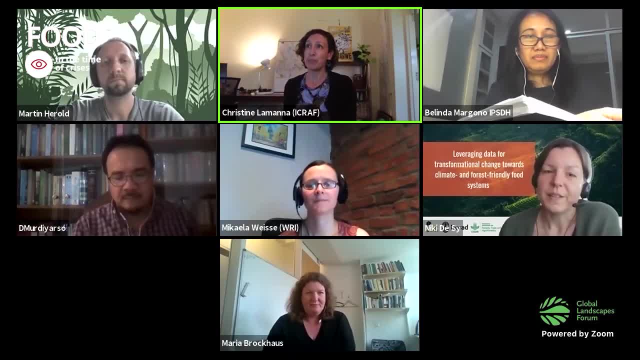 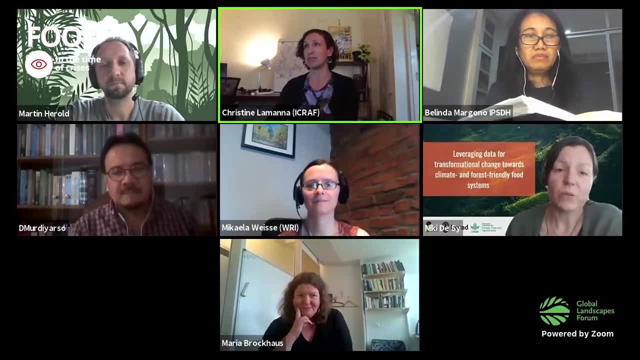 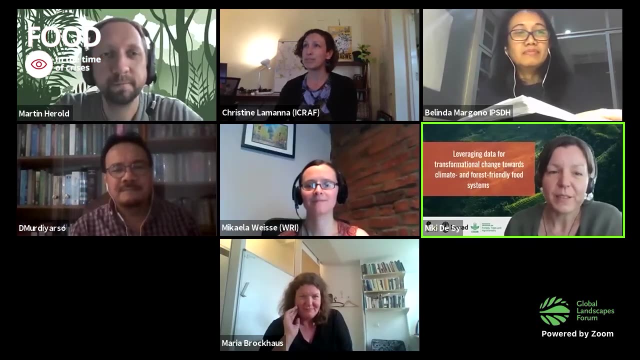 adaptation options. Thank you, Christine. So I'm seeing that we're almost nearing the end of our session, so if I can give the floor to one other person, if they still want to react on this last topic, let's see if I see any raised hands. 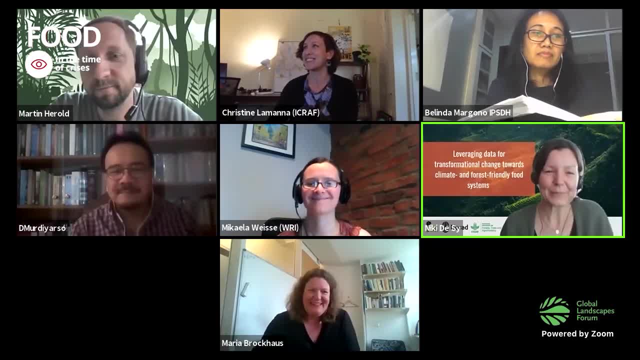 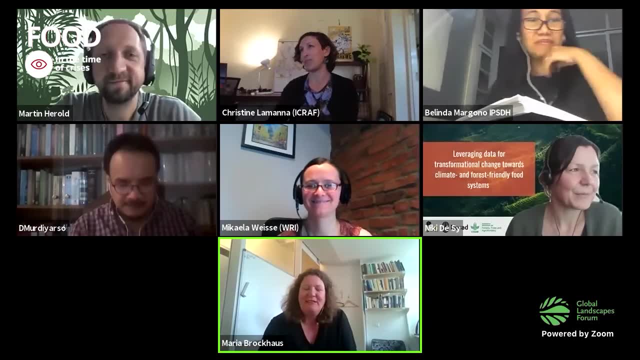 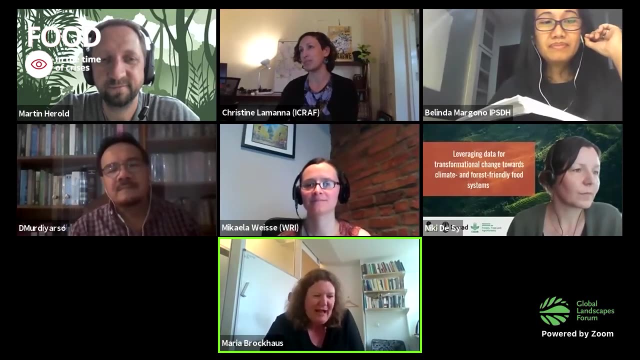 I think Maria wants to say something. Yes, If nobody else wants to say something because I spoke so much, OK, I would like to ask actually the restoration question, because I think it's a great question. and what do we currently perhaps not know, not ask enough? 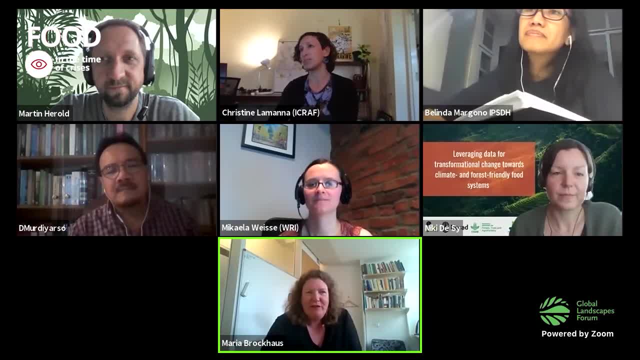 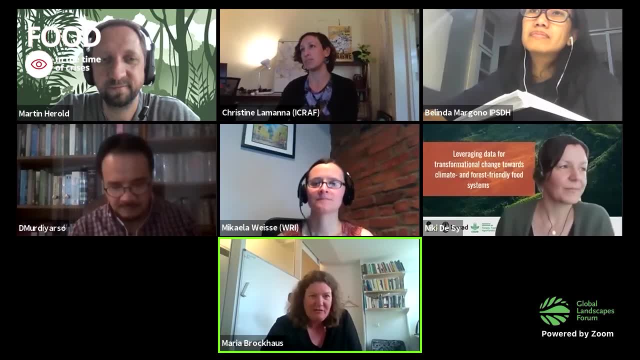 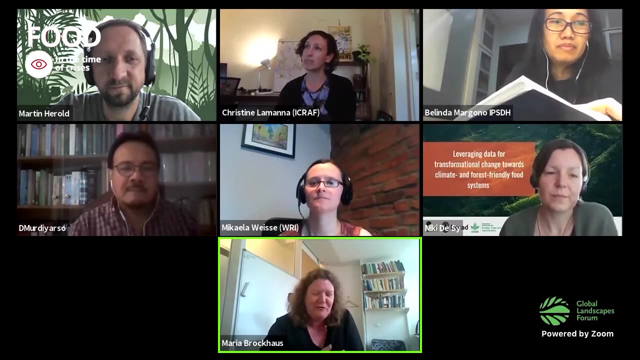 My answer to that would be: actually, who benefits from restoration? So who are those that benefit from large scale restoration across the global South? And that, for me, is a crucial question. We don't even know, which is very interesting Because we know so much about deforestation, on the one hand, 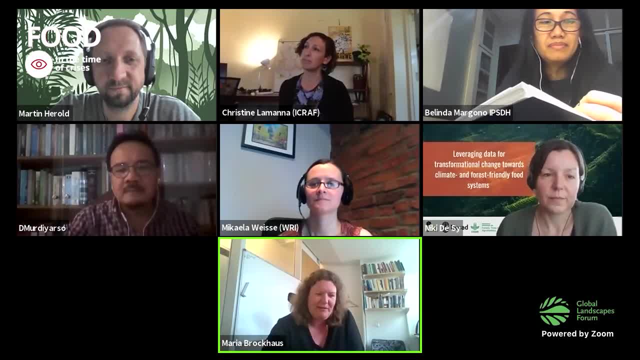 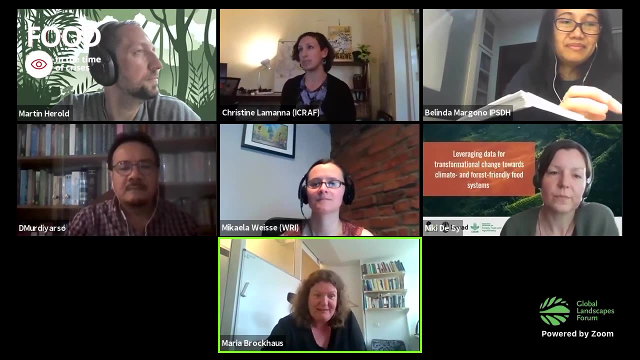 But till today I haven't seen a single paper that really makes the effort to tell us which sector- economic sector- is actually causing most deforestation. This is scarce information And it seems also here we don't ask the questions. Maybe we need to ask more. what species are selected for restoration? 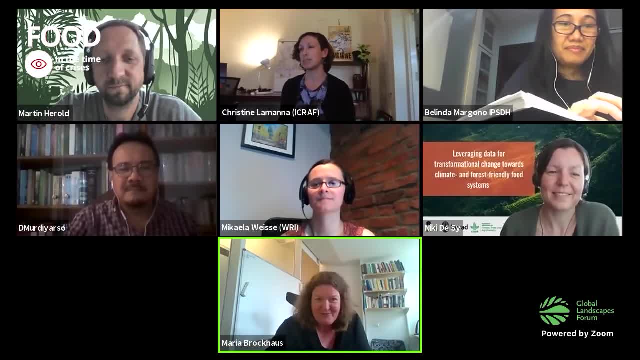 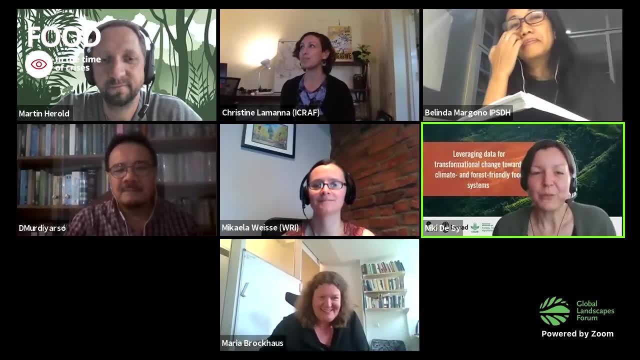 That would be another one leading to the question of who benefits from restoration. Thank you. Thank you, Maria. I'm afraid we're running out of time, so we'll have to wrap up here. I would like to thank all the speakers for being here today.